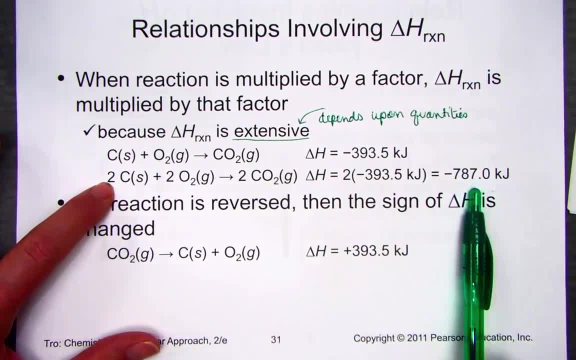 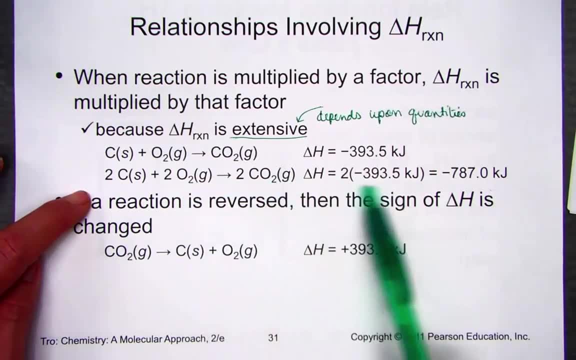 also. then double the delta H Twice. the heat energy is then released. The same is true as if I tripled it. Whatever I did to distribute through coefficients, I do the same to the delta H. If I half it, I take half the delta H. 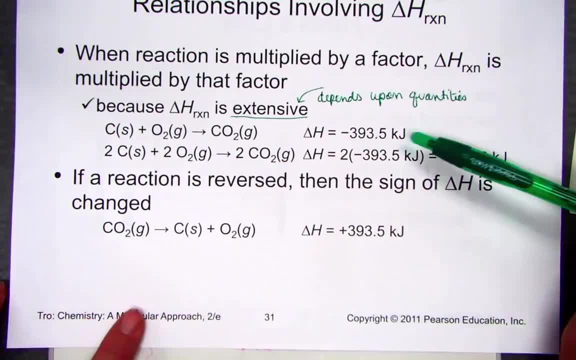 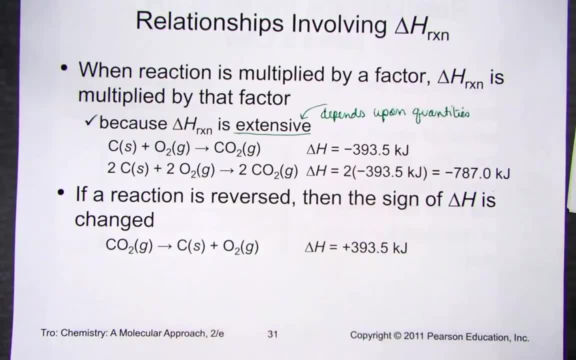 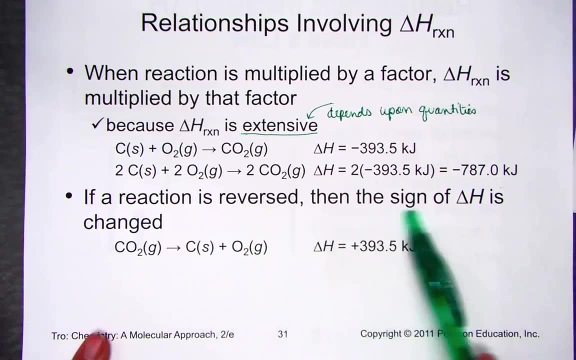 If the reaction is exothermic in one direction, I flip the direction of the equation. The reaction is written in the reverse order. The sign also changes from negative to positive. If the reaction is reversed, the sign of delta H is opposite: Endothermic in one direction. 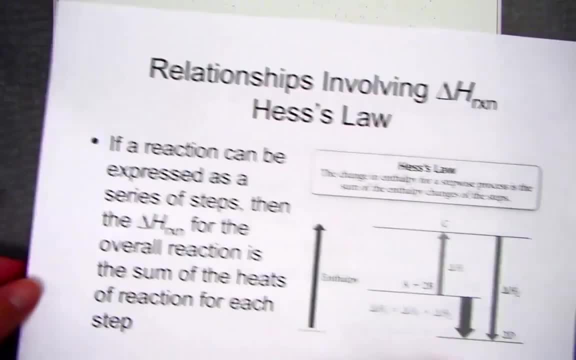 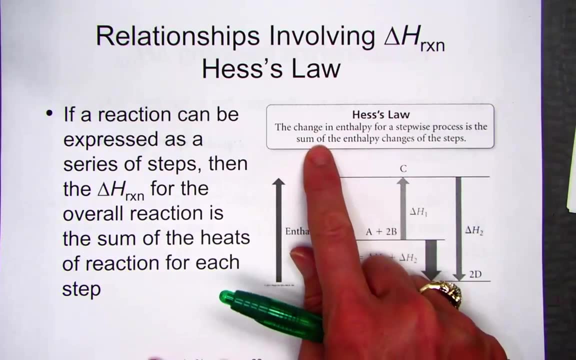 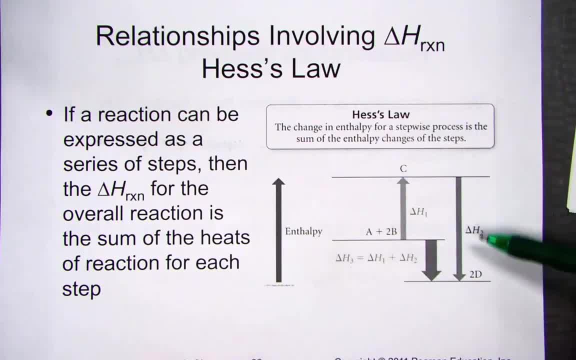 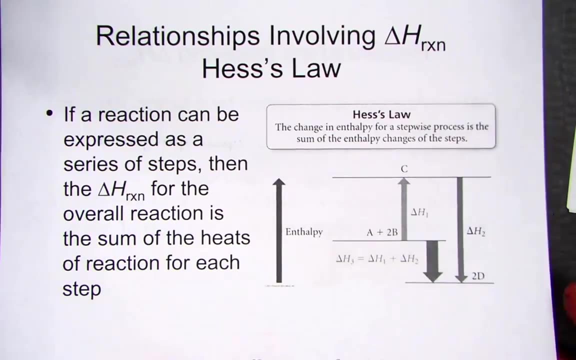 in one direction creates an exothermic in the opposite direction. When added to step one, gives me the complete change. of step number three, The heat of reaction for an overall reaction is the sum of each individual step along the way. If chemical changes occur in a step-by-step fashion, we can simply add those steps together. 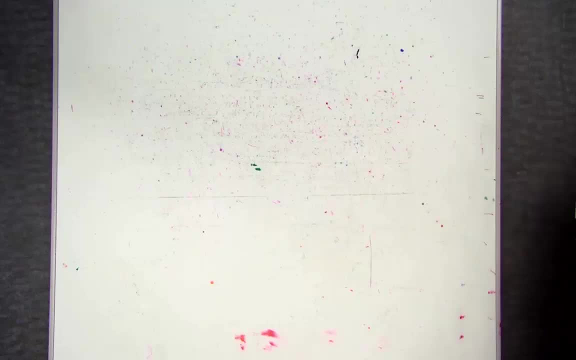 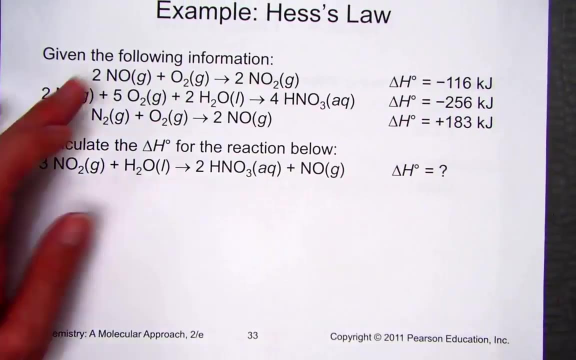 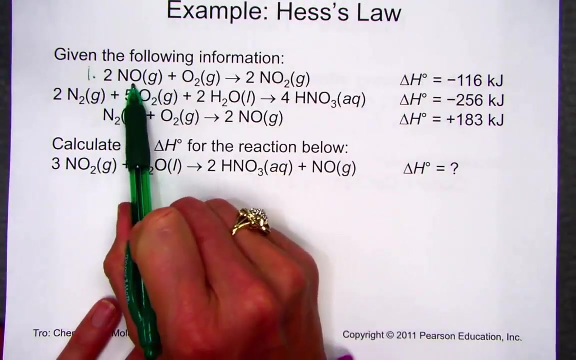 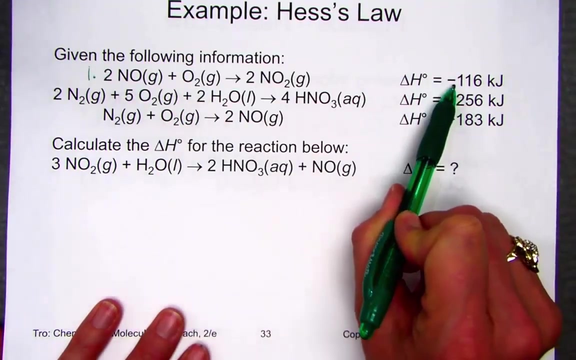 to find the overall equation. Let's model a Hess' Law to see if this helps clarify An example of Hess's law. Let's examine what we called elementary reactions. Elementary reaction: one: two units of NO combined with one unit of oxygen to form two units of NO2.. An exothermic process: 116 kilojoules of heat released. 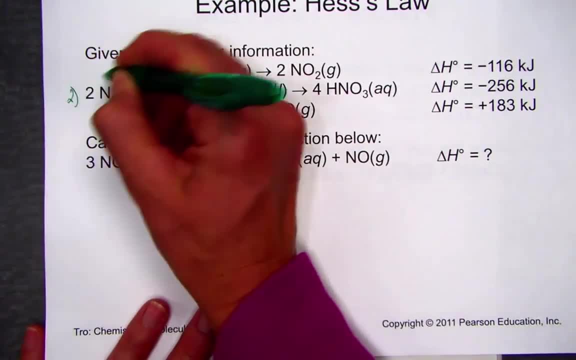 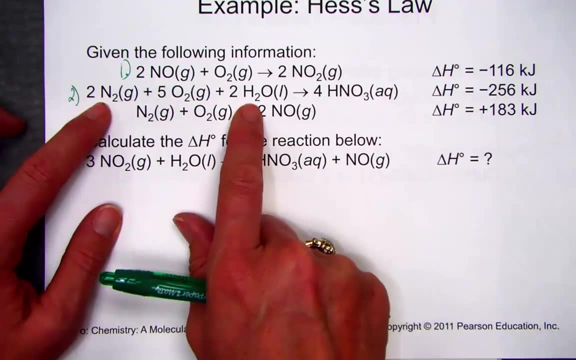 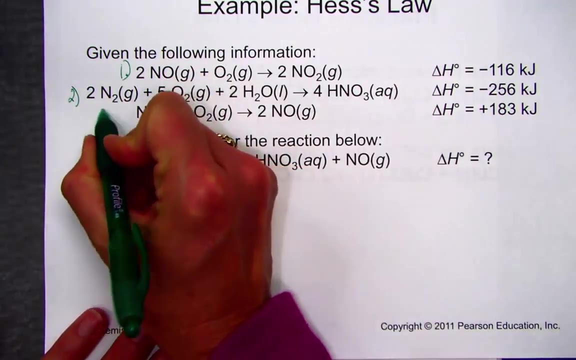 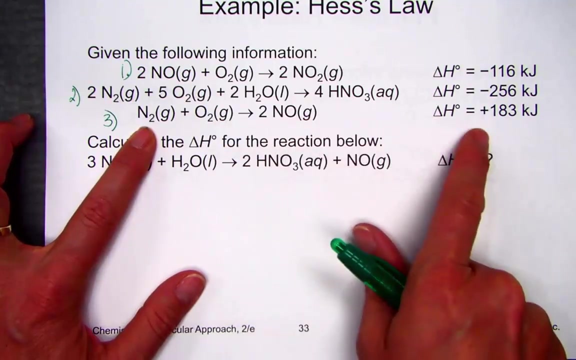 Elementary reaction number two says: two molecules of nitrogen react with five of oxygen and two of water to form four HNO3s, an exothermic value. And there's a third elementary reaction: Nitrogen and oxygen form two NOs. It's an endothermic process. 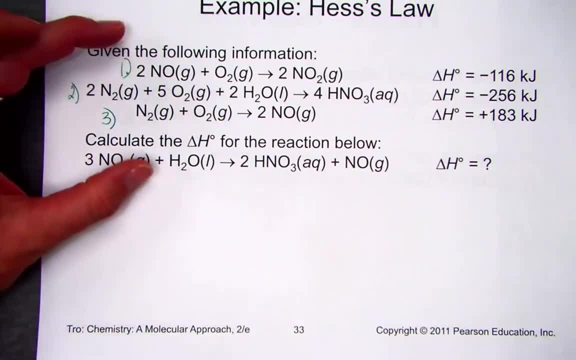 What Hess's law is asking us to do is to combine the two, Combine these three equations so that when it's simplified- just as in algebra- we can simplify things that are on the same or opposite side of the equal. we can do that as well with chemical equations. 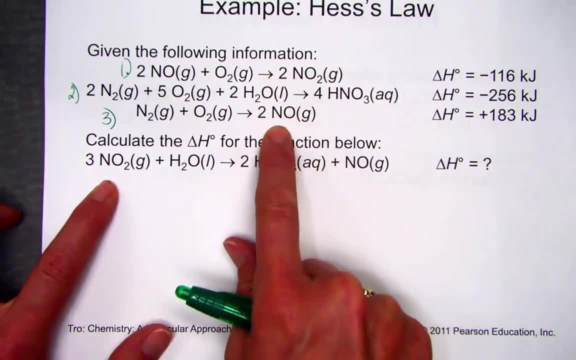 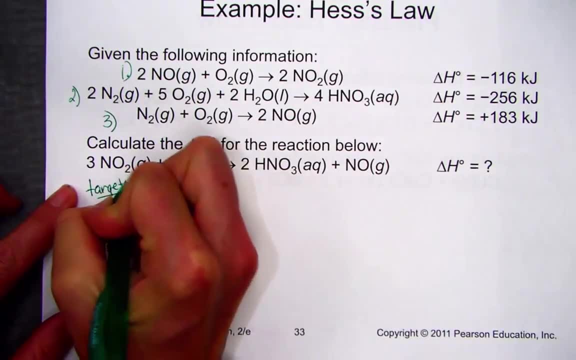 What we'd like to do is to be able to add these three equations so that, when I simplify them, they give us the target, And that's what I refer to as this bottom one. This is our target equation. How do we build three units of NO2?? 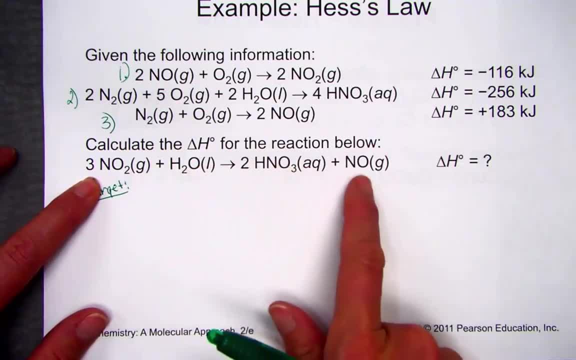 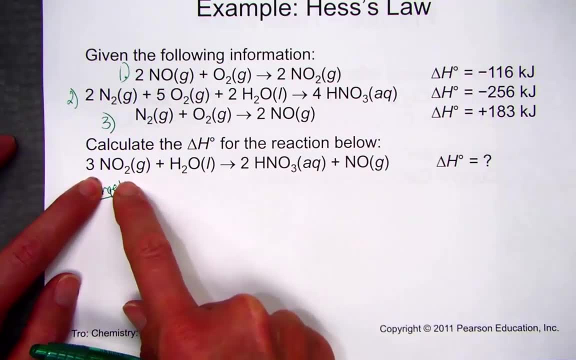 We're going to have two HNO3s plus one water, giving us two HNO3s and one molecule of NO. So I look at the first reactant in my target equation- for no other reason than it's written first, And here's what I notice. I'm going to start going through my equations and see where it's written. 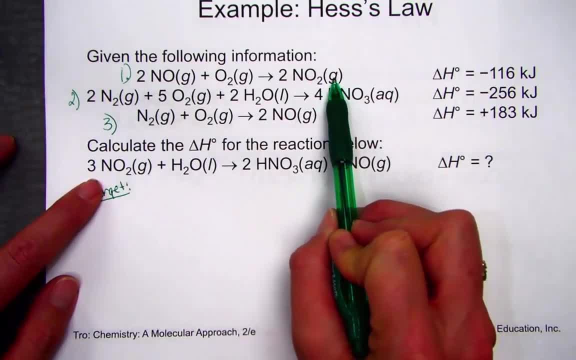 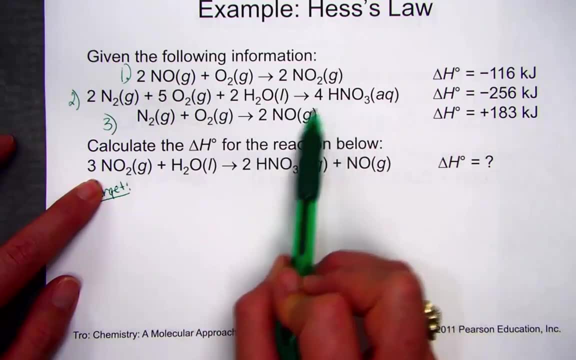 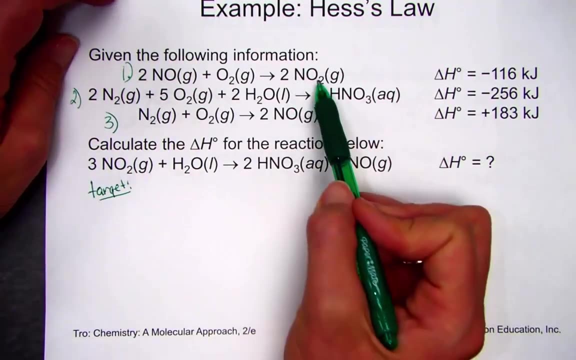 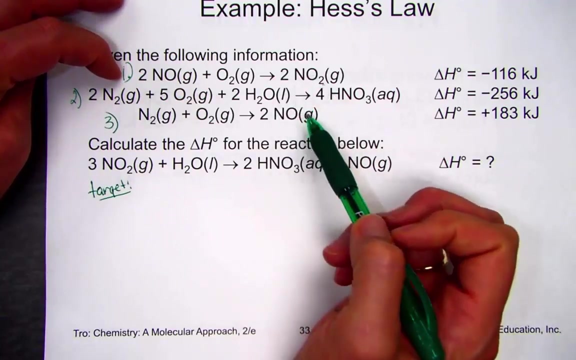 I notice that NO2 is a product in the first equation. Is it written anywhere else or is that the unique place? I don't see NO2 written any other place. So here's what I like about it: NO2, its unique position. So now that gives me some ideas of what we're going to need to do with this particular equation. 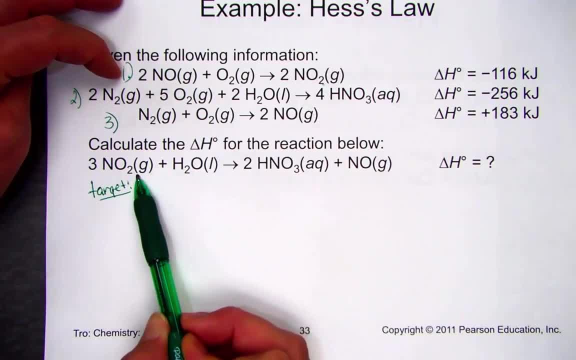 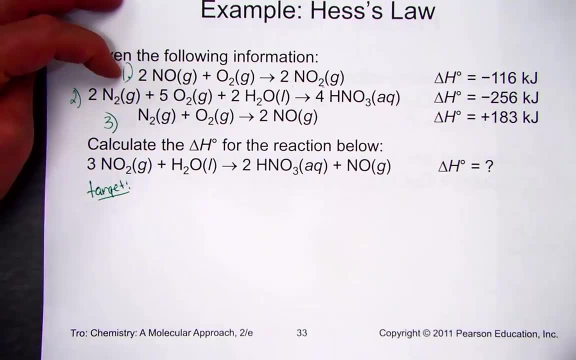 It's on the wrong side of the arrow. It's supposed to be a reactant, but I see that it's a product And instead of two units we're supposed to have three units. Alrighty, What do I multiply two by to get to three? 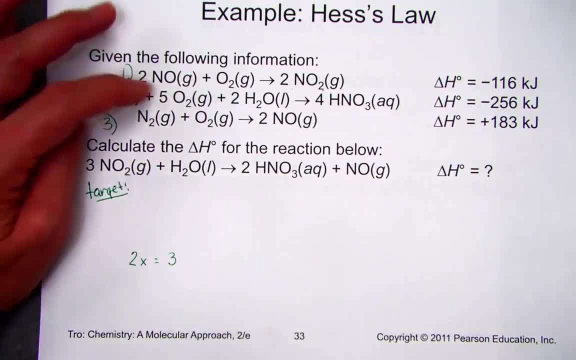 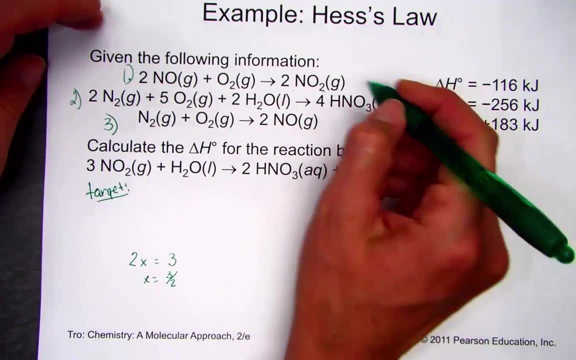 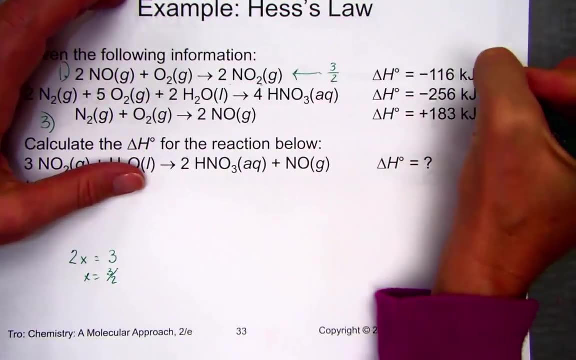 2x equals 3.. So x, of course, is three halves or 1.5.. What I think I need to do is not only flip the direction, but I'm going to have to take three halves to distribute, And so when I do that, think about the delta H. 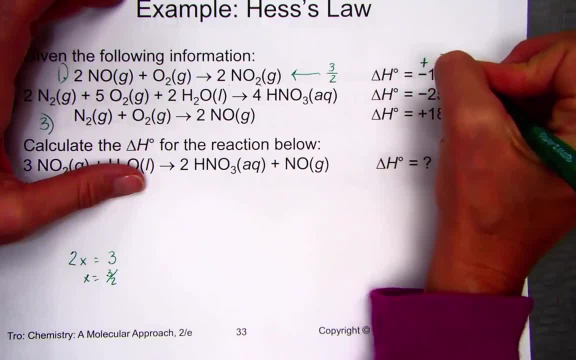 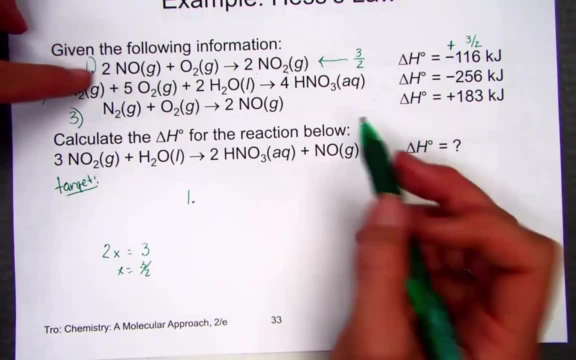 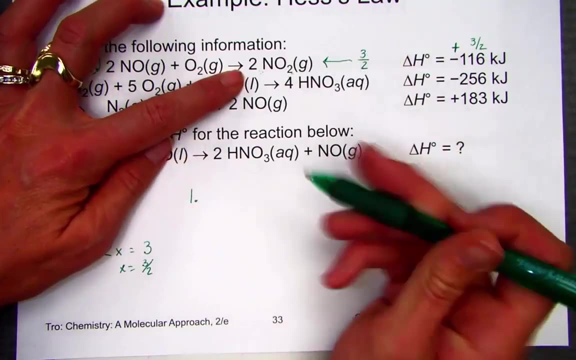 You're going to flip the sign and multiply it by three halves. Let's pause and do that together. We're going to flip the direction, So two units of NO2.. Two times two is six. Six over two is three. So three halves times two gives me the whole number of three units of NO2.. 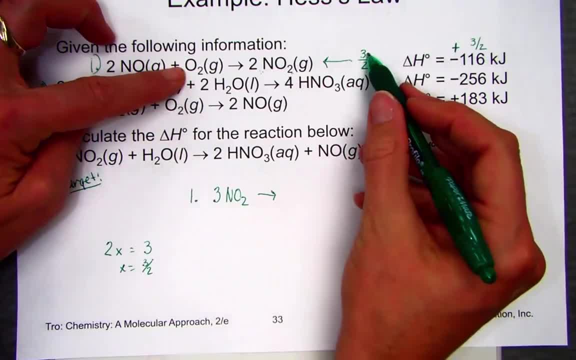 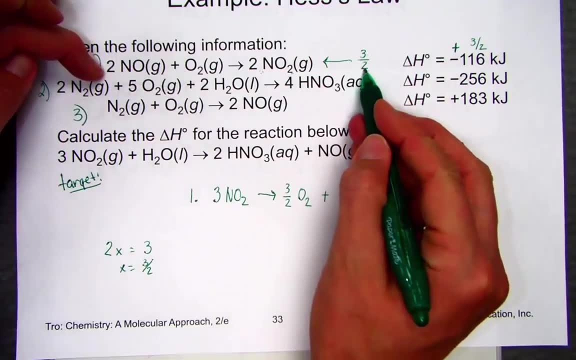 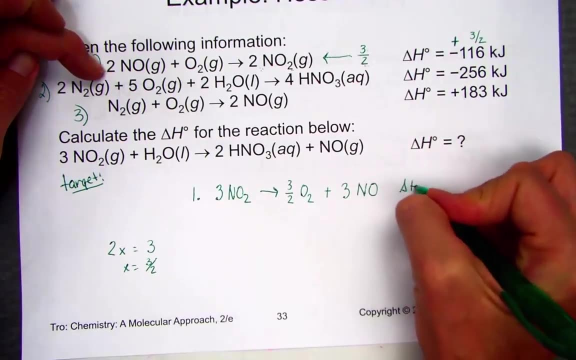 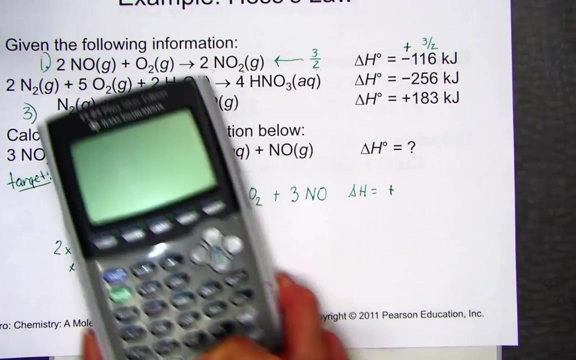 Then the arrow: Three halves times one is three halves oxygen, And three halves times two gives us three units of NO, The delta H. for this equation we flipped the sign because we flipped the direction, And let's just simply hit three halves of 116.. 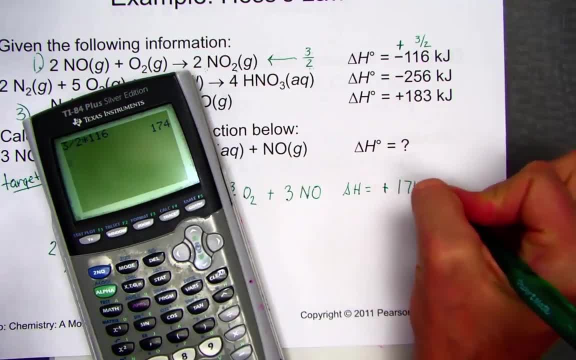 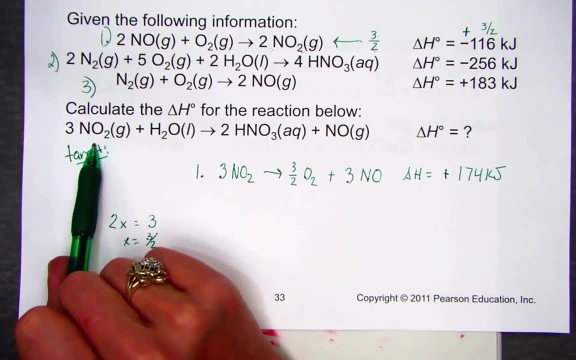 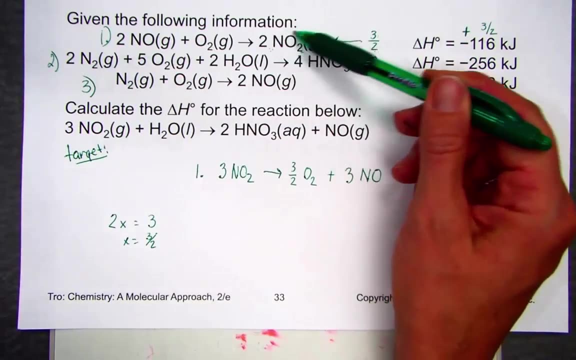 And I get 174 kilojoules of heat. So what I've done so far is just examined the first reactant, NO2.. The unique position in my building equations these elementary reactions was in the first target equation. here The NO2 was written as a product. 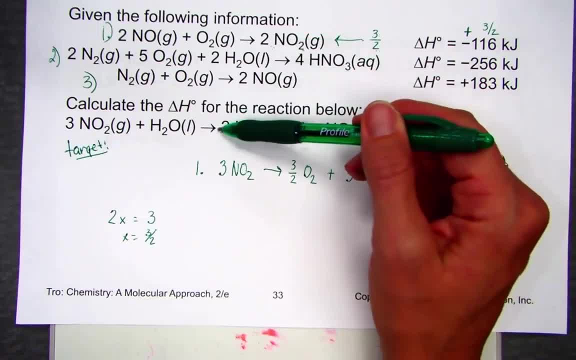 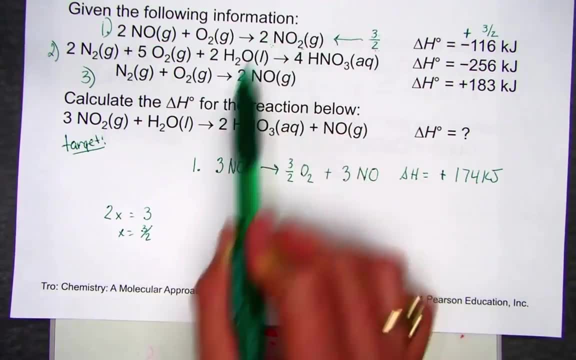 It's on the wrong side of the arrow from my desired location, so I knew to flip the direction. I also had the wrong amount, so I took a fraction. Three halves of two gives me the desired amount found in the target. So I flipped the direction and distributed a three half. 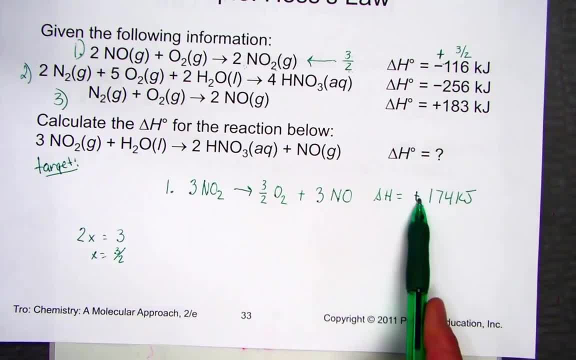 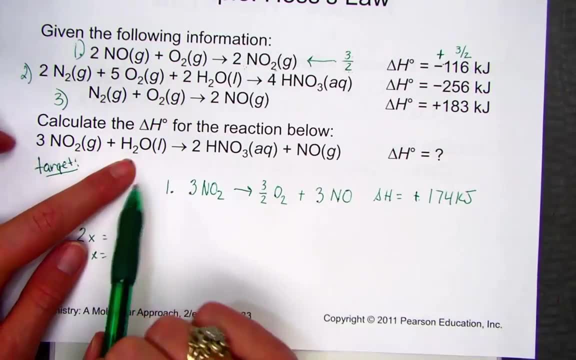 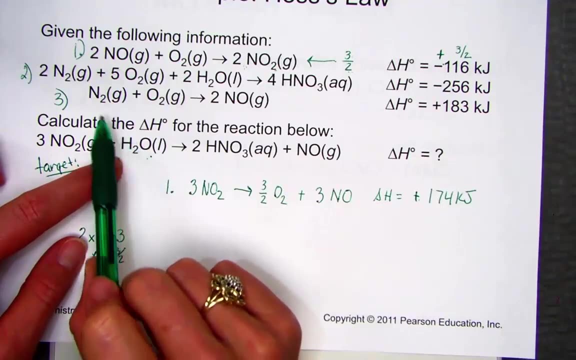 When I flipped the direction, I flipped the sign on delta H and I distributed three halves through the 116.. Let's go on and examine the second reactant in our target equation. The second reactant is water. Let's begin skimming through our building equations to see where we locate water. 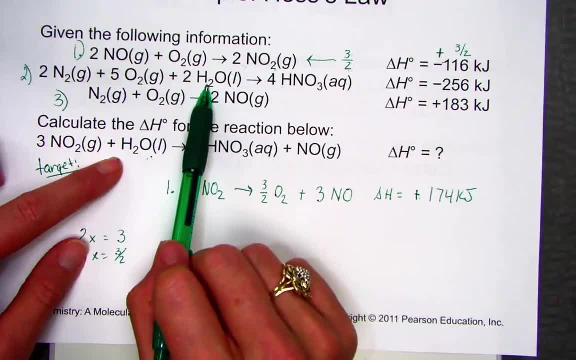 I find it in the second equation And it's the only place I find water. I like the side of the arrow it's on. It's on the left side, as it is in the target, But I have twice the number that I need. 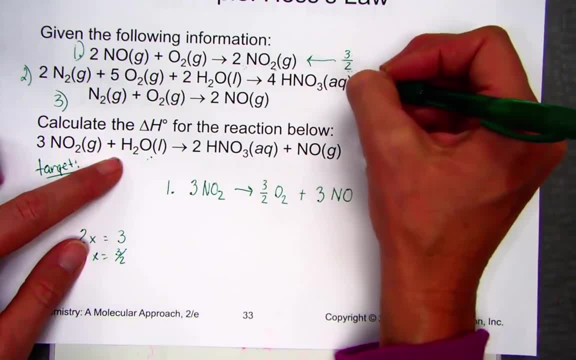 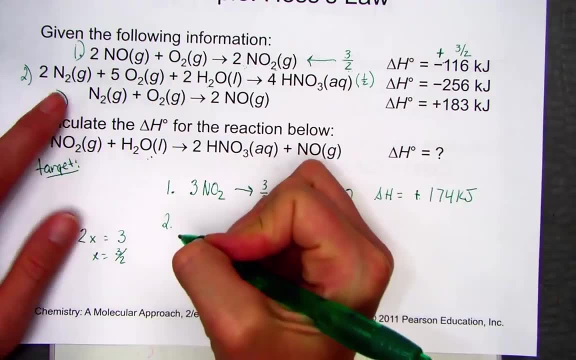 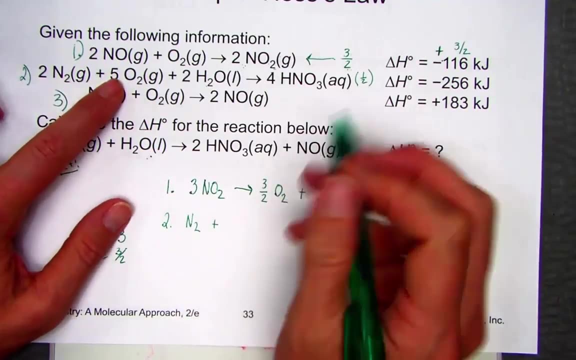 So I'm going to leave the direction alone, but I'm going to distribute one half through that equation. I need half the number, So let's do that together. One half of two is one: One molecule of nitrogen plus one half of five. 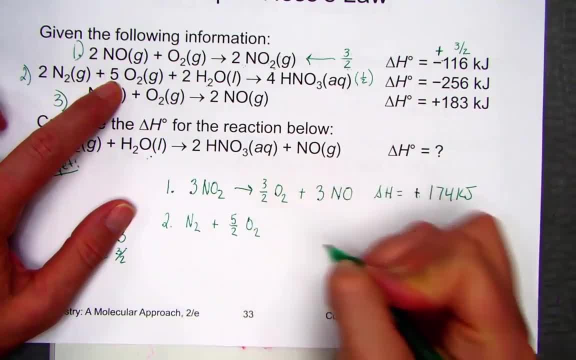 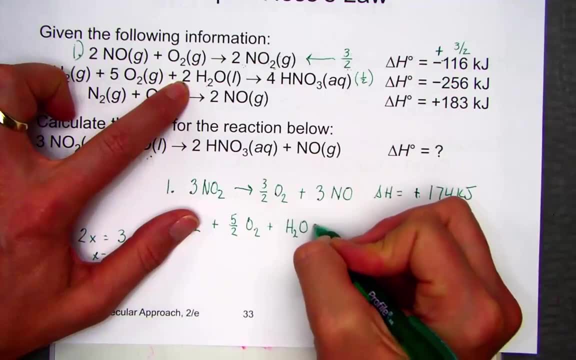 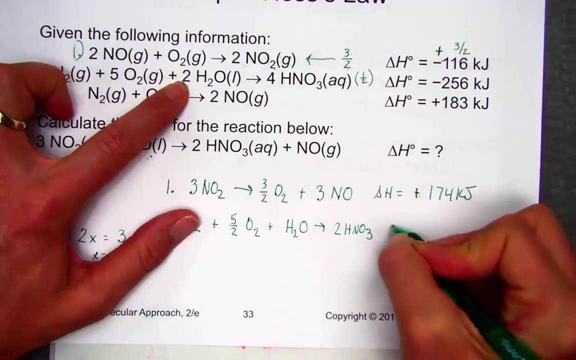 I'll just write it as five halves oxygen Plus One. half of two is a single water: One water And we have an arrow. One half of four is two HNO3s. Let's adjust the delta H Distributing one half. 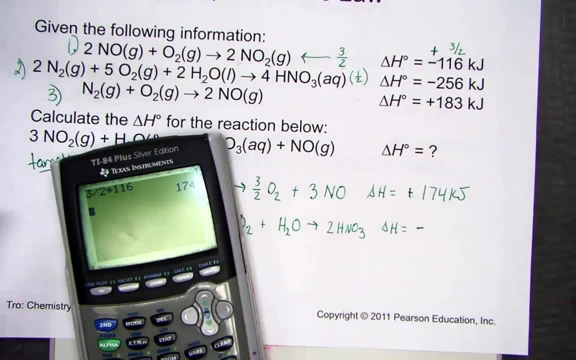 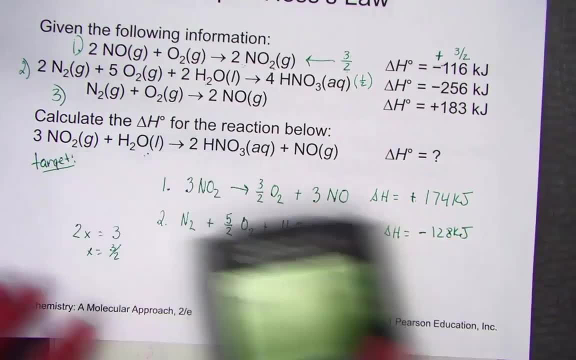 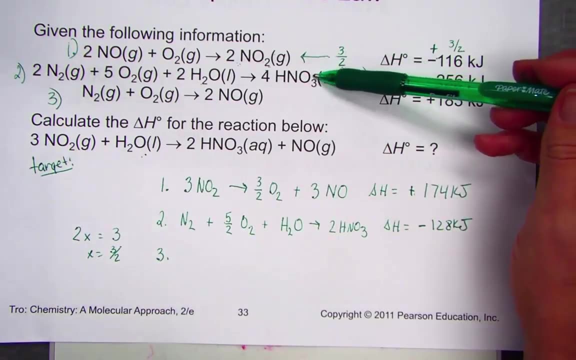 Now I'm going to leave the sign the same: It's still negative. But 256 cut in half is 128 kilojoules. All right, Let's see what else needs to happen. The HNO3s. that's the first product. 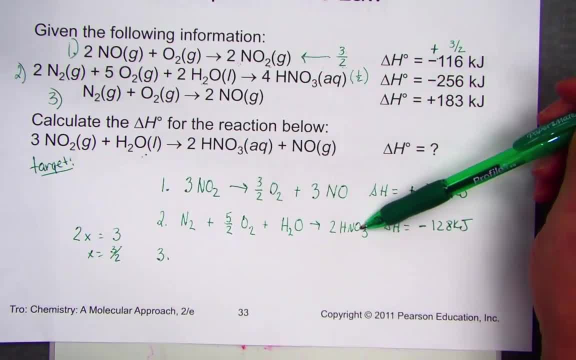 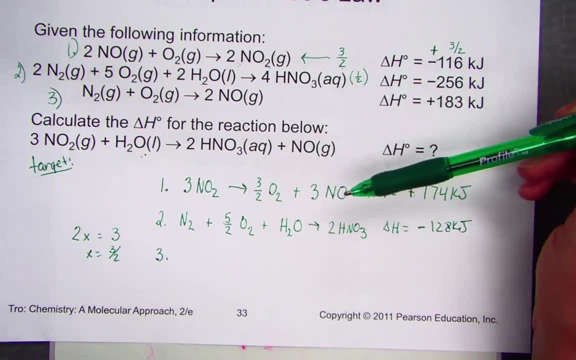 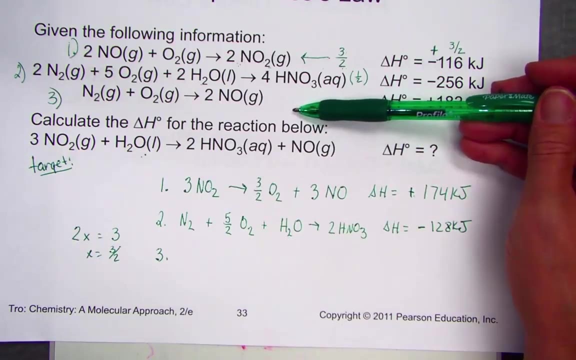 I believe we have taken care of. I see it on the product side in that second elementary reaction And we have the desired amount. We have two units. by cutting the half from up above We have the product NO which appears in a unique position in number three. 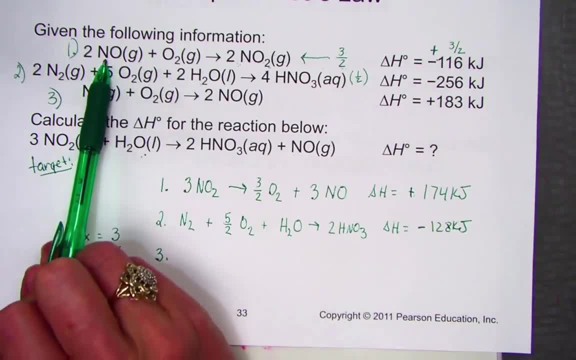 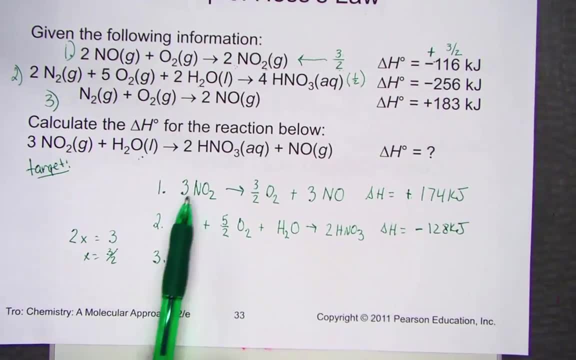 No, it's not unique. I see it in equation one and equation three. All righty, Now equation one. we adjusted. Remember, when I stare at the original equation, there were two units that might appear that we wanted to cancel those out. 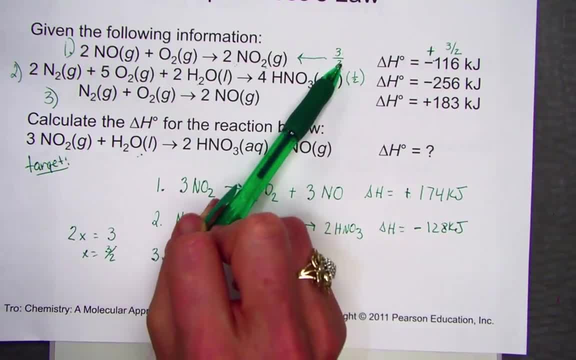 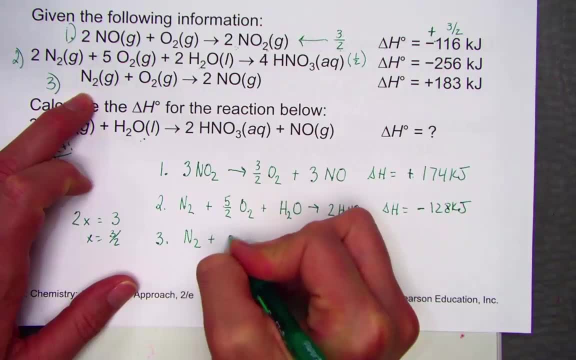 And they would have, except we had to adjust that first equation. So leave the third one alone. Let's just rewrite it as it is. Leave it alone: N2 plus O2 gives us 2NH Gives us 2NOs. 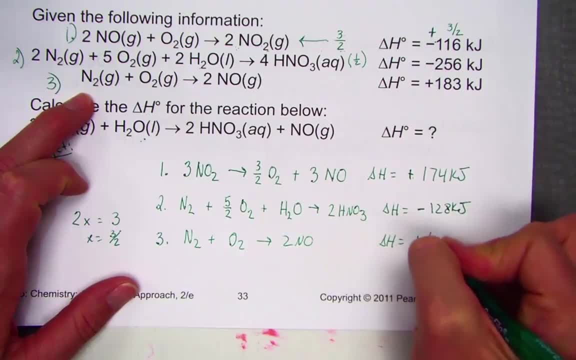 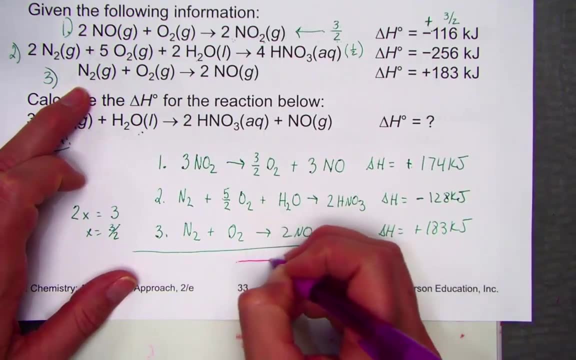 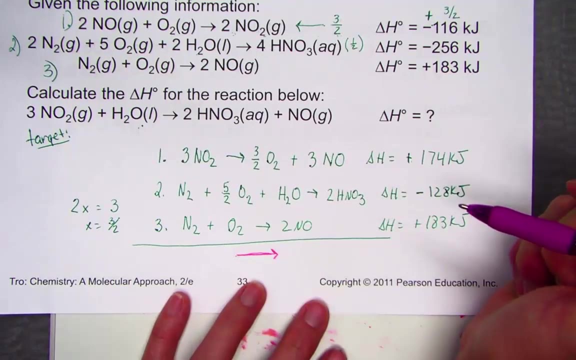 And I didn't do a darn thing, so I'm just rewriting the delta: H Positive 183 KJs. If we add these equations together, simplifying anything from the opposite sides of the arrows, cancel them out, just as you would in algebra. 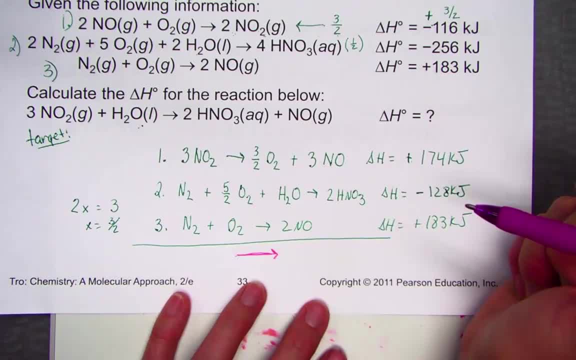 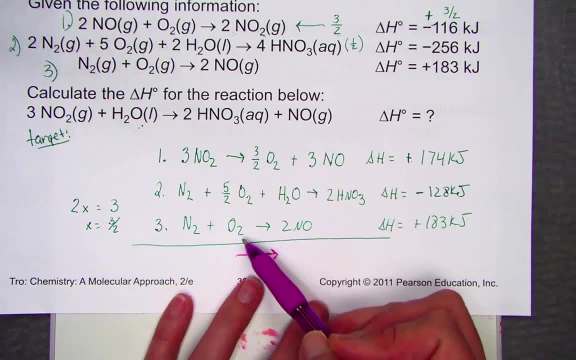 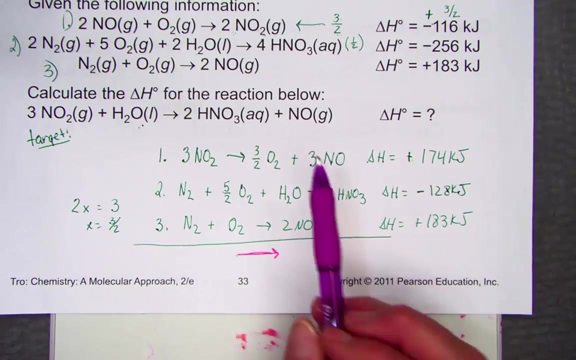 Here's what I'm finding. I have on the left side of the arrow. let's see nitrogens are combining Well, interestingly enough, this number three. I think I made a mistake, But examining is always the secret to figure out if we've done this correctly. 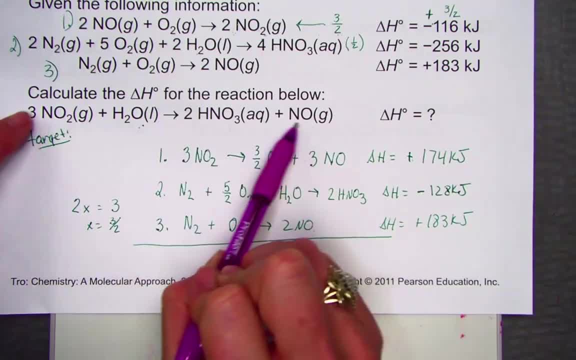 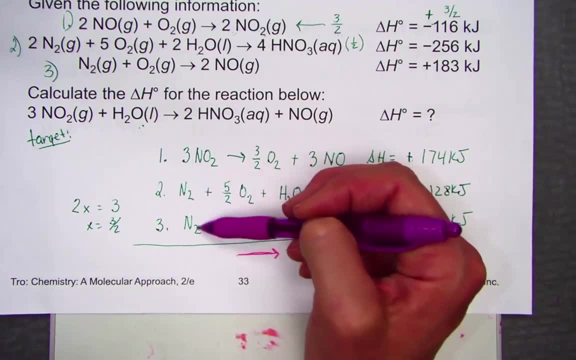 What I noticed is there's no nitrogen in the target equation. You probably noticed that right away. The nitrogens have to disappear. Right now, all the other equations are combining them. That doesn't make sense. I think I need to go back to the drawing board. 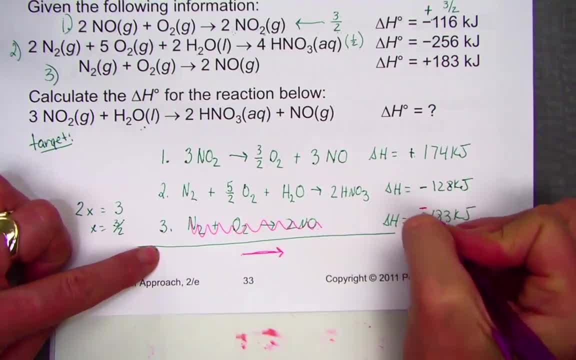 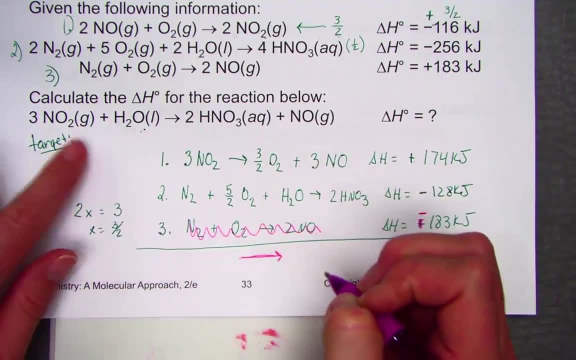 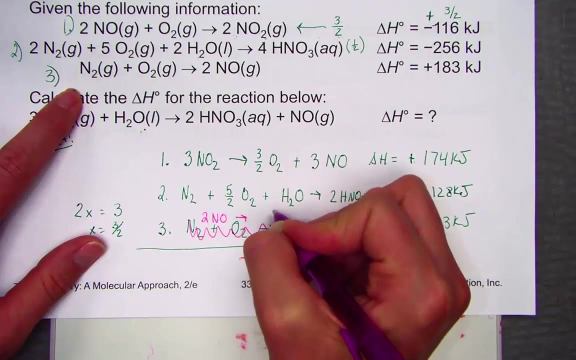 and flip the direction of the third. And if I flip it I've got to change the sign Back the bus up. Let's rewrite the second, Rewrite the third equation in the opposite direction. I bet magic happens. 2NOs yields N2 plus O2.. 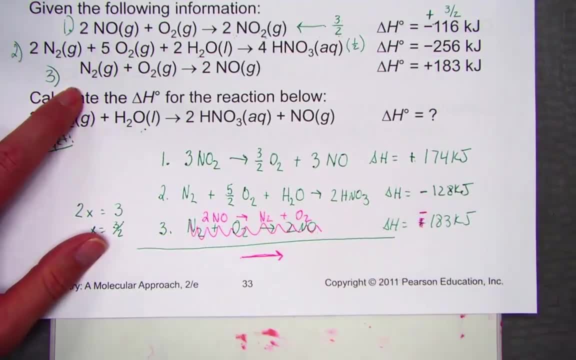 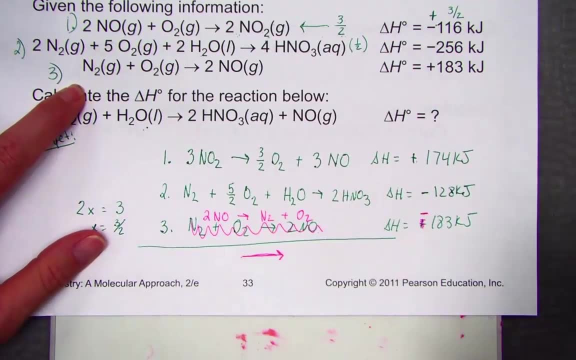 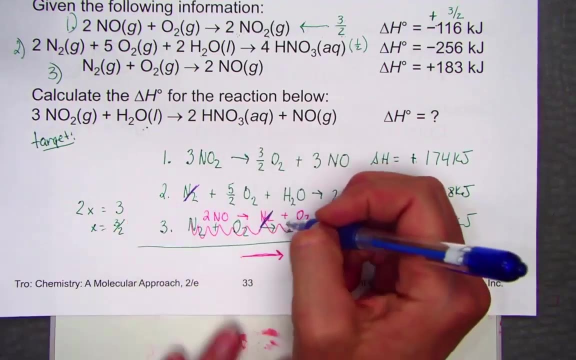 Now I'm seeing it. All right, new color. Here's what we've got going. N2s- now cancel. I have one molecule of N2 on the left in equation two, one on the right in equation three. They cancel. 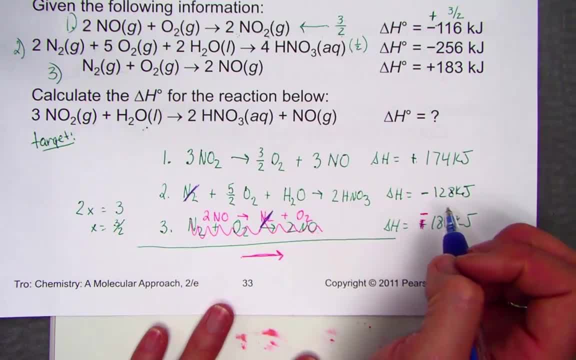 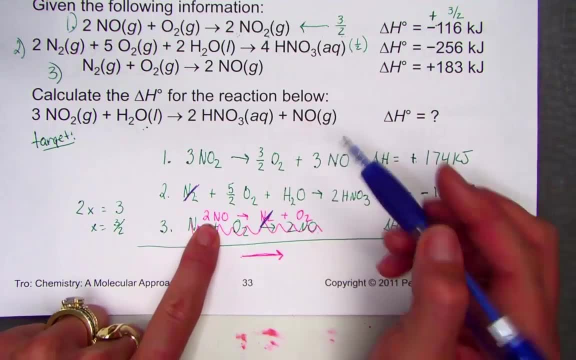 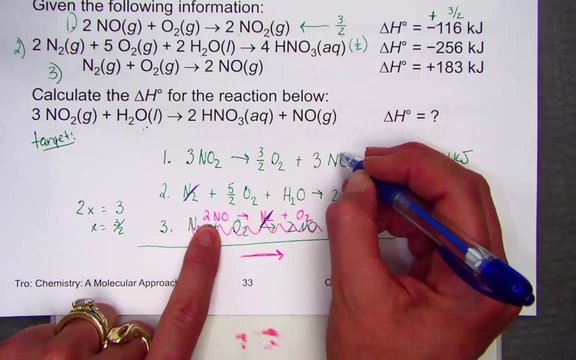 What else might cancel or simplify? I have. how about here Two molecules of NO on the left in equation three, three molecules of NO on the right in equation one. That can be simplified? That's the whole reason I knew to flip this one. 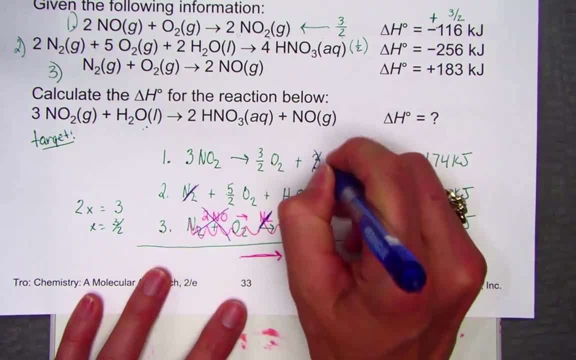 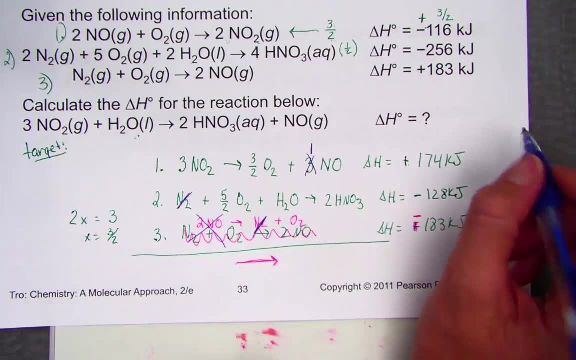 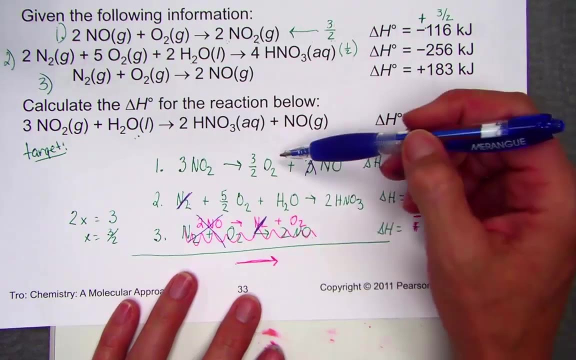 Two units of NO. leave me a net remainder of one NO in that top equation. Here's what else we see: On the left side of the arrow in equation two there's five halves of oxygen. On the right side is some oxygen in both equation one and three. 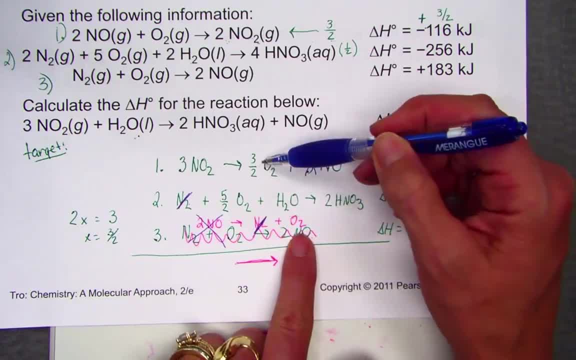 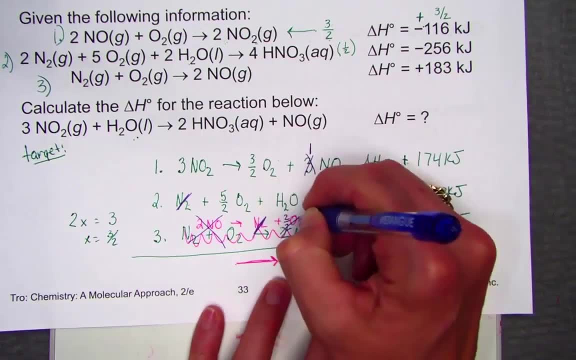 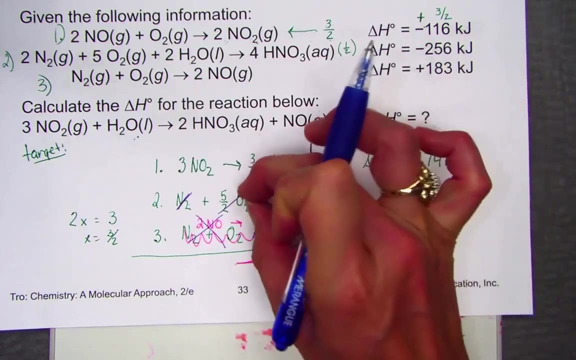 Three halves and one whole more is the same as five halves. Think of this as two over two and you can simply add three plus two to make five halves. That's going to simplify and the oxygens are all gone. Five halves combined on the right can simplify. 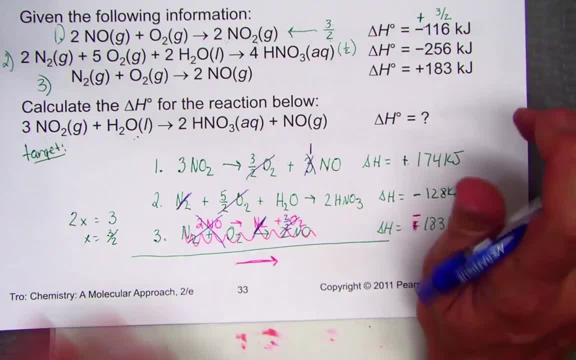 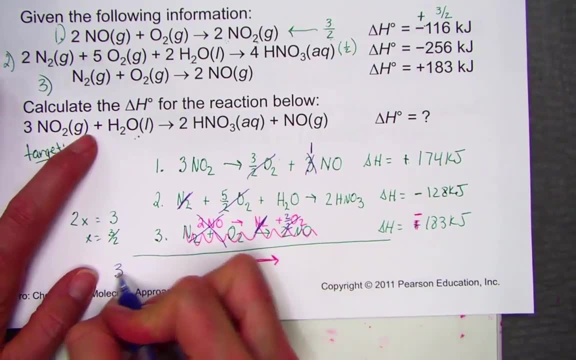 with the five halves written in equation two And I think we've got there. I had one little flip in equation three that I had to repair, but here's what's left over. Equation one has three units of NO2.. That's the first target reactant. 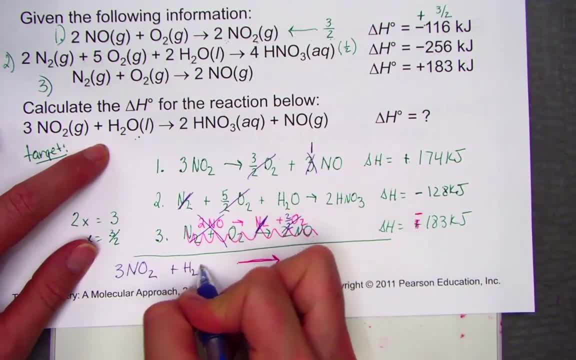 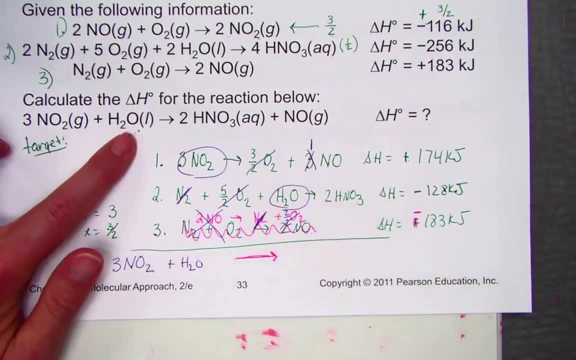 I see in equation two a reactant, and that's the water molecule. That's cool because there it is. It's in our target. Those are the only two reactants left over and they match the target. Let's look to the right side of the arrows. 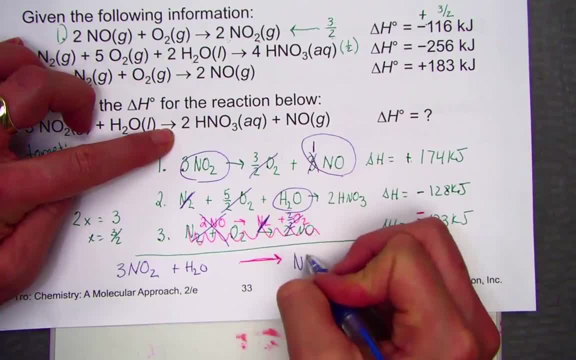 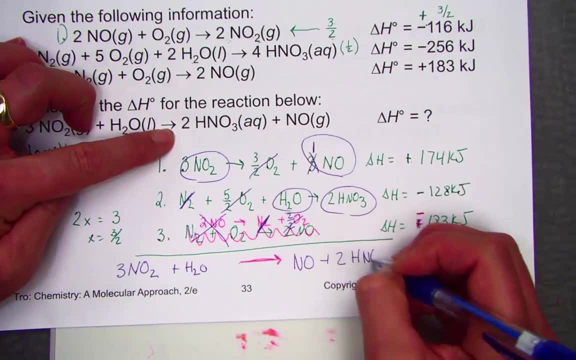 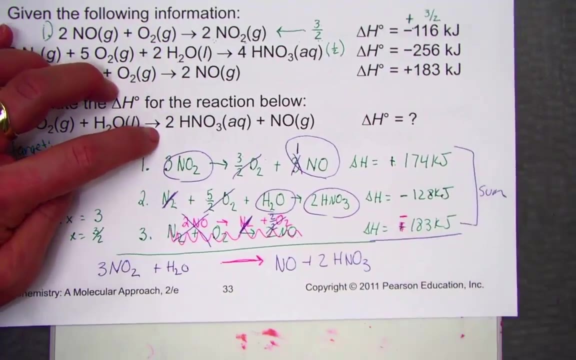 I have one molecule of NO that did not cancel out- and that's in our target, and two molecules of HNO3.. This indeed matches the target equation. The only thing left to do is to sum the three delta H's to get the new equation. 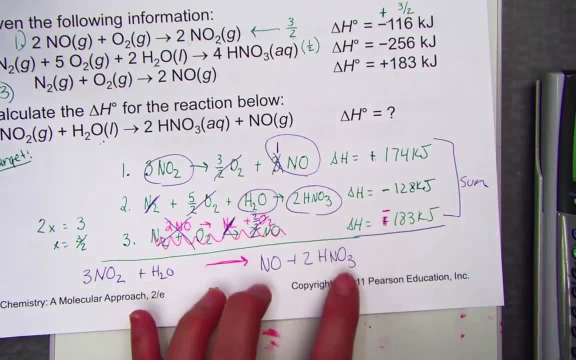 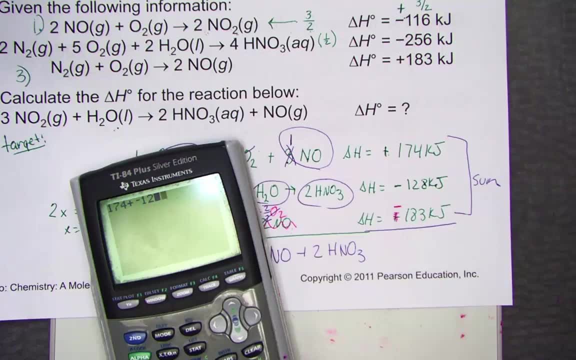 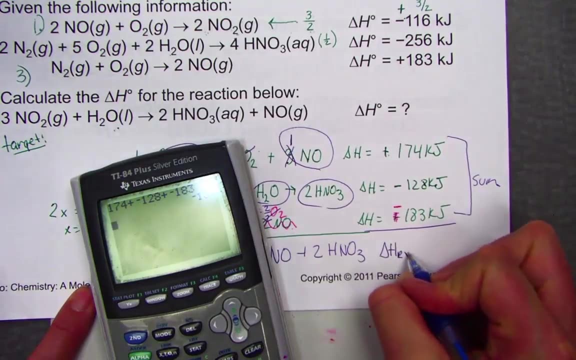 Add together what we've calculated, So positive 174.. Let me show the calculator: Plus negative 124. That's 28.. Plus a negative 183. And the heat of our reaction for the target equation is negative 137 kilojoules of heat. 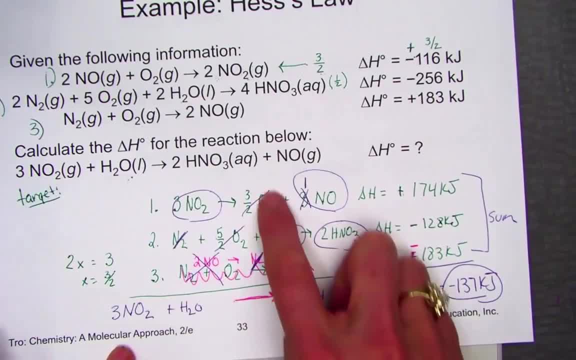 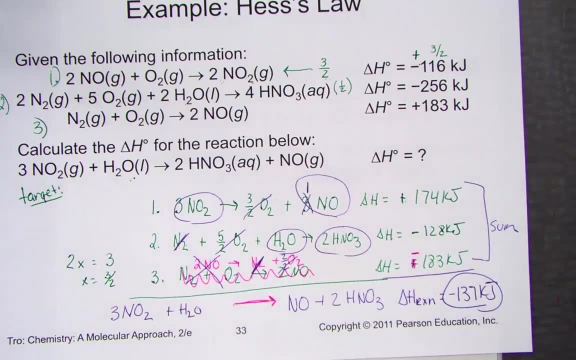 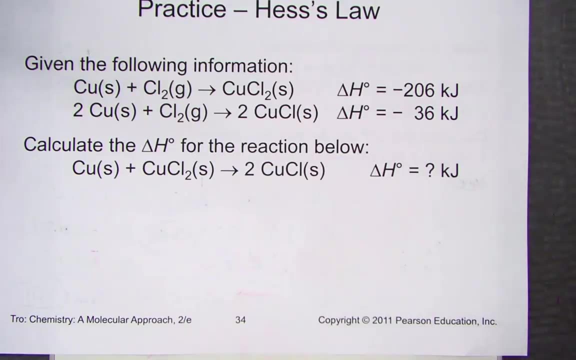 Hess's Law, Little puzzles. What can I do with these elementary reactions so that when I combine them back and simplify, I've built the target? I like them as little mental practices, little puzzles. Obviously, I gotta keep trying if something isn't working. 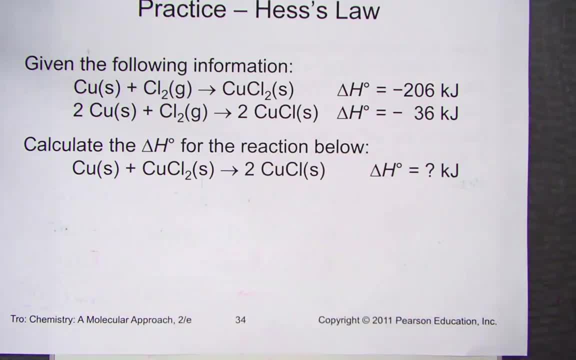 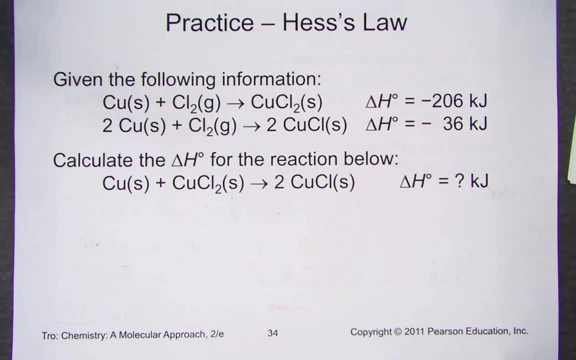 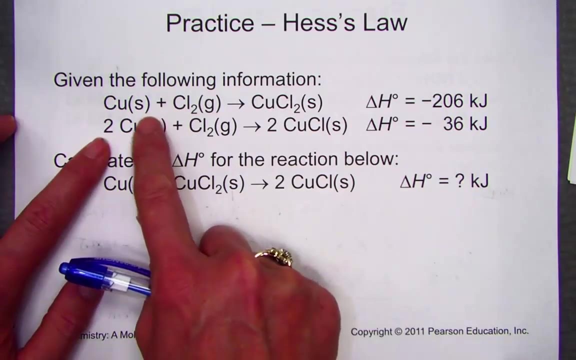 Pause the video, take a look at this next practice and, when ready, play it. Here's our next practice in Hess's Law. Let's see if we've reached a common answer. As I read, the first elementary reaction- copper- is combining with chlorine. 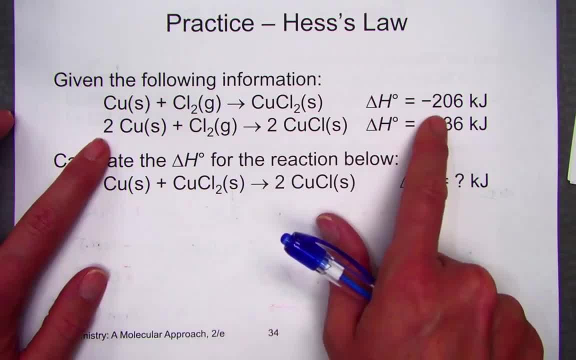 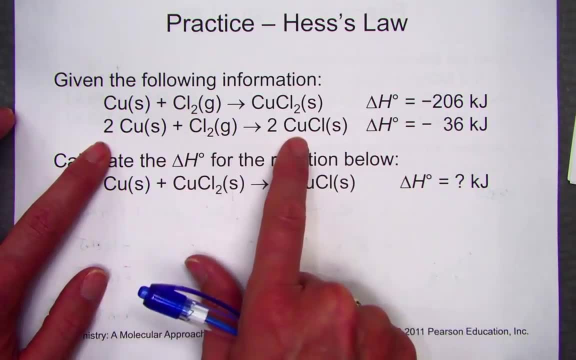 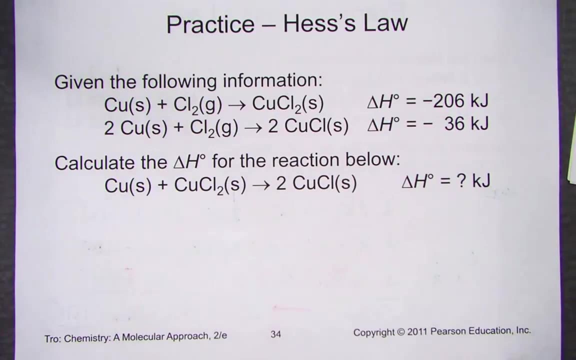 to produce copper chloride, an exothermic reaction. Second equation: Two coppers with a chlorine produce two units of copper, one chloride- Different names based on the charge of the copper- Again an exothermic process. How can we combine these two reactions? 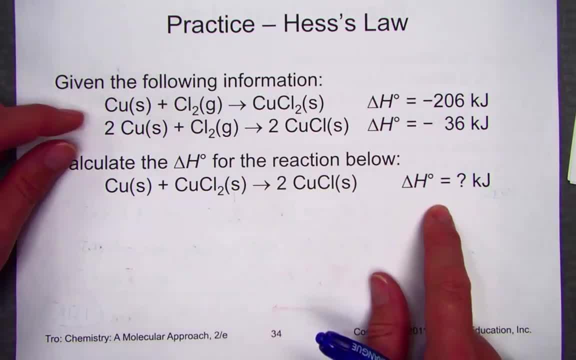 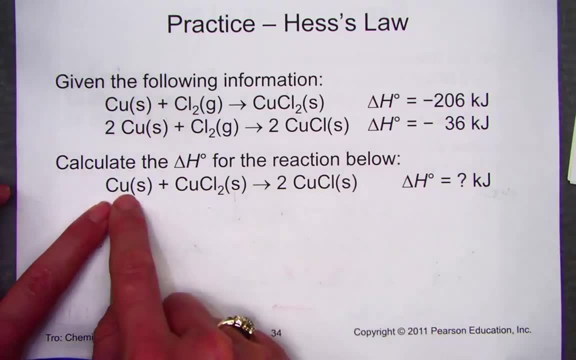 to form the target equation. Building from these two, let's create the target. Well, again, I like to start- for no other reason than it's written- first with the first reactant in the target equation. Here's what I like about it. 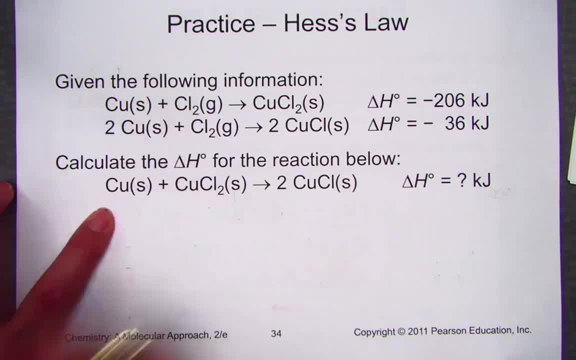 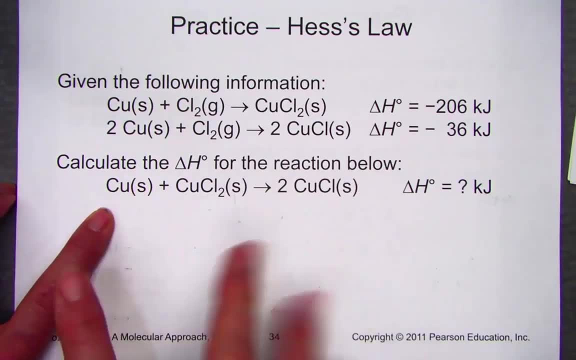 Copper as a solid is written on both sides of the equal here, so it's not in a unique position. The first reactant: I'm really not finding too helpful to get any ideas what to do with the elementary reaction. Let's see if we can find something else unique. 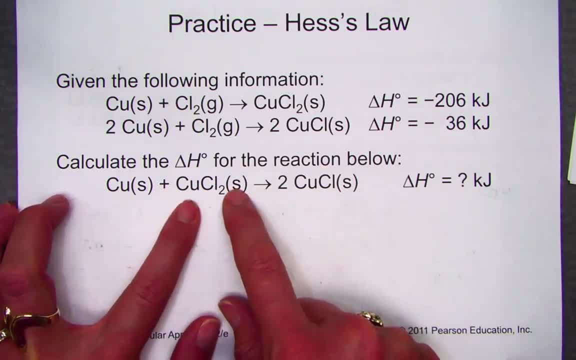 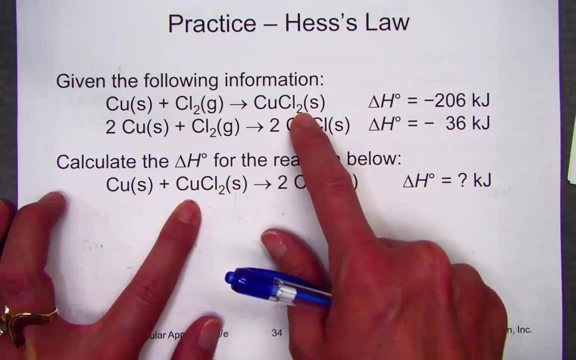 Here is copper chloride as a solid, and that particular reactant is in a unique position. Only one of them appears, and it's in the first equation. I like how many I have, but it's on the incorrect side of the arrow. 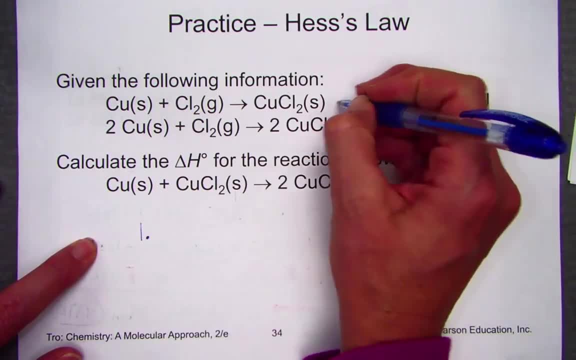 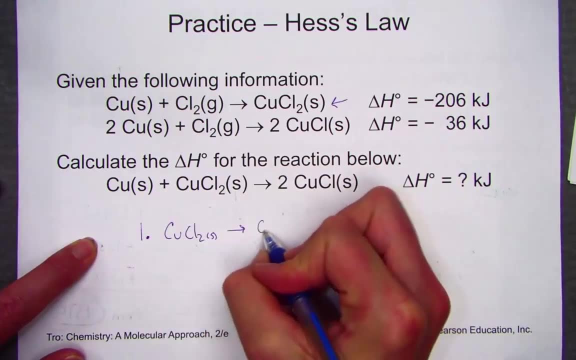 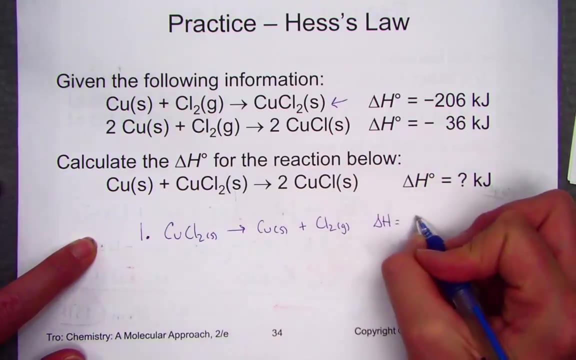 So I think what I'm going to do is rewrite this first equation and flip its direction, So CuCl2 as a solid will go to Cu as a solid and Cl2 as a gas. Since I flipped the direction, the delta H goes from negative. 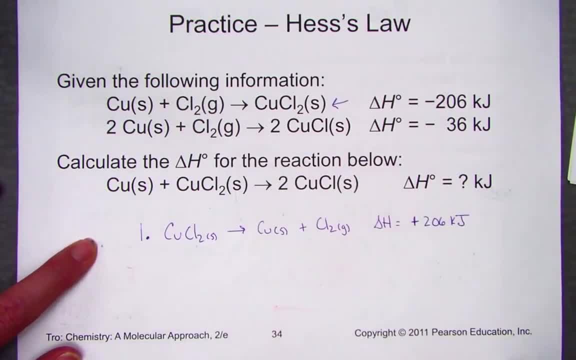 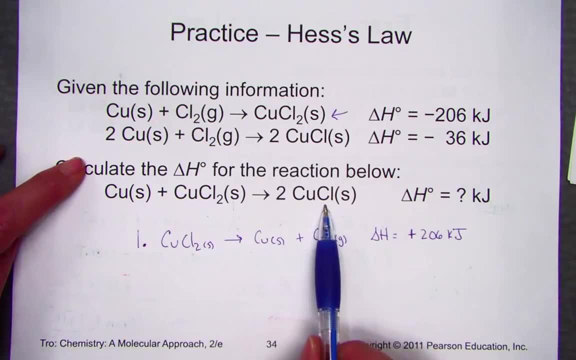 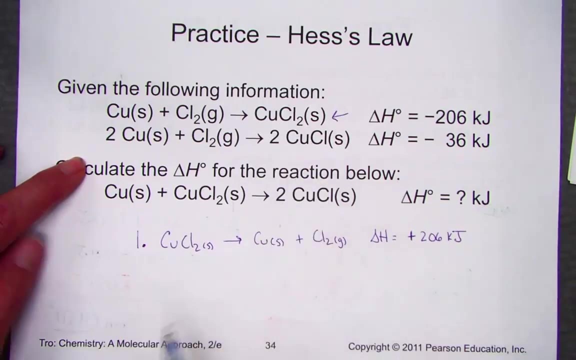 to positive 206 kilojoules of heat. Let's see what else we have. The product is two copper chloride solids. Well, that's exactly written in the correct position in that second equation above, and it's the correct number. Could it have been as easy to flip the first? 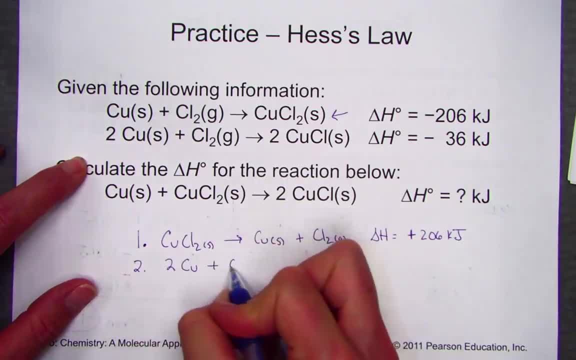 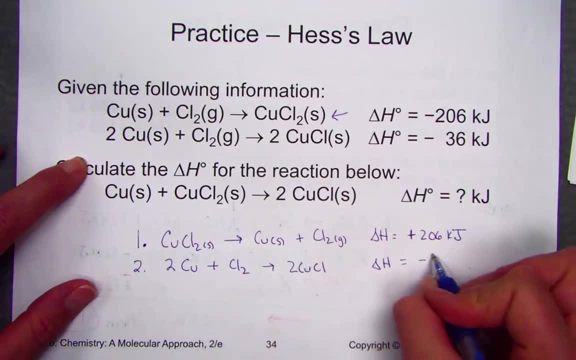 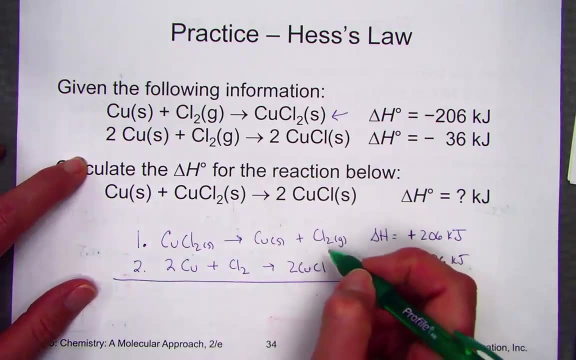 and leave the second. Let's take a look. If our strategy indeed is correct, it should simplify to create the target. If I flip the first, leave the second as is, Let's see. if indeed it simplifies, I notice chlorines will cancel out. 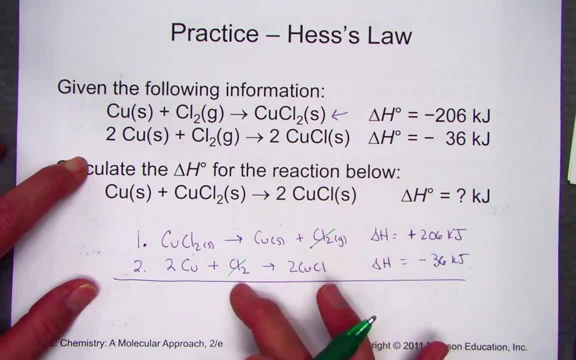 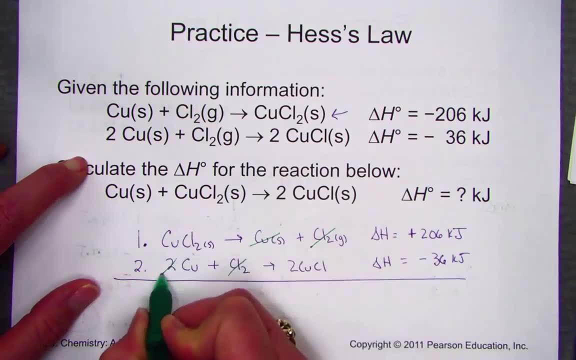 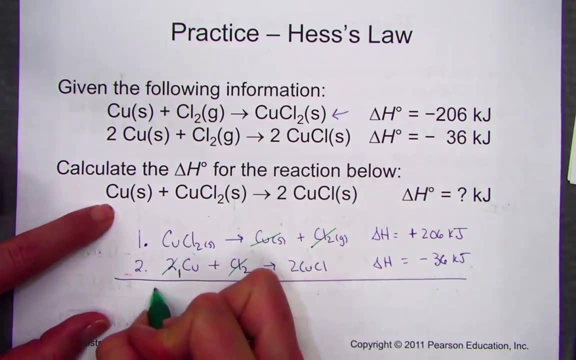 It's a product in the first equation, a reactant on the other, They will cancel. I have one unit of copper solid, two units on the left in the second equation. That's going to give me a net of one copper. I think it really was that easy. 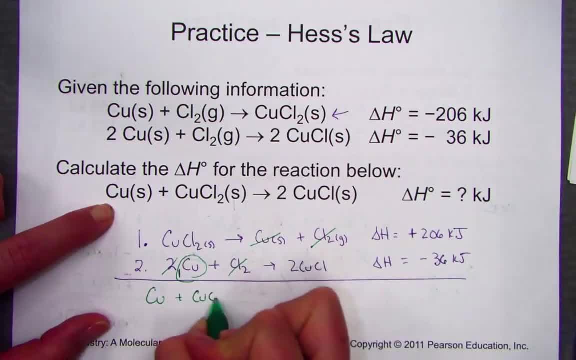 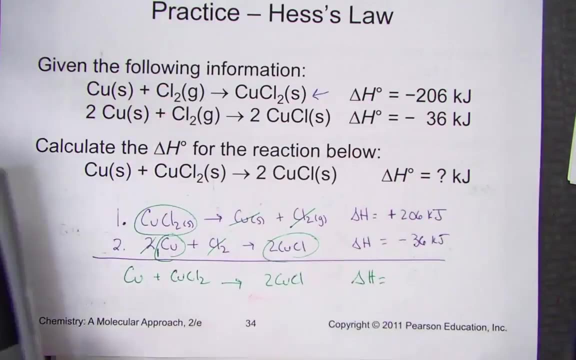 One copper is remaining, plus CuCl2 on the left side of the arrow, giving us two copper chlorides, the only products left in our equation. All we have left to do is to add to find the new heat of reaction. We'll take positive 206. 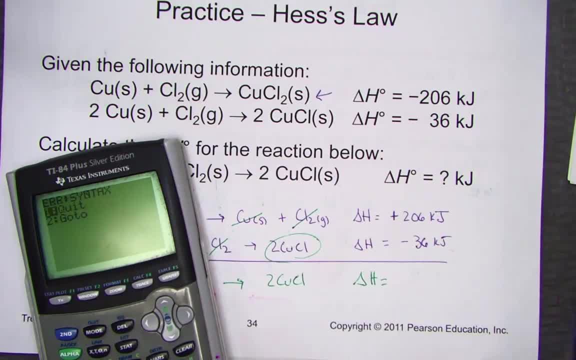 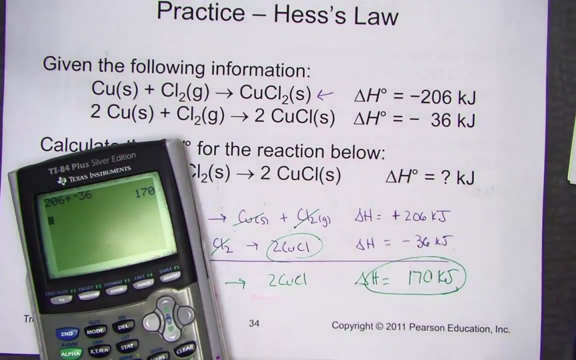 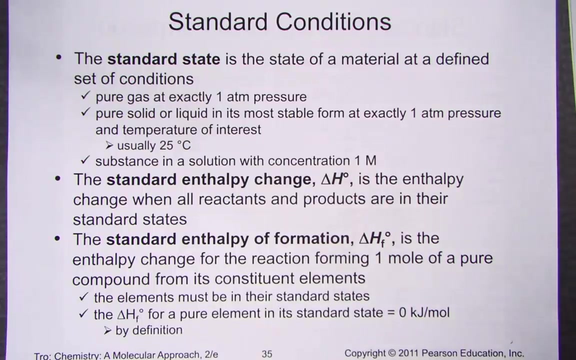 and add a negative 36.. I'll try that again: Positive 206 plus a negative 36 and we get 170 kilojoules of heat energy. Perfect, I hope that matched yours. Our next topic to be covered is called standard conditions. 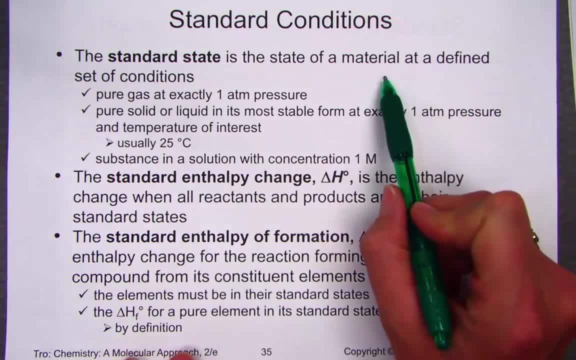 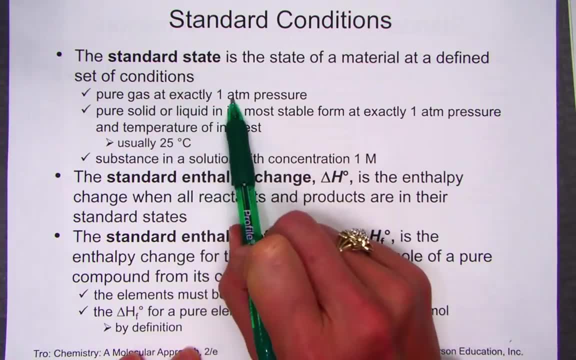 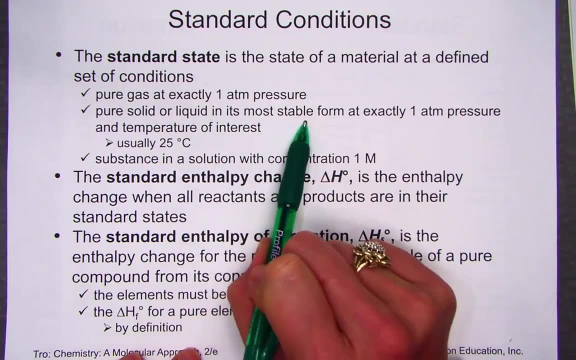 The standard state is the state of a material at a defined set of conditions, For instance, of a pure gas. the standard state would be taken at exactly one atmosphere of pressure. A pure solid or a pure liquid in its most stable form at exactly one atmosphere of pressure. 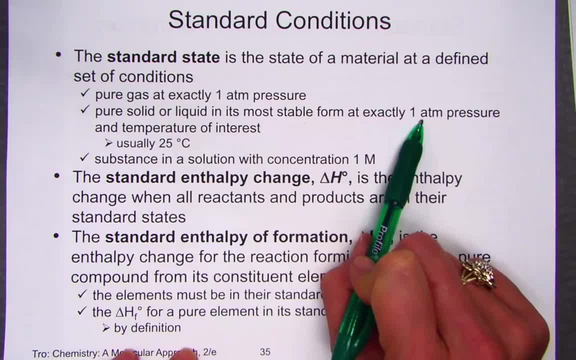 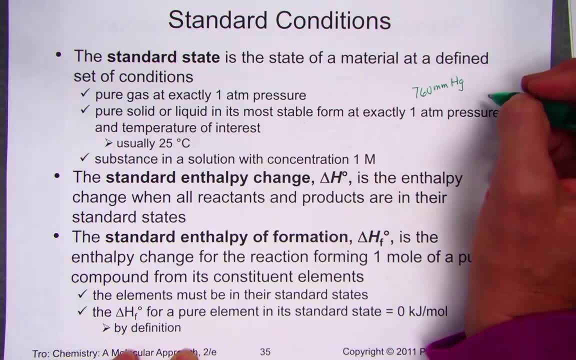 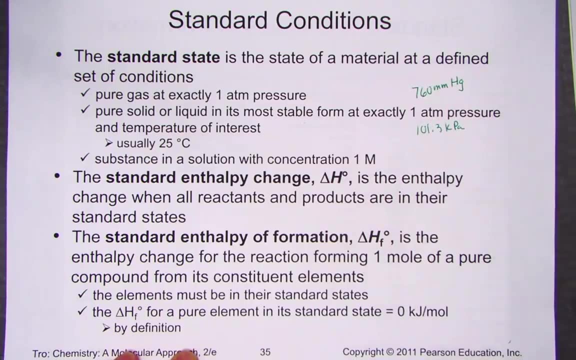 Standard pressure is typically one atmosphere From our gas law units. perhaps you remember other pressures: 760 millimeters of mercury, we called tor, is another standard value. 101.3 kilopascals is another standard value, which happens to be the metric system. 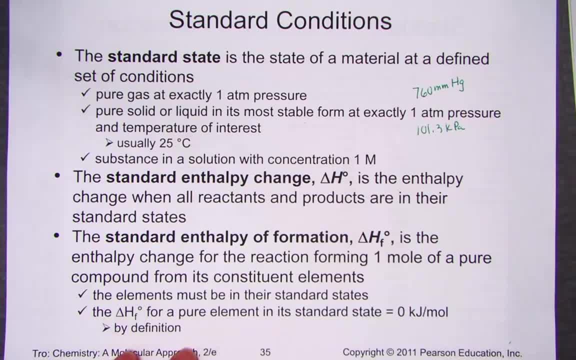 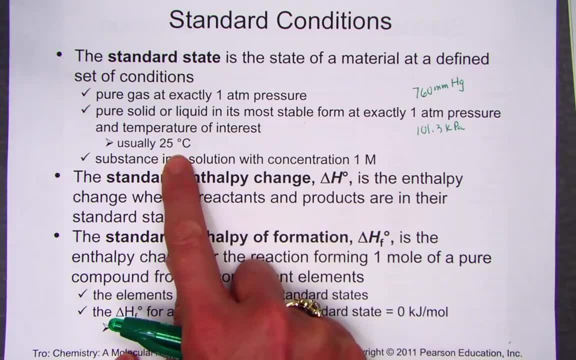 Standard pressure is going to be defined as the standard state of any solid liquid or gas as its natural condition. Temperature is given as room temperature, 25 degrees Celsius, And the standard state of a solution is taken as one molar, one mole per liter. 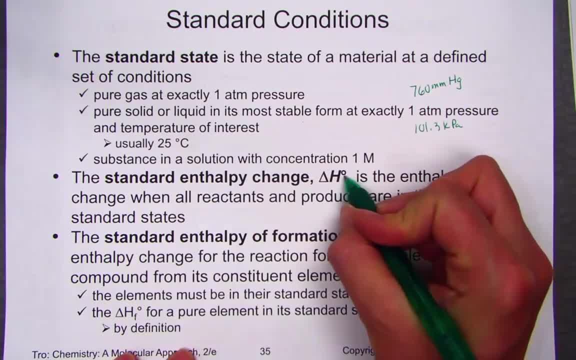 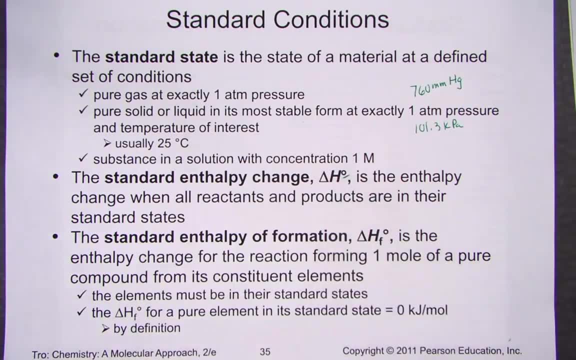 Standard enthalpy change is now going to be given just a little symbol to represent that we've been measuring this in a standard state condition And you'll just see that with a super knot after the H Defined as the enthalpy change when all reactants and products 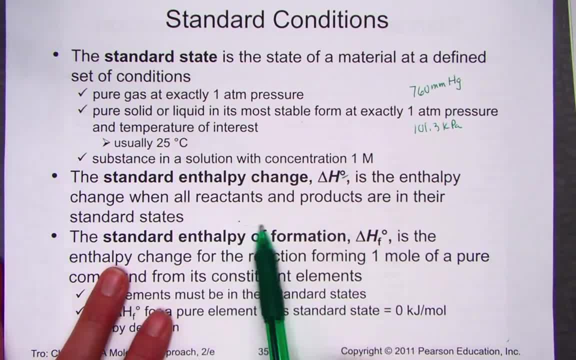 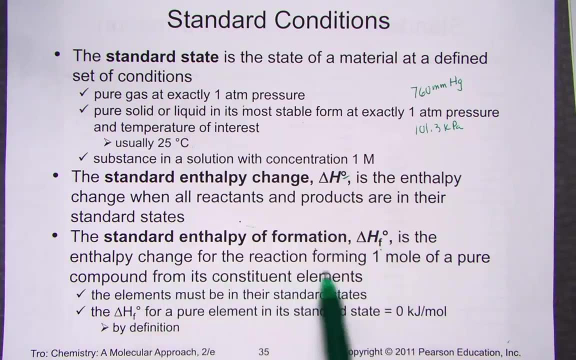 are, in their standard states, running the reaction at standard pressure and temperature of 25 Celsius. The standard enthalpy of formation, given with a sub F, after heat of formation, the enthalpy change for the reaction forming one mole of a pure compound. 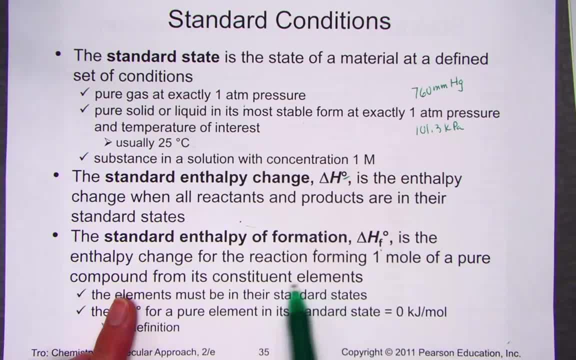 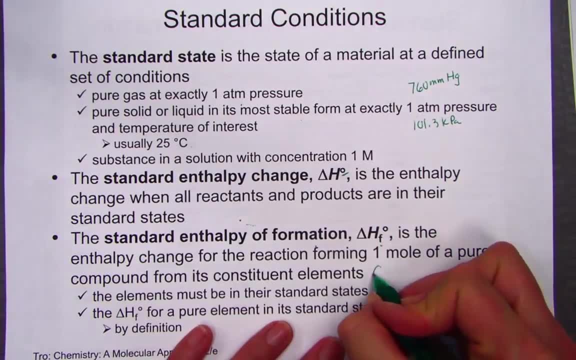 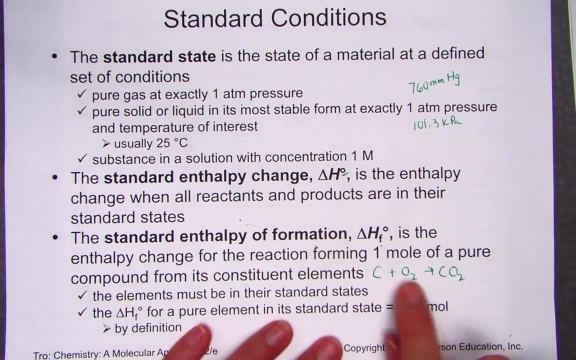 from its constituent elements. Constituent means just one of those made up from the compound. The constituent elements of carbon dioxide would be carbon and oxygen Found in the natural state. carbon is written as C. It's a solid Found in its natural state. 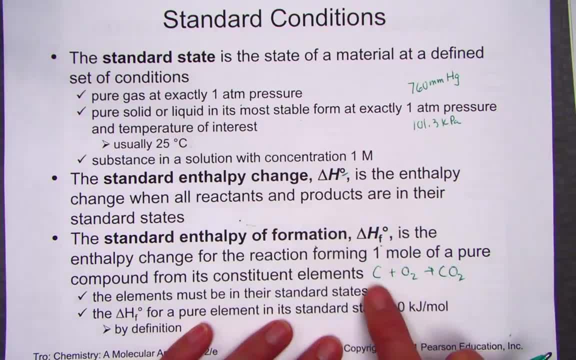 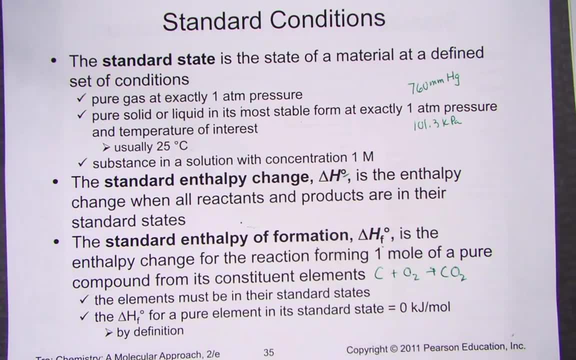 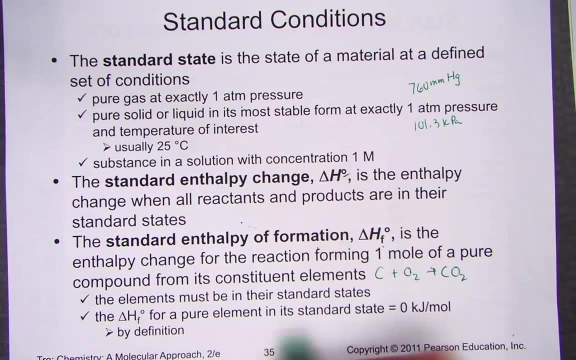 oxygen is the diatomic molecule Forming a compound from its standard state. constituent elements is called the heat of formation. Pure elements are not made in nature. That's what we find and build compounds from. If a pure element in its standard state is found in nature, 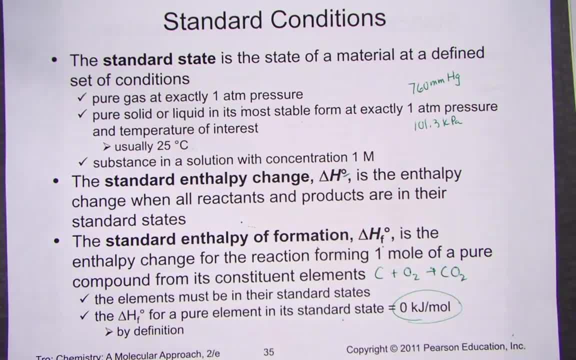 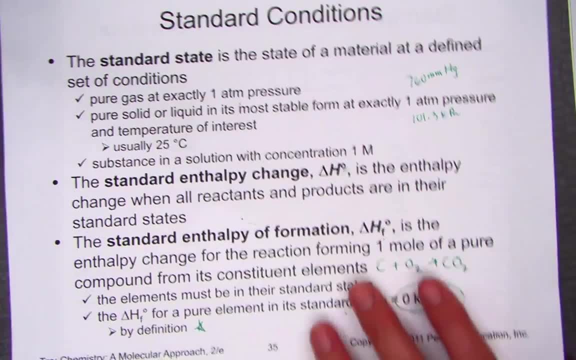 it's just given a value of zero kilojoules per mole. That's the very definition of heat of formation. We do not form elements. We build compounds from them. Here's a chart that deals with the standard enthalpies of formation. 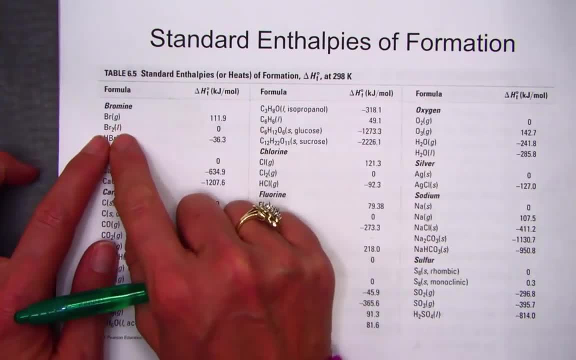 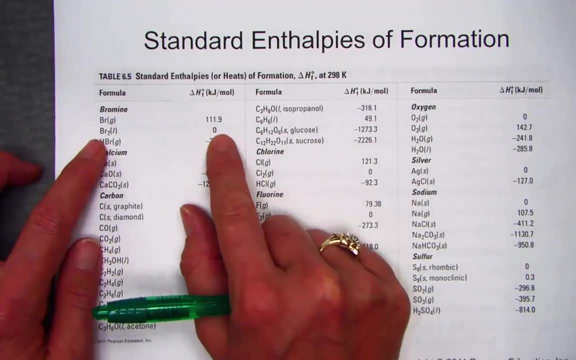 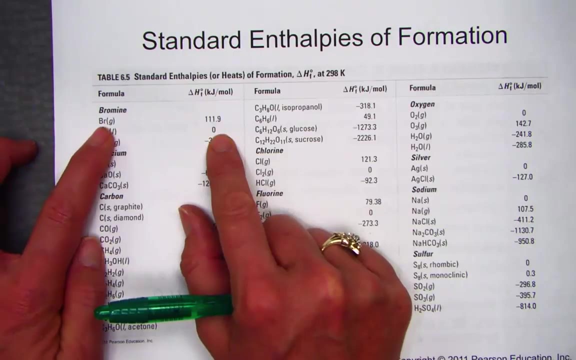 Bromine, for instance, is a liquid at room temperature and it also is one of the lucky seven diatomics. Notice, it has the value of zero. The natural state of bromine is a liquid in a diatomic form. A single atom of bromine in a gaseous form. 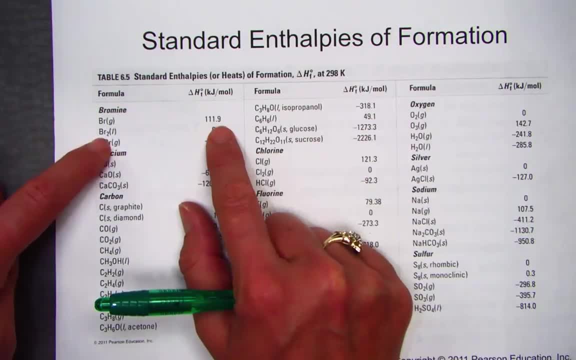 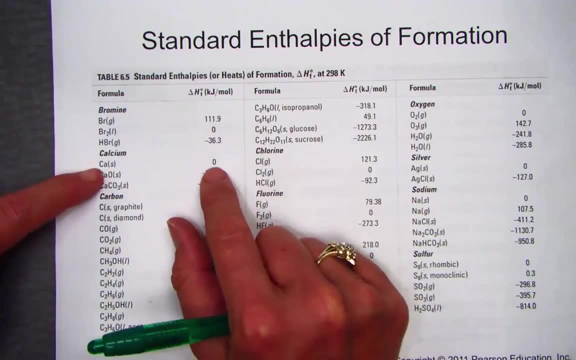 takes energy to build. We'd have to split this molecule to create the unnatural state of atom bromine. Here's calcium as a solid. That's the way we find it in nature. It has the value of zero And I see compounds listed. 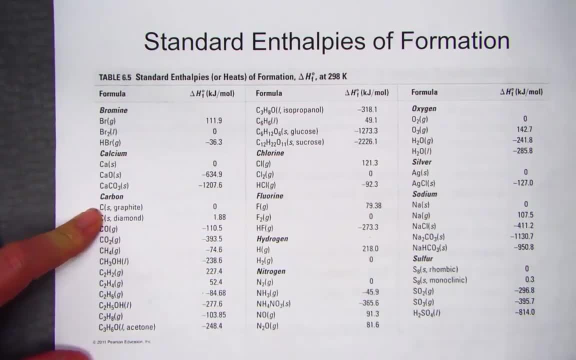 How much energy it takes to build those compounds from the elements it's made of. In nature, carbon is typically found as graphite, which is like pencil lead or a lump of coal Given a value of zero. it definitely takes energy to create diamond. 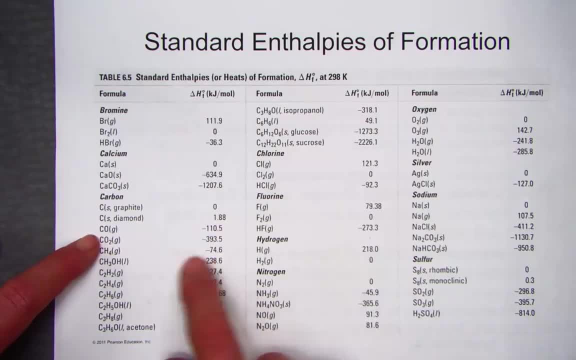 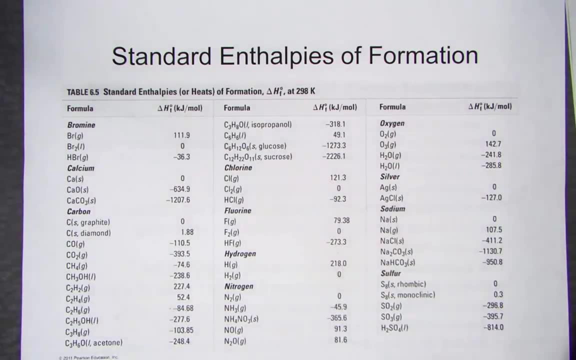 And you can see it has a positive 1.88 value and so forth. So here's a list, in a somewhat alphabetical order, of standard enthalpies of formation. I'm going to keep this chart handy. We'll be using it, as we do some of our math problem examples. 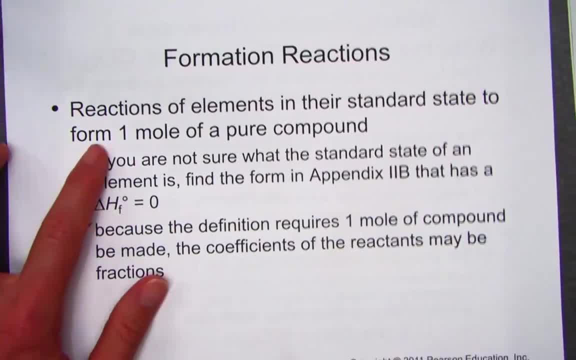 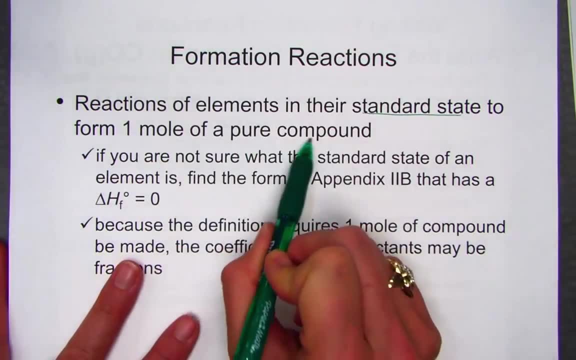 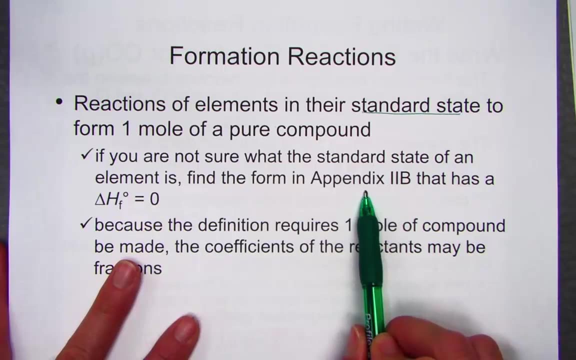 So formation reactions. it simply says reactions of elements in their standard state, the way we find them in nature to form one mole of a pure compound. If you're not sure what the standard state of an element is, we have an appendix in the back of our textbook 2B. 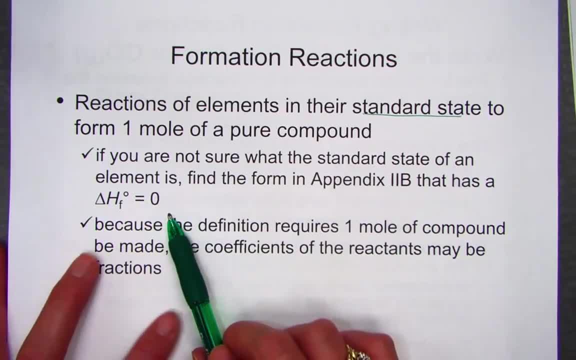 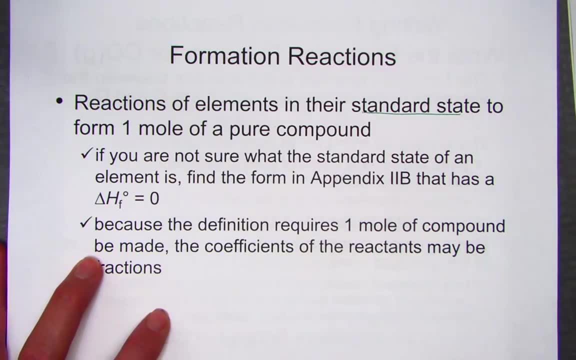 that has a heat of formations for those pure elements. And again I happen to have one in front from the previous slide. That one was taken out of our Table 6.5.. The appendix in the back of your book has a much more extensive list. 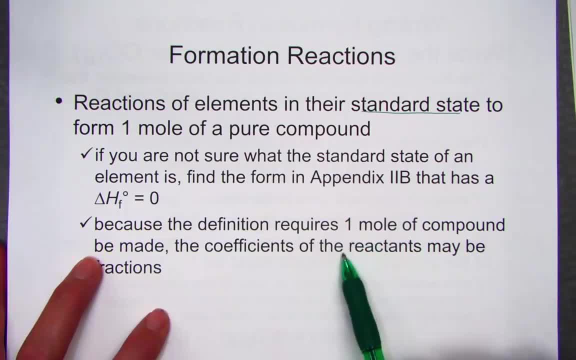 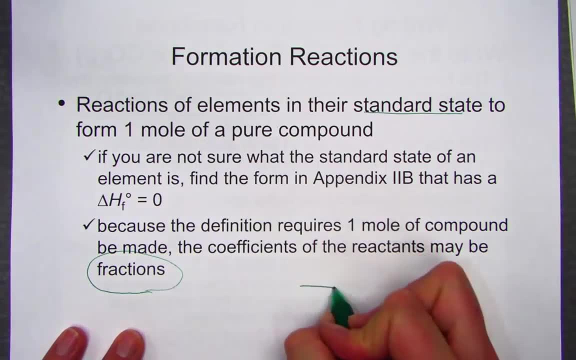 Because the definition requires one mole of a compound be made, the coefficients of the reactants may be fractions. To clarify, suppose I want to build one mole of a molecule called carbon monoxide. One mole of carbon will react with half a mole of oxygen. 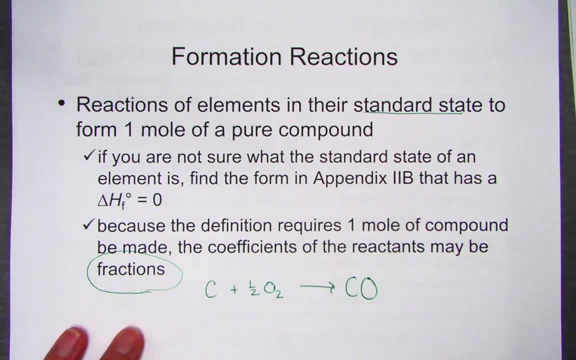 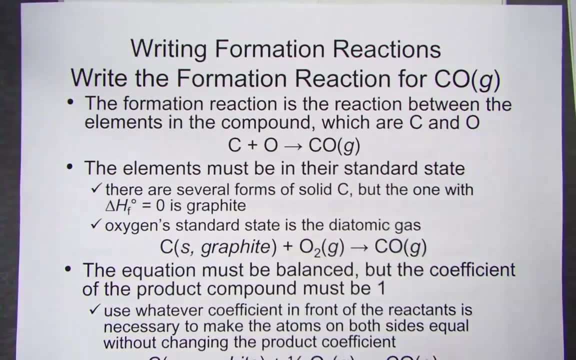 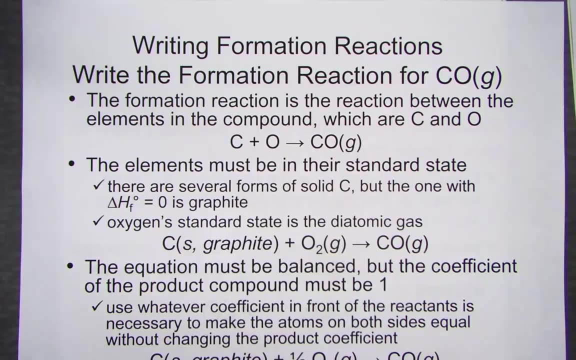 to create one mole of carbon monoxide, So fractions are allowed, simply reading in terms of mole values. The formation of a reaction is the reaction between the elements in the compound, which are carbon and oxygen. But the elements must be in their standard state. 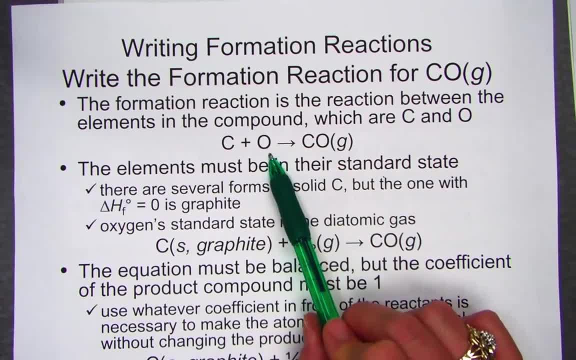 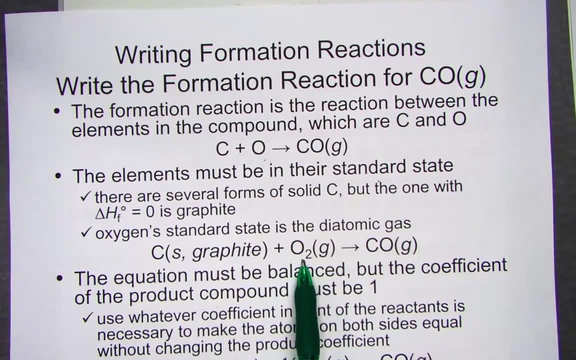 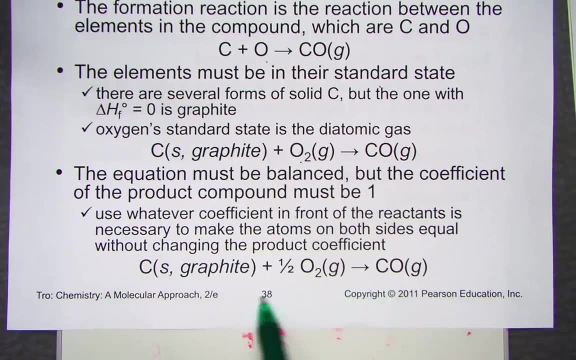 We do not find oxygen as an atom in nature. It's too unstable. Instead, we find it as a diatomic gas and we use the oxygen molecular form to create compounds. And notice what they've done here To keep it balanced. 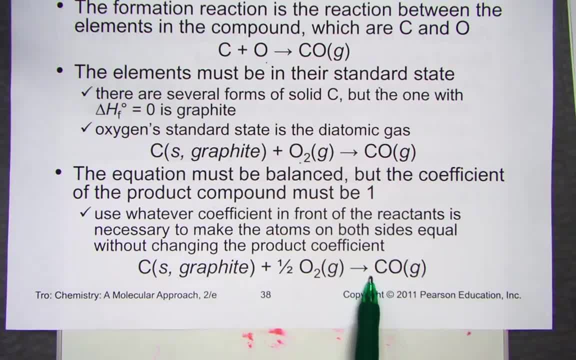 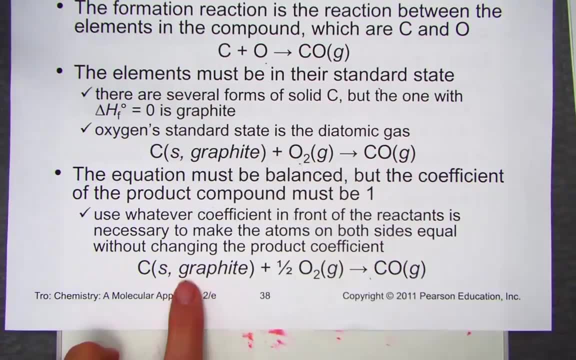 to produce just one mole of a molecule of carbon monoxide, we took one half a molecule of oxygen and combined it with carbon in the graphite form. Carbon in its natural state is graphite. The heat of formation is zero. Again, if you're not sure, 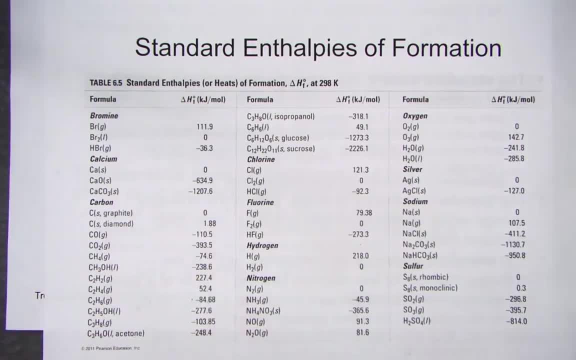 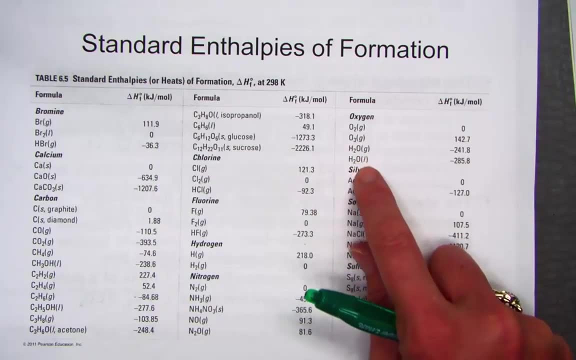 it's found in our appendix. Oxygen in its standard state is a diatomic molecule. Oxygen is a molecular gas. It is zero when it's O2 as a gas, And I don't see it written any other way, so that's my only choice. 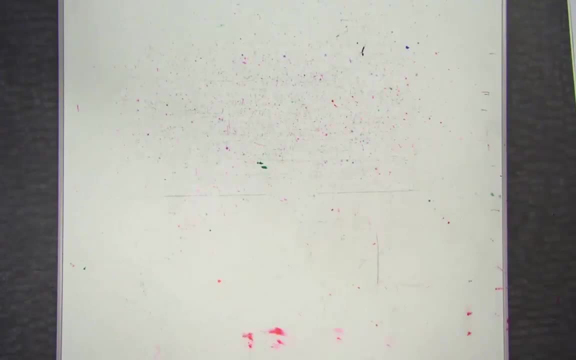 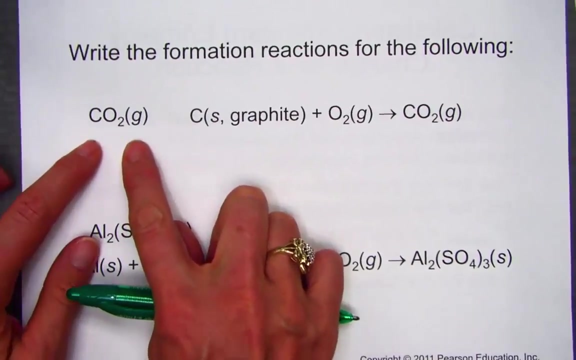 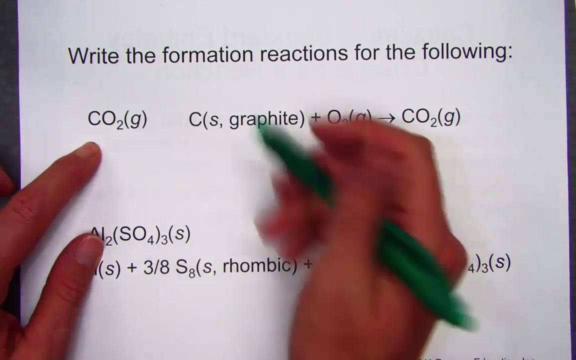 to write it as O2, as a gas. So what might be some heats of formation reactions for the following. Here's an example. If we wanted to create a formula showing the formation of carbon dioxide gas, Carbon is in the form of graphite. 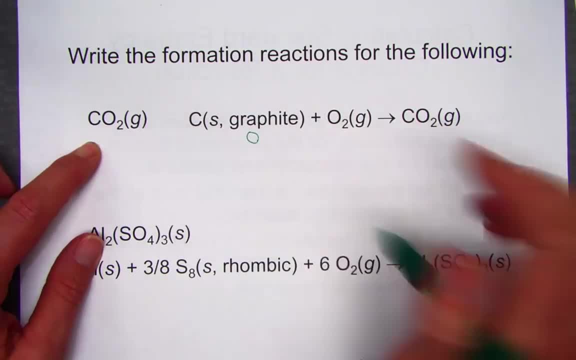 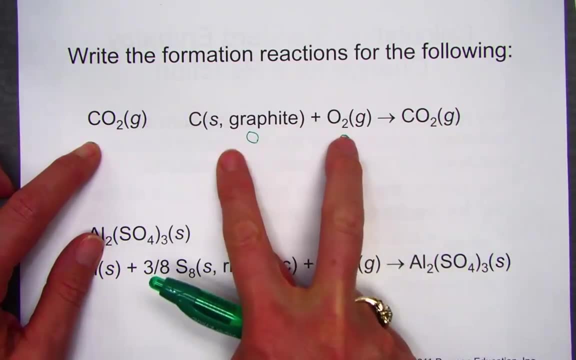 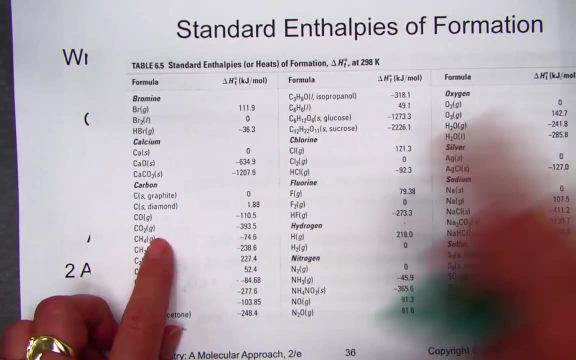 heat of formation of zero Oxygen in its molecular form is a gas heat of formation of zero Carbon dioxide, as a gas is formed from its constituent elements, And I literally can just simply look up carbon dioxide in its gaseous form: negative 393.5 kilojoules of heat. 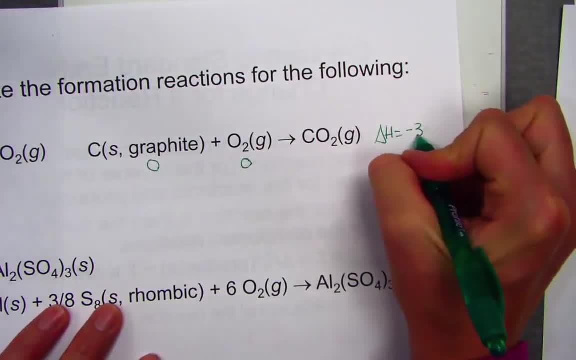 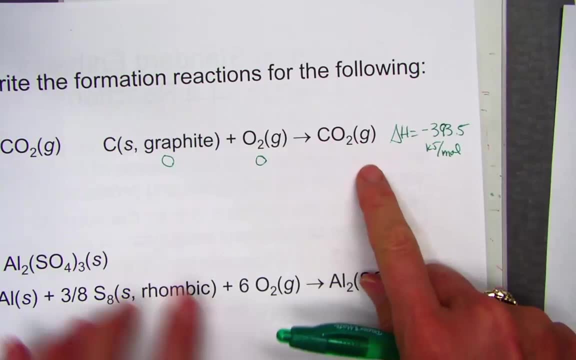 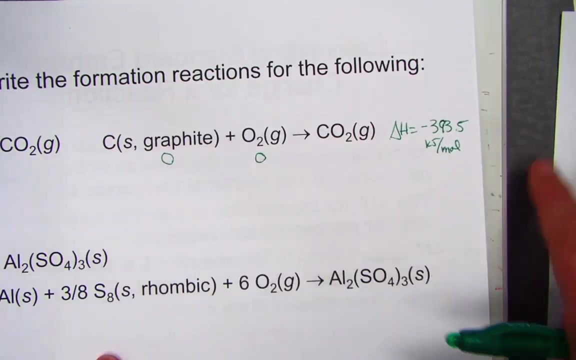 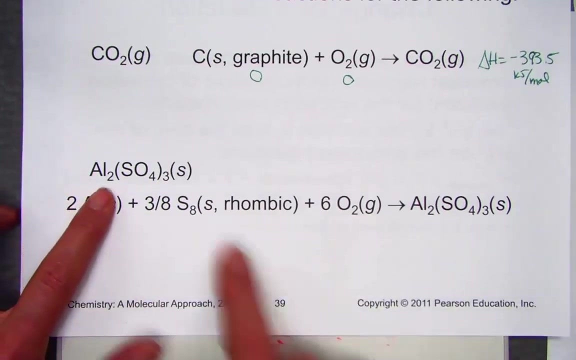 Delta H would be negative. three oh shoot, I lost it. 393.5 kilojoules per mole of CO2 formed The carbon dioxide value built from its natural state elements. This thermochemical equation is exothermic. Suppose we want to produce aluminum sulfate solid. 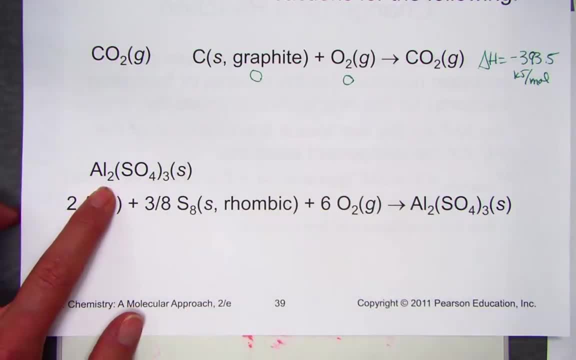 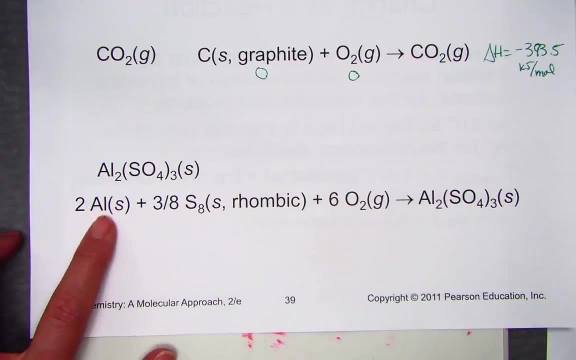 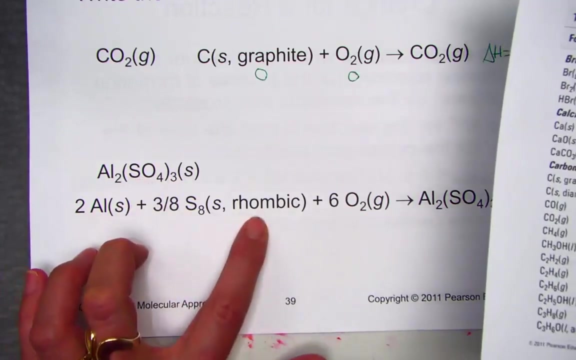 Aluminum sulfate is actually built of three different elements: Aluminum, sulfur and oxygen. Aluminum in its natural state is a solid Sulfur in its natural state is rhombic. S8 is its natural state. How are we supposed to know that? 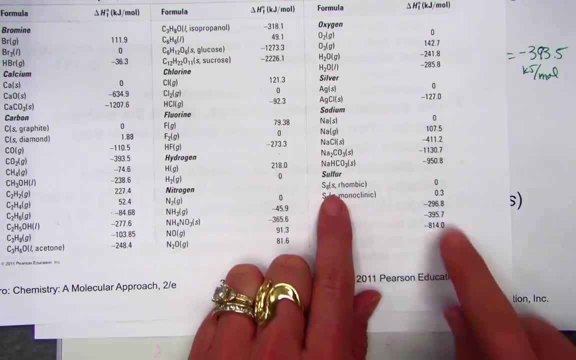 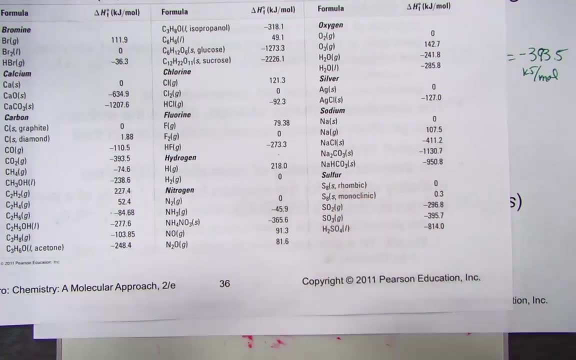 Well, I check it out using my enthalpy of formation. The standard state, the way we find it in nature, has the zero assigned to it And notice it's a rhombic, which is just a geometric pattern of how we find sulfur atoms bonded together. 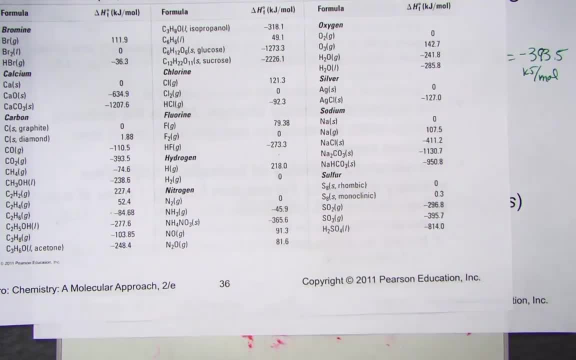 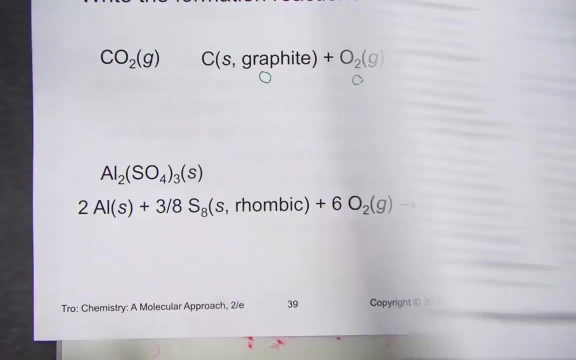 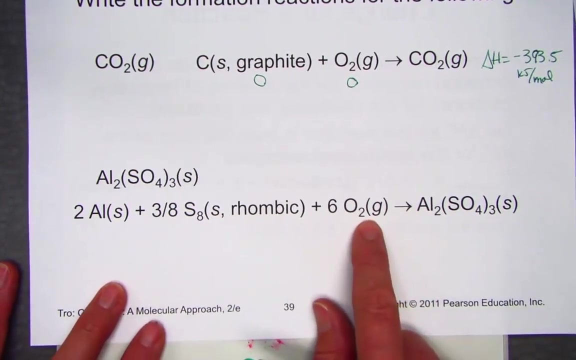 We had diatomic molecules such as oxygen, chlorine, bromine. there were seven of those. This has eight atoms bonded together in a rhombic geometric pattern. So this has an assignment of zero And again, oxygen has an assignment of zero. 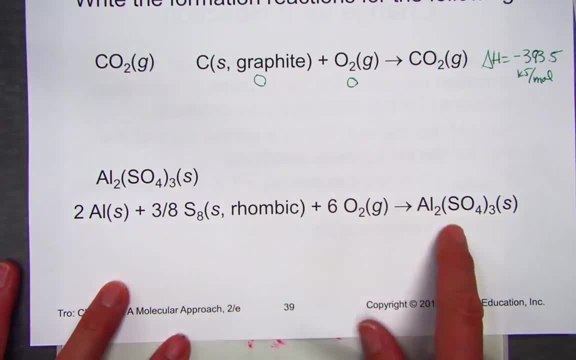 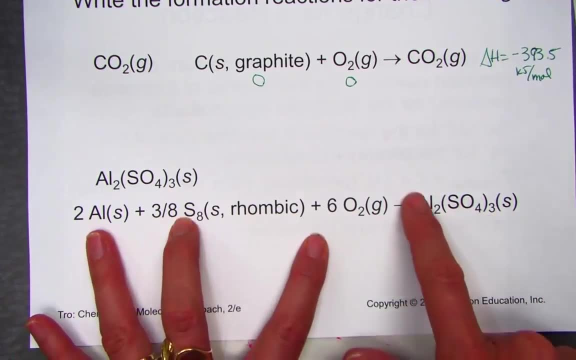 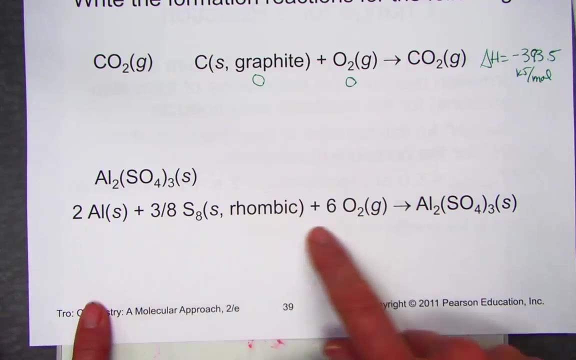 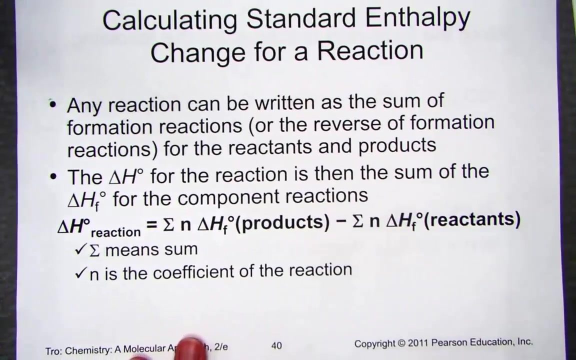 When the three natural state elements combine to form the compound, aluminum sulfate is produced. The fractions here, or coefficients, are simply to create one mole of aluminum sulfate. Notice that we're just taking each element individually to build the compound. When we want to calculate. 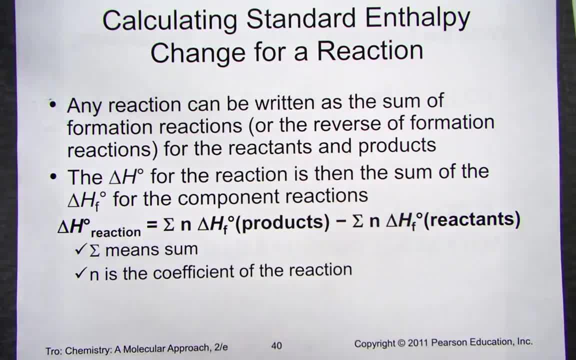 standard enthalpy change for a reaction. we need to have access to that table- heats of formation table- either in your appendix or from printing this particular PowerPoint. But any reaction can be written as the sum of formation of reactions. That's Hess's law. 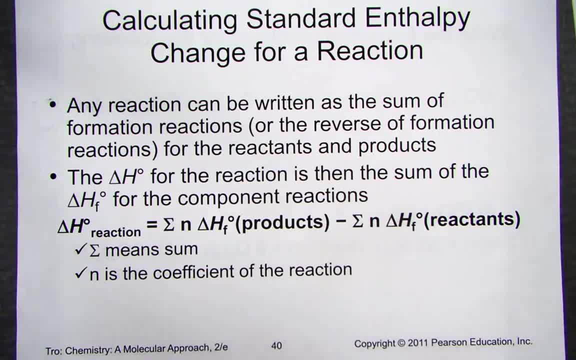 or the reverse of formation of reactions- Again Hess's law: if you flip the direction, we simply flip the sign. So instead of using Hess's law- as tedious as that might be, although I find enjoyable- we've come up with an easier way. 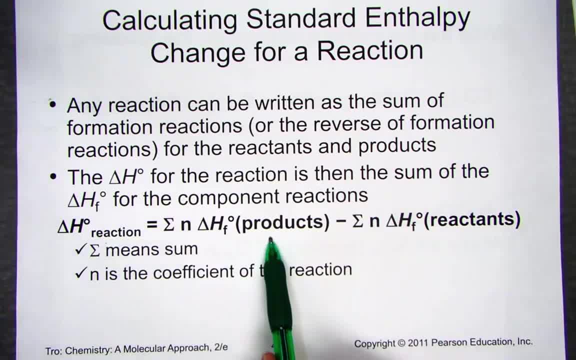 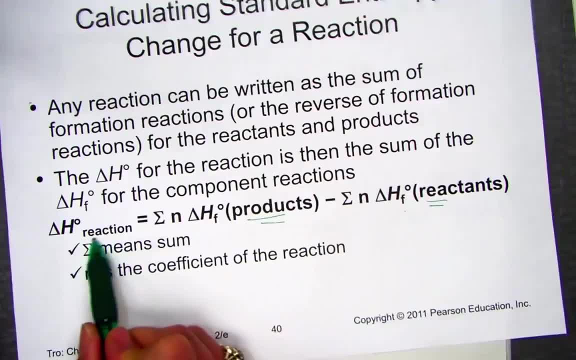 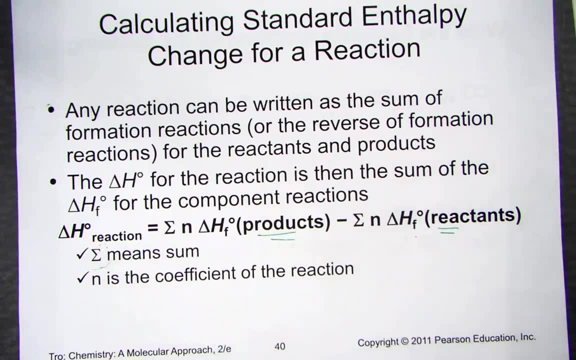 to find a target equation and that's simply taking the sum of the products minus reactants. Products minus reactants will find the sum of the heat of reaction. That sigma stands for sum. It's a Greek symbol. Perhaps you're familiar with it. 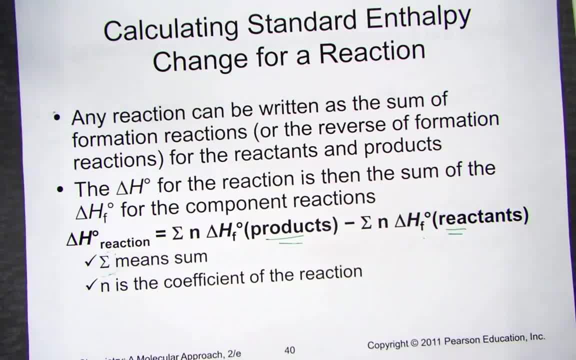 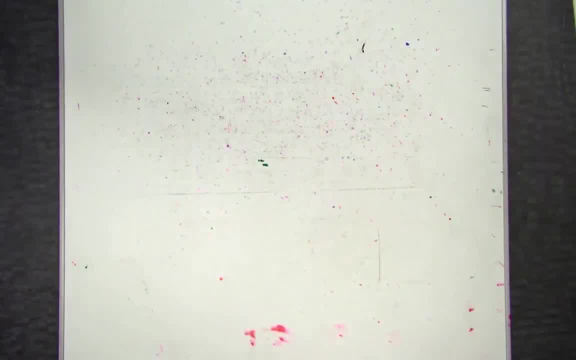 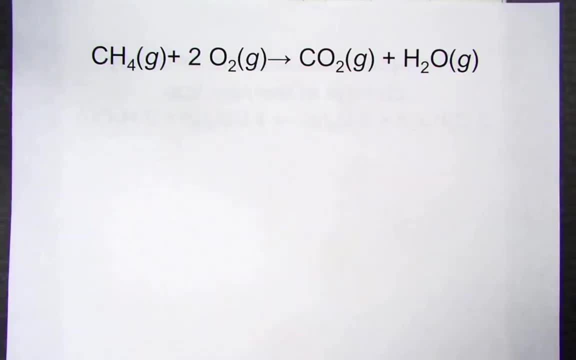 N is the coefficient in front of each product or reactant. So using our standard heats of formation, we're able to calculate a little easier than using Hess's law. Let's model with this example on slide 41.. Methane gas plus oxygen gas. 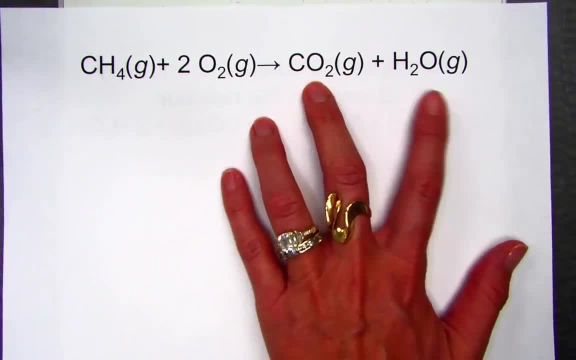 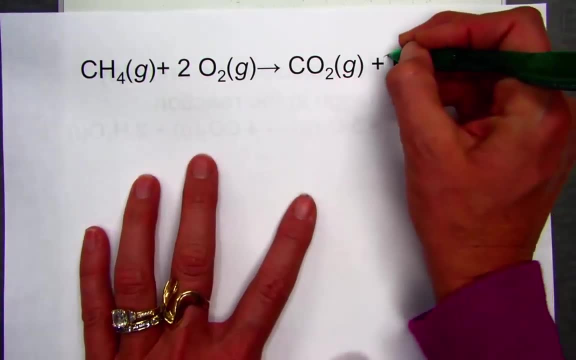 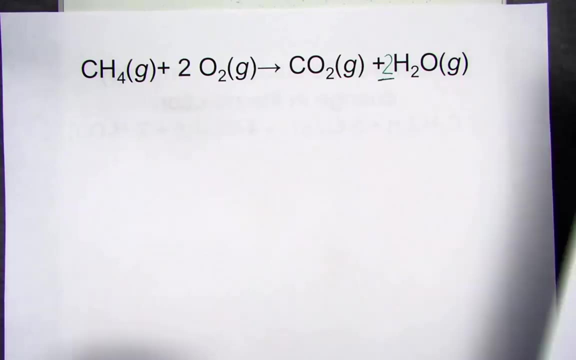 this is a combustion pattern: produce carbon dioxide gas and water gas. This is a balanced equation with a one to two to one to two equation. We need to repair that coefficient. Let's go to work and see if my PowerPoint slide has enough or if I have to pull out. 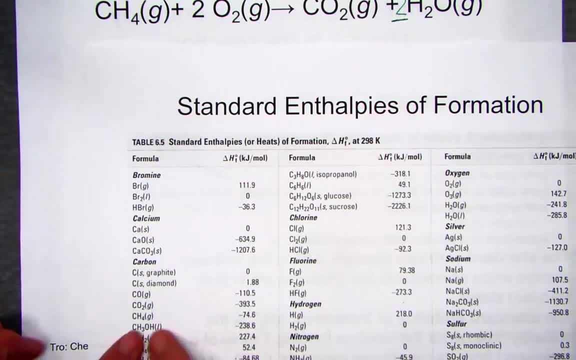 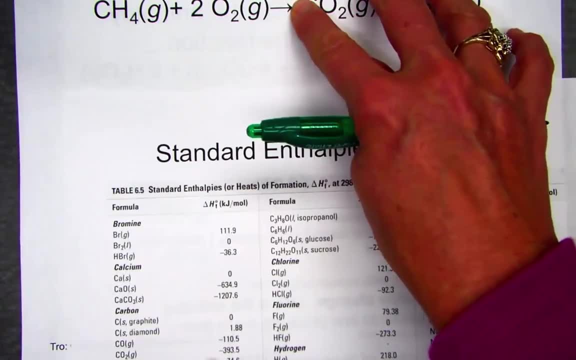 the back of our chemistry book. Methane is CH4 as a gas. I go to work and I find its value and I'm just going to write it for now. right underneath the equation I'm going to write negative 74.6,. 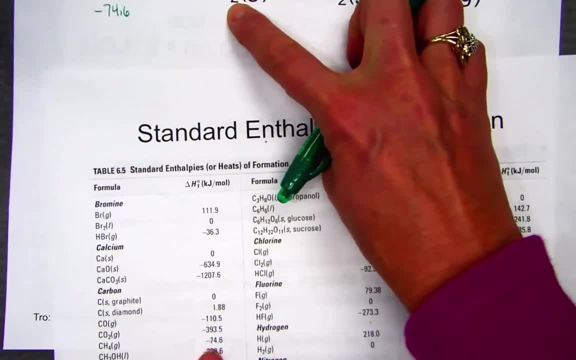 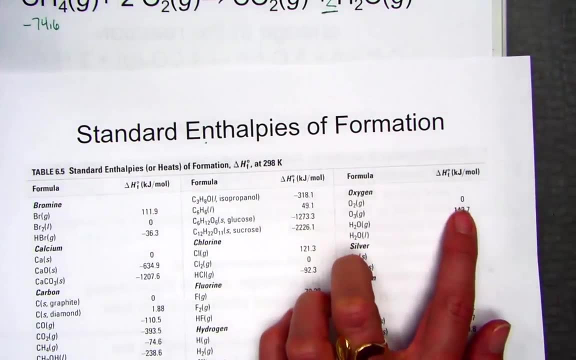 and that's in a kilojoule Diatomic molecular oxygen oxygen is zero, Again just showing that we know oxygen in its natural state- here it is- is zero O2 gas. And again I would distribute the two. 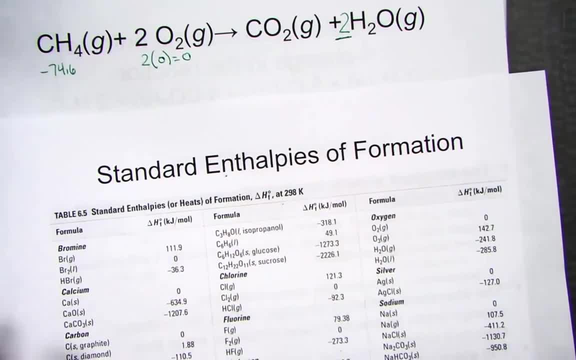 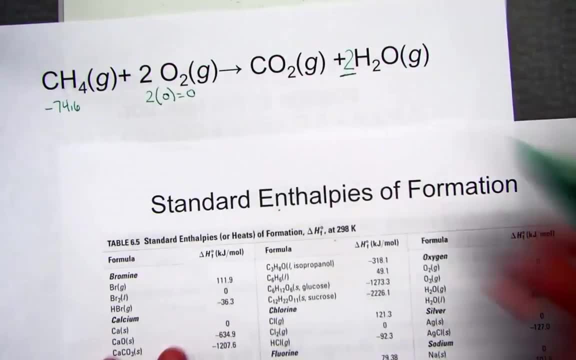 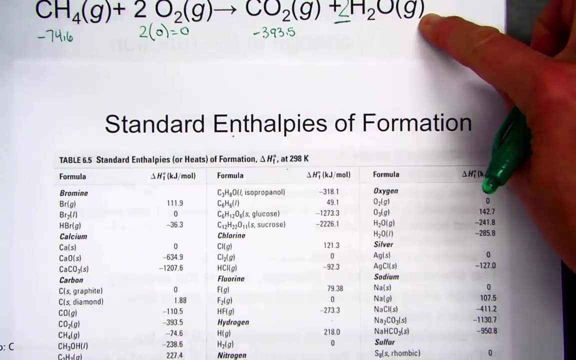 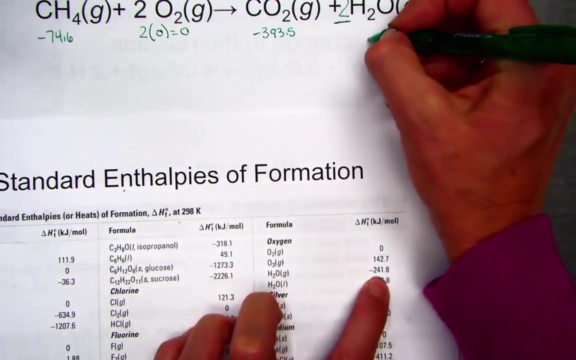 Two times zero is still zero. Carbon dioxide gas going to our chart: CO2 gas negative: 393.5.. And how about water gas? H2O And water is listed under the oxygen Water as a gas negative: 241.8,. 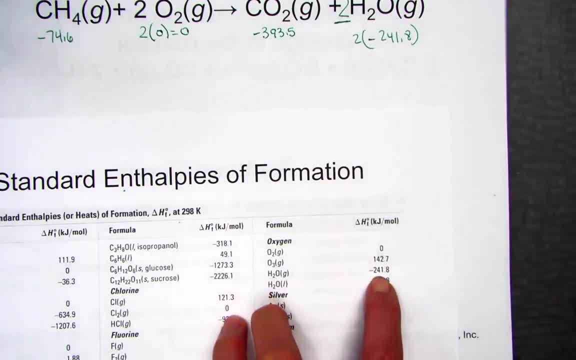 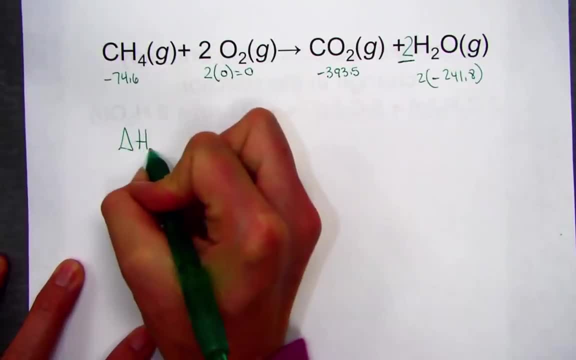 but I have to distribute the two through that, All right. so coefficient times the number from our chart. Simply stated, if I want to calculate the heat of this reaction, it's the sum, and I'm not very good at drawing those sigmas. 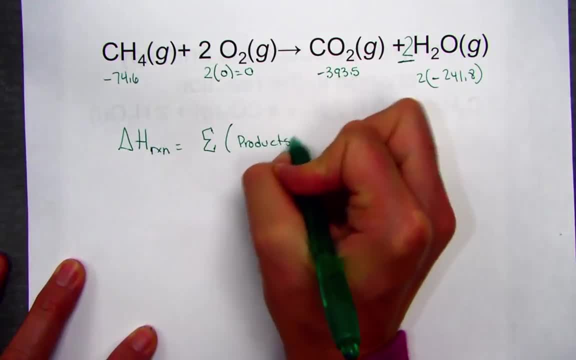 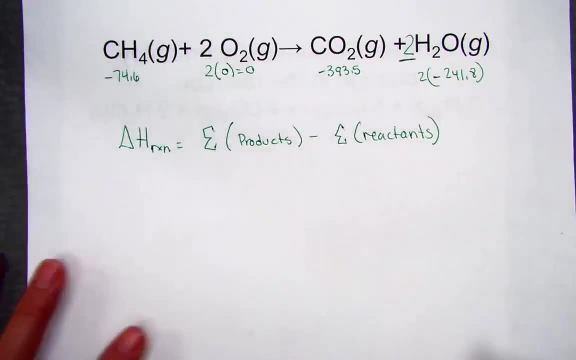 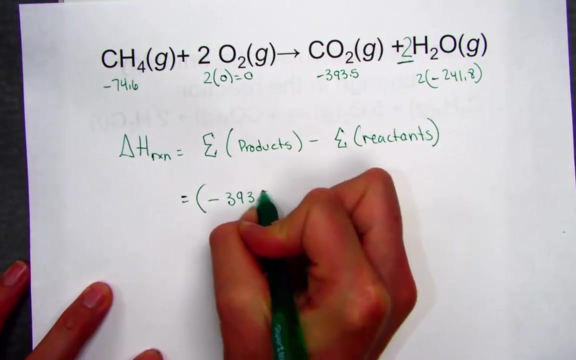 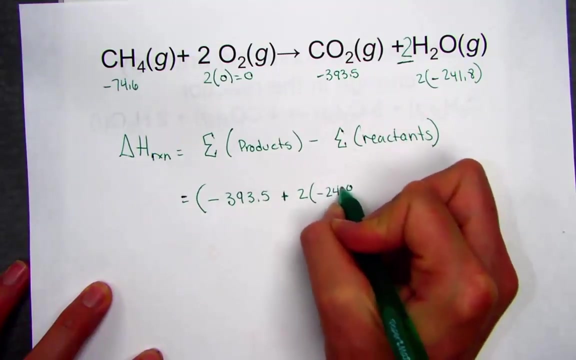 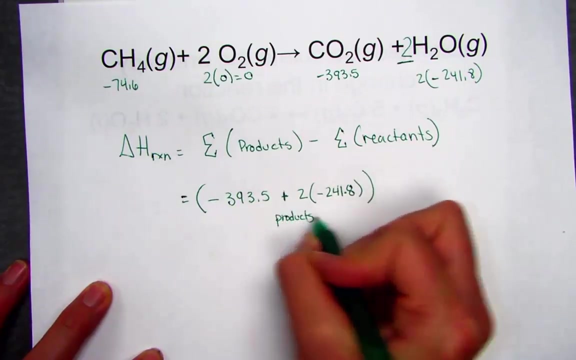 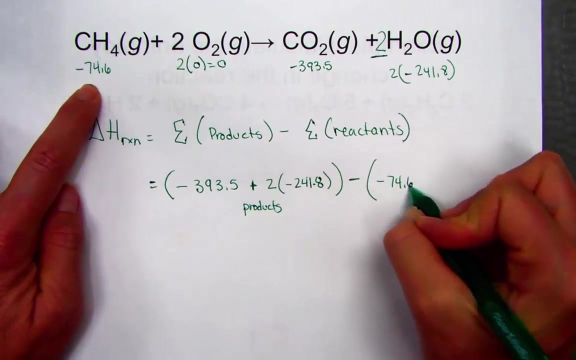 the sum of the products minus reactants. So products first. I'm going to take negative 393.5 plus two times negative 241.8.. The sum of the products minus the sum of the reactants: Negative: 74.6 plus zero. 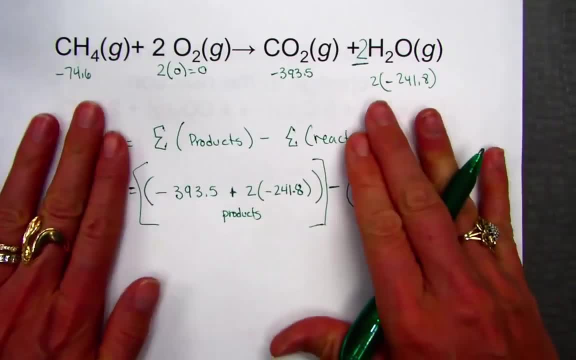 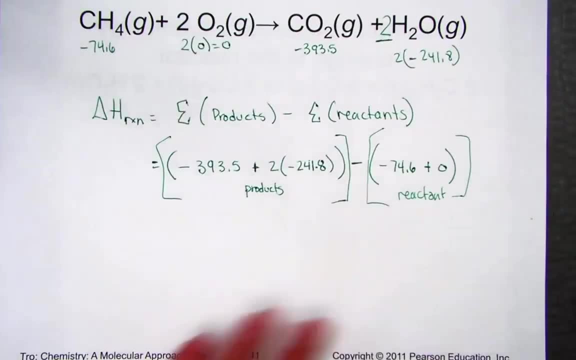 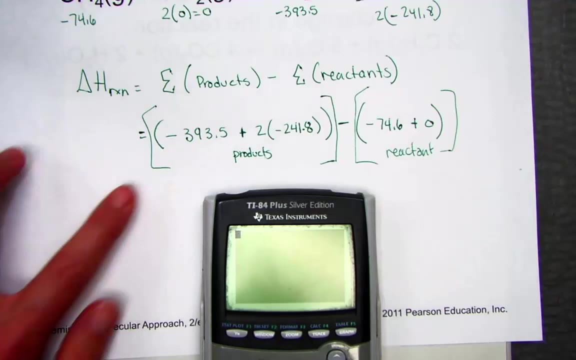 So here's what we have just to kind of clarify. First big bracket is product minus reactant. Let's hit on our calculator and see if we can get a common answer. All right. so first set of parentheses looks on Negative 393.5.. 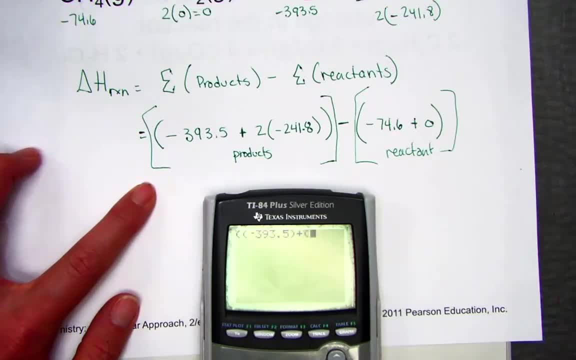 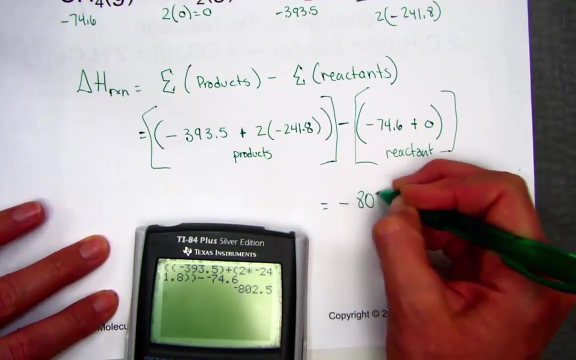 Plus two times negative, 241.8.. Close your parentheses out. Minus negative 74.6 equals- and I found the heat of this reaction to be negative 802.5 kilojoules of heat. These problems simply have us take time. 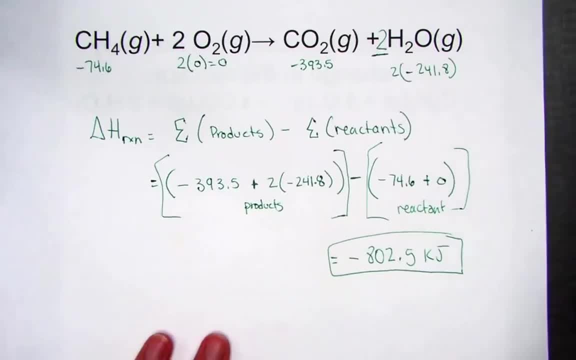 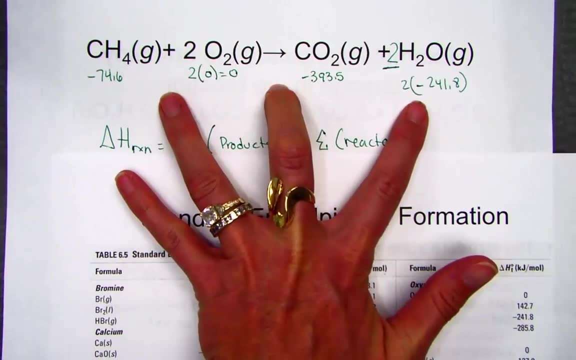 with the standard Enthalpiza formation chart, either using your appendix or the slide from the PowerPoint, finding the values, and I just record them underneath just to help me tabulate. I have to distribute the coefficients through: I sum the products. 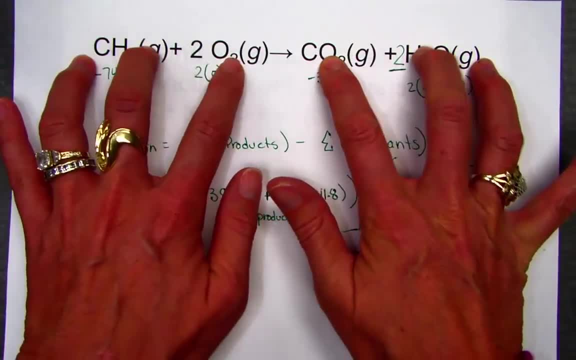 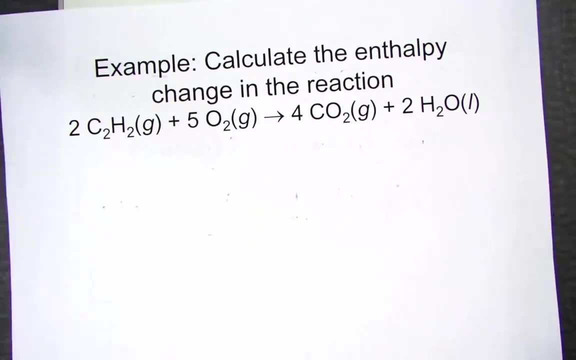 and I subtract the sum of the reactants- Products minus reactants- will pull out the kj- the heat of energy- for that reaction. Why don't you try one and see if we can reach a common answer, Pausing the video and working ahead? 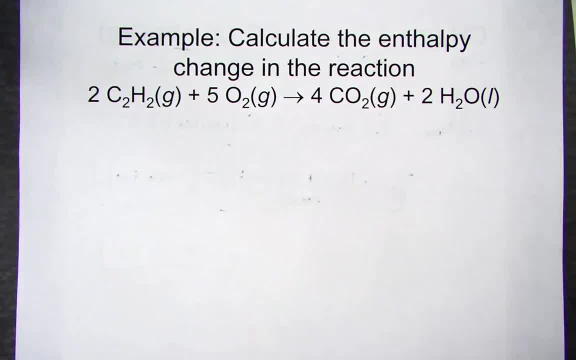 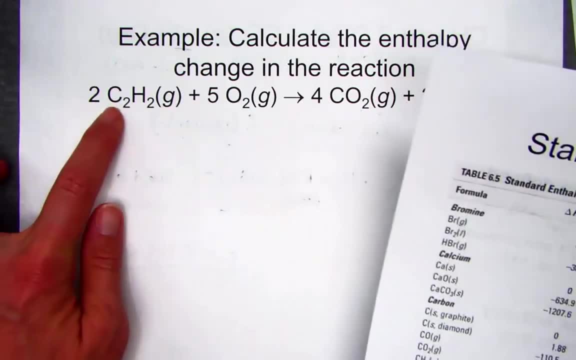 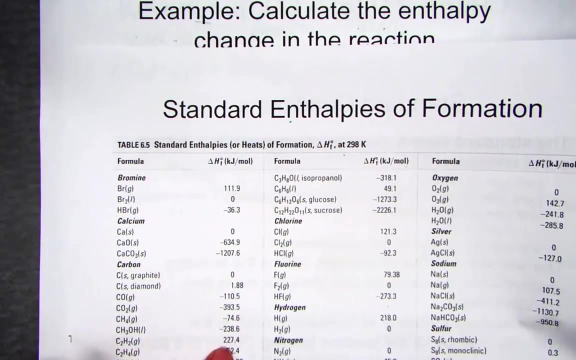 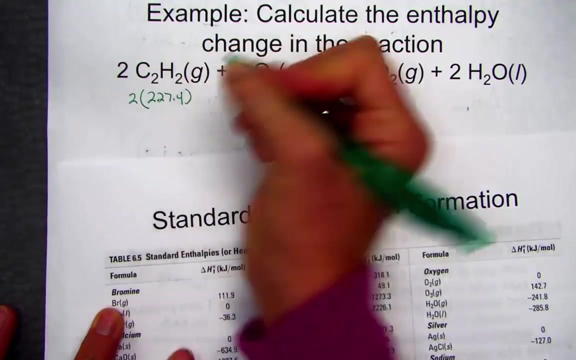 turning it back on when ready to check. Here we have C2H2 as a gas Again. I'm just going to use my chart and find C2H2 is positive 227.4.. 227.4.. I'll know I'll have to distribute through. 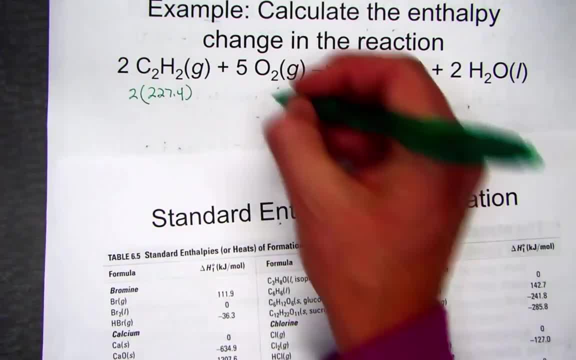 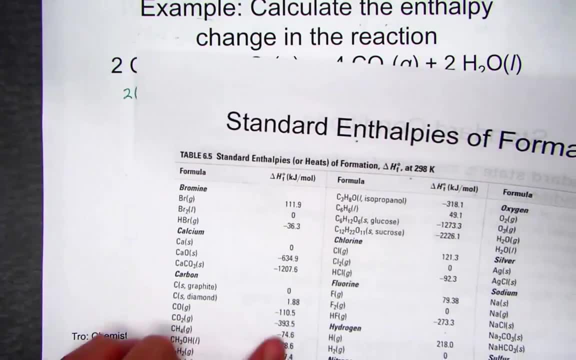 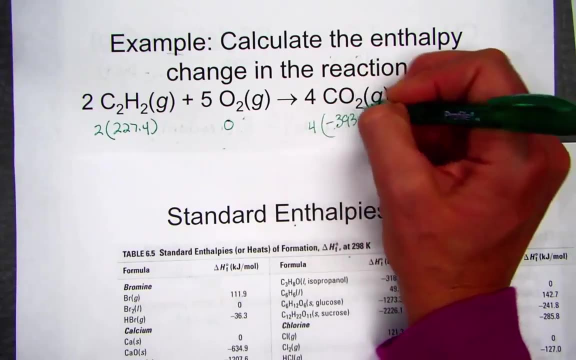 two times that value. It is a positive Oxygen again in its natural state, is zero Carbon dioxide gas. we looked up negative 393.5.. Remembering to distribute a four through that value from the coefficient, And now liquid water. 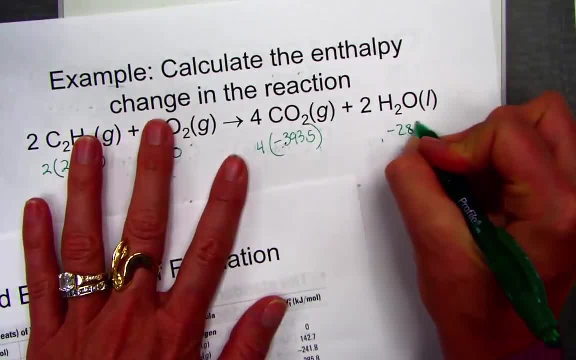 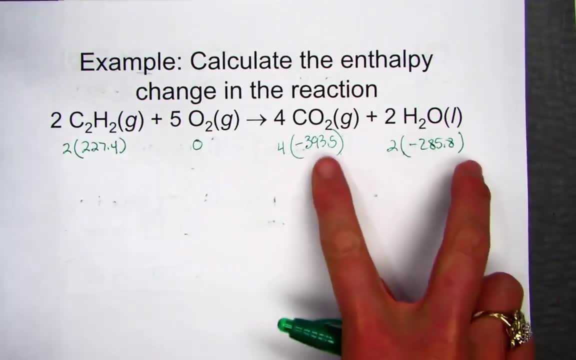 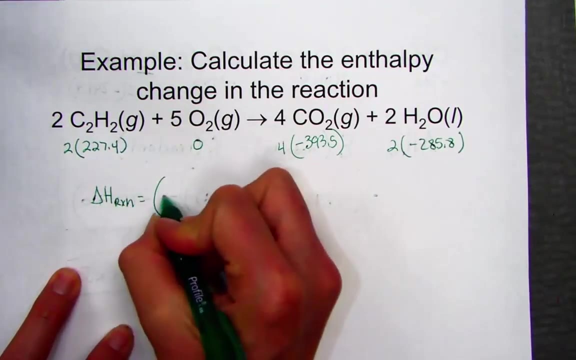 negative 285.8.. Distribute a two through that, The heat of this reaction is the sum of products minus reactants. So I'll just set up my math. The heat of the reaction is found by taking four times negative 393.5. 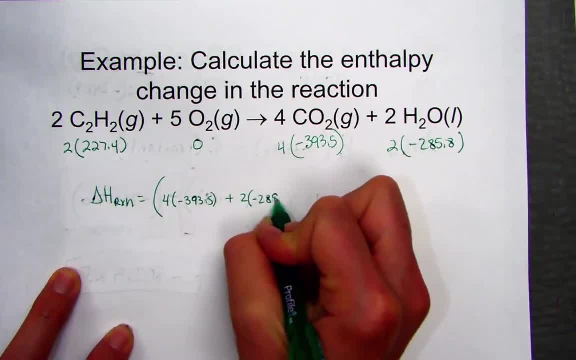 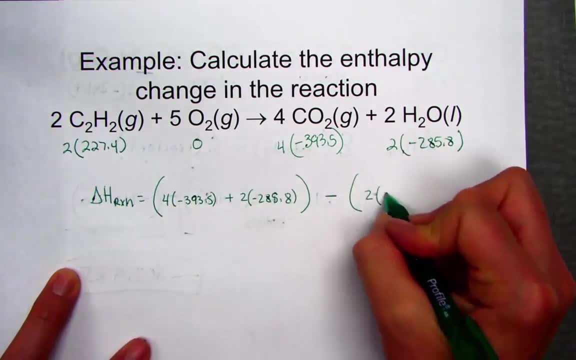 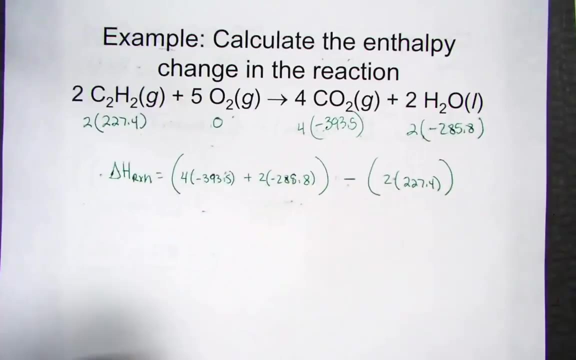 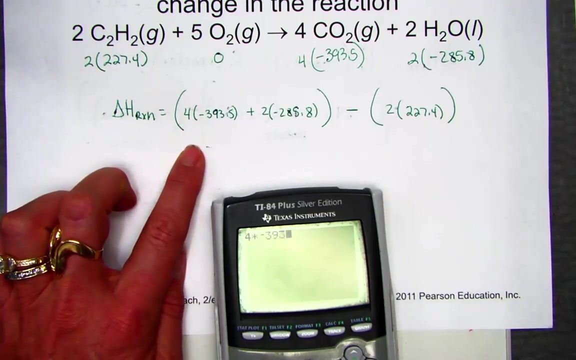 plus two times negative: 285.8.. The sum of the products minus two: 227.4.. And there's the sum of the reactants: Products minus reactants. Let's hit together and see what we find. We have: four times negative: 393.5. 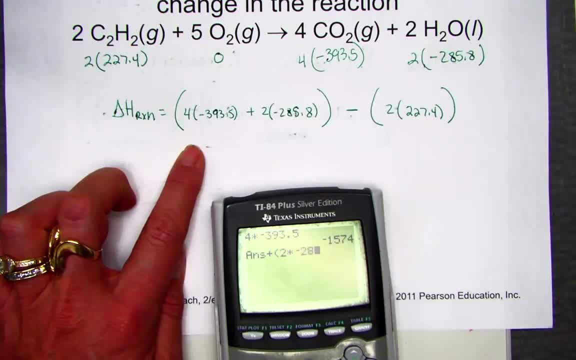 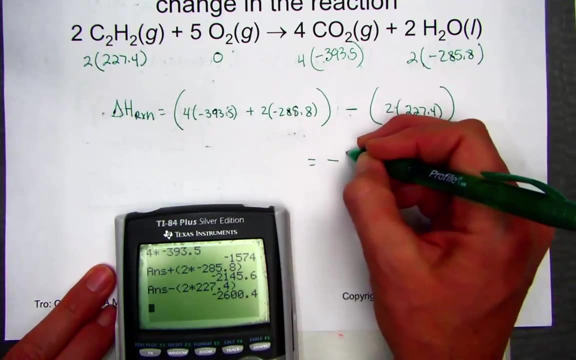 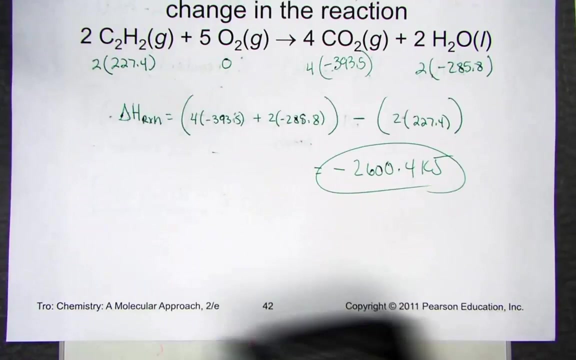 plus two times negative 285.8, minus two times 227.4.. We get a value of an exothermic negative 2600.4 kilojoules of heat Products, minus reactants. distributing the coefficients and simply taking some time to look through. 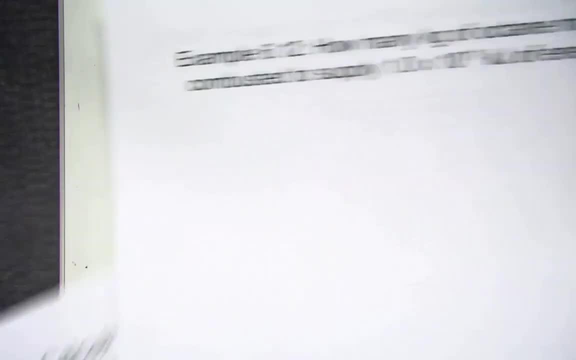 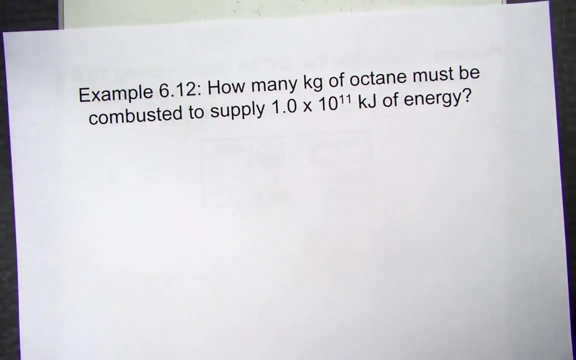 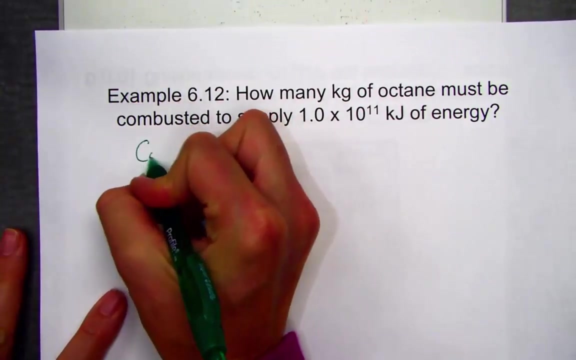 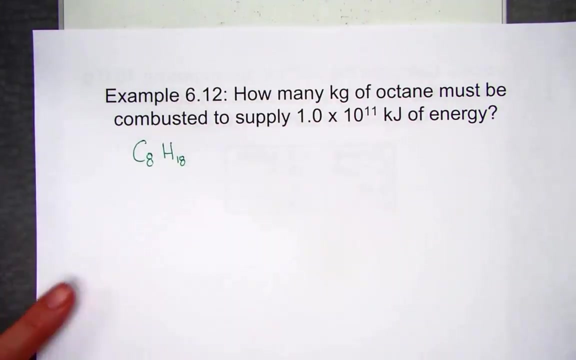 the standard enthalpy chart to find your equation: How many kilograms of octane? just on the right slide looks like it: How many kilograms of octane? C8H18, that's gasoline, must be combusted, so add oxygen. 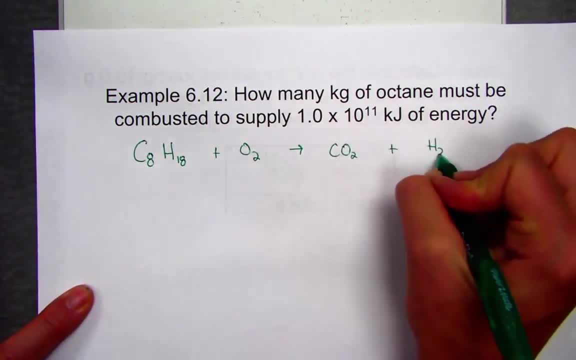 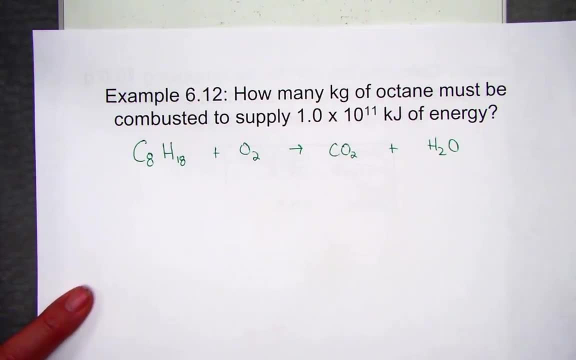 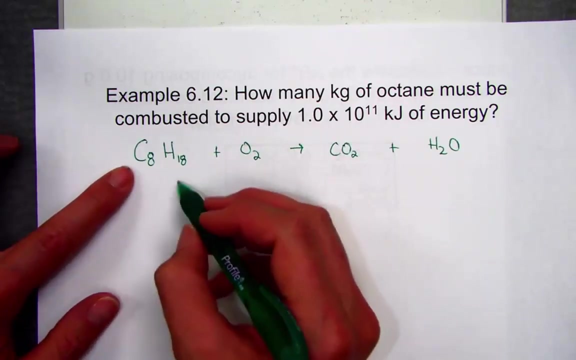 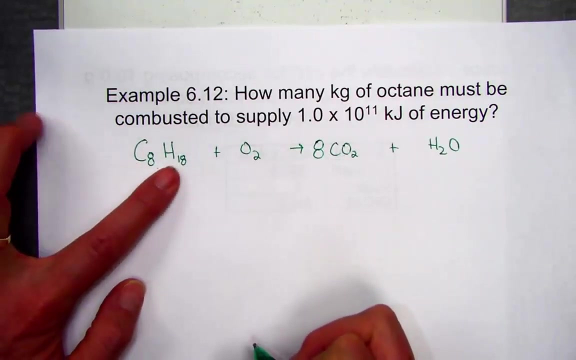 out comes carbon dioxide and water, to supply one times ten to the eleventh kilojoules of energy. Well, let's balance, as I'm counting in my head. Eight carbons, try an eight there. Eighteen hydrogen, so I'll try a nine here. 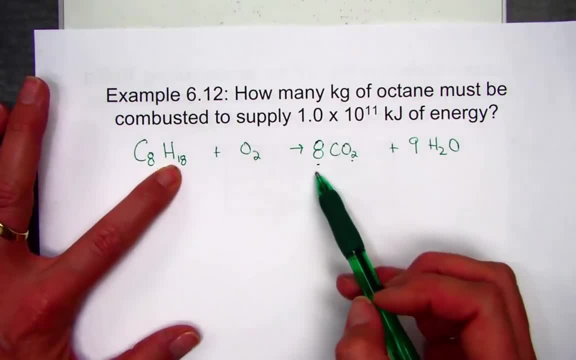 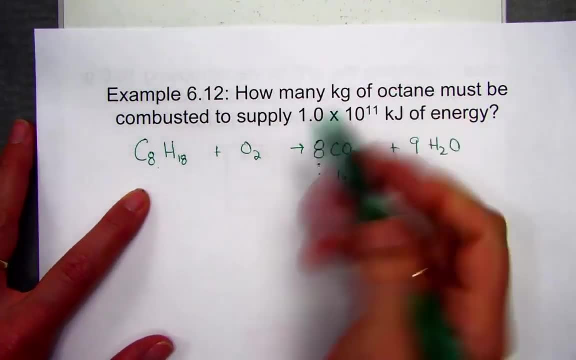 That's going to give me an odd number of oxygens, which is completely fine if we want to care. We have eight times two is sixteen plus nine is twenty-five. To put a whole number here wouldn't make sense because I can't get O2 to add to twenty-five. 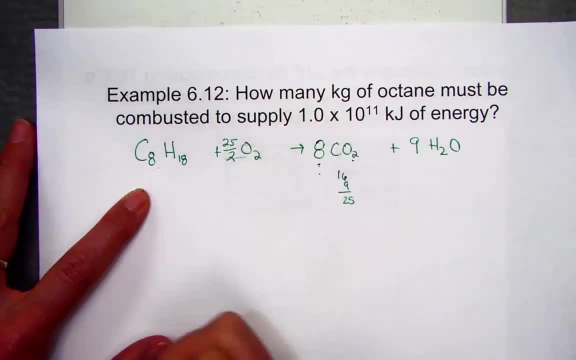 But I can do a little trick. It's twenty-five halves, And I don't mind doing that, because the heat of formation for oxygen is zero. Any number times zero is going to stay zero, And yet this still allows me to balance the equation. 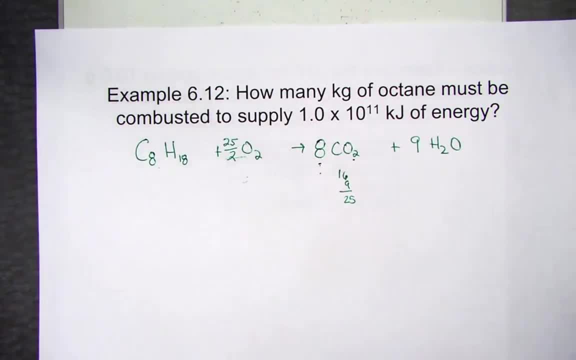 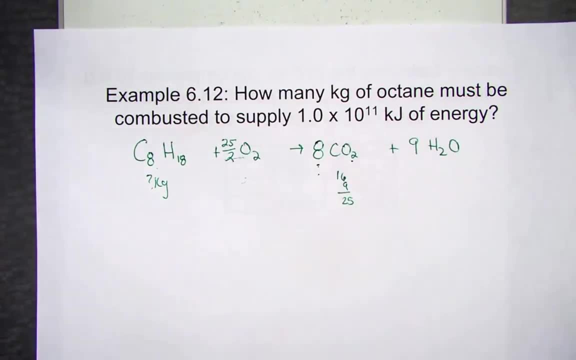 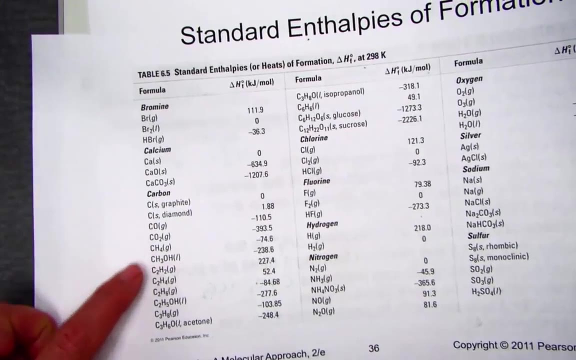 Alrighty. So how many kilograms of octane? I guess we're ultimately trying to solve for octane C8H18.. C8H18.. C8H18 isn't on our list, C8H18. But we can solve for it. 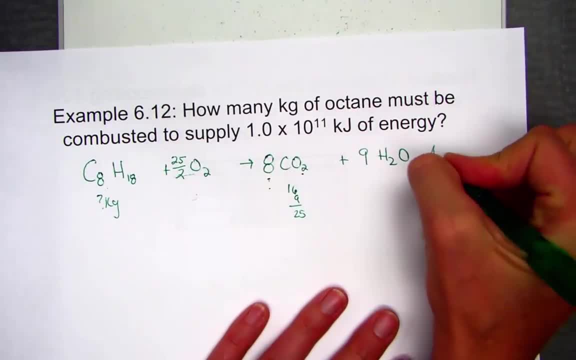 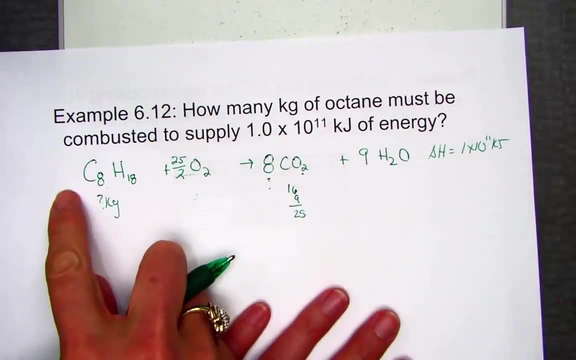 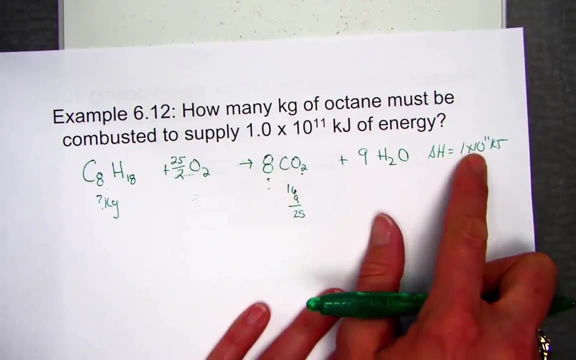 So suppose the delta H for this reaction is one times ten to the eleventh kilojoule, and that's for every one mole of octane. Alrighty, If this particular reaction per mole releases one times ten to the eleventh kJs. 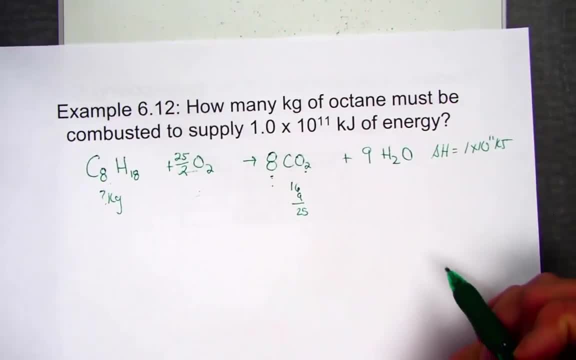 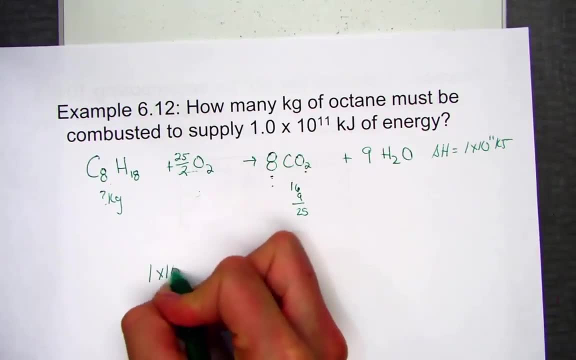 how many kilograms would be released. I look at this more as stoichiometry than really with the enthalpy chart. So if I know that one times ten to the eleventh kilojoules of heat are released, I don't really know that. 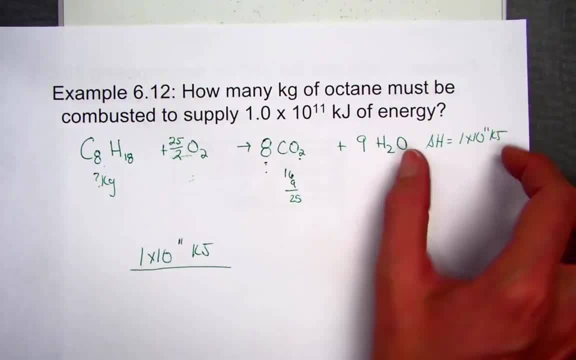 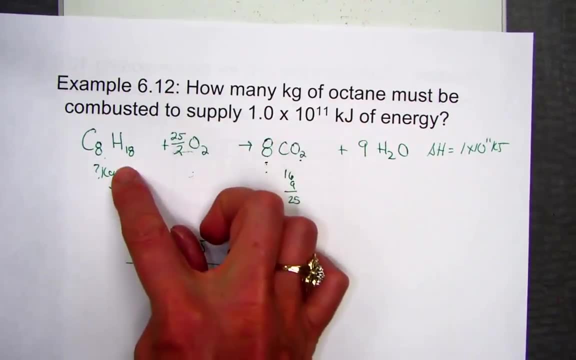 I'm going to pause. Let's think this through. What I don't know is that's the delta H, because it does not say that it's in kilojoules of heat. Alrighty, But what if I solved for this? 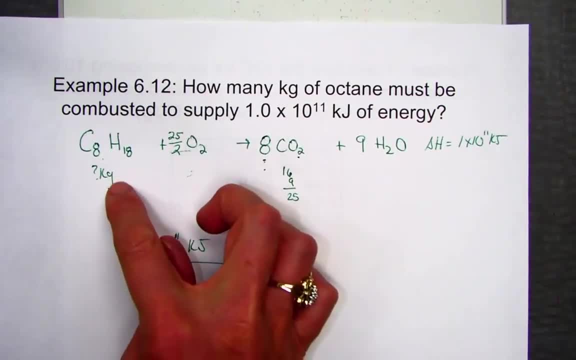 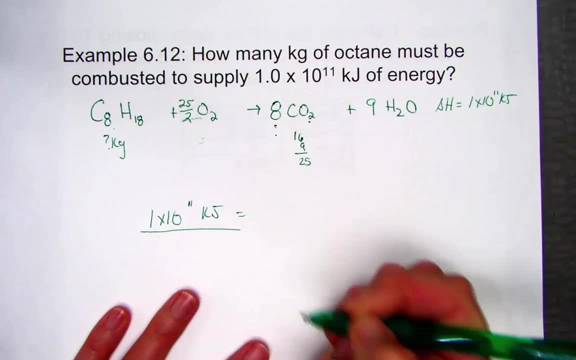 making this the target, I can find out how many moles or kilojoules of octane must be there If one times ten to the eleventh is the heat of the reaction, the sum of the products minus reactants, where I can target the octane. 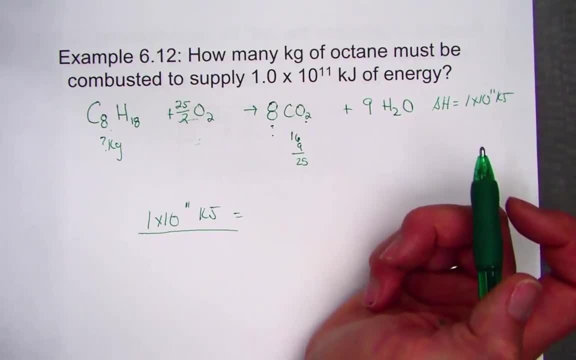 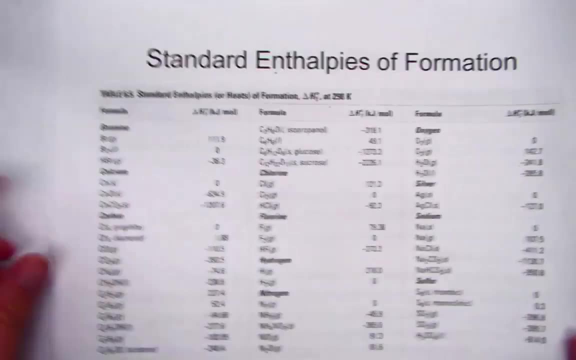 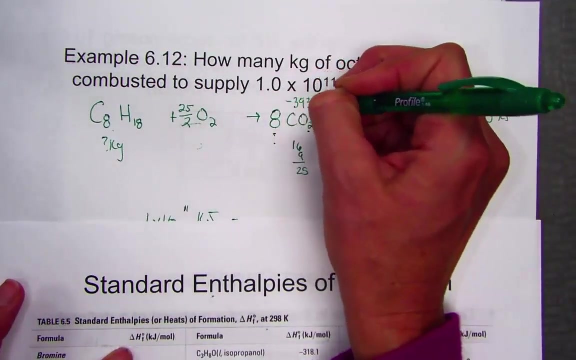 which would tell me its heat per mole and I can turn that into kilograms with a little mole map. So let's go to work. Carbon dioxide: looking up CO2 as a gas, negative 393.5.. And again, a combustion. 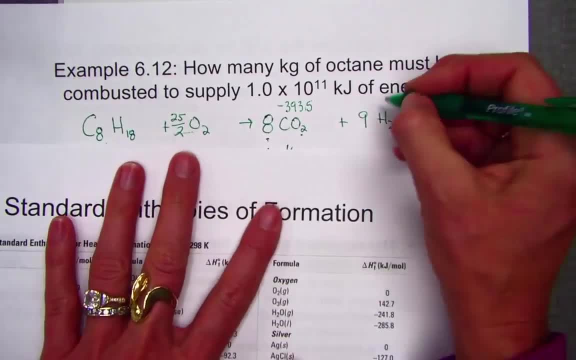 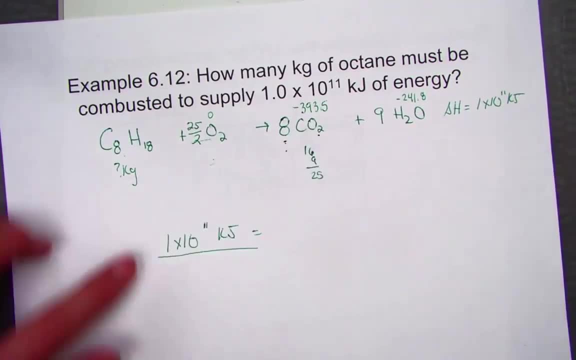 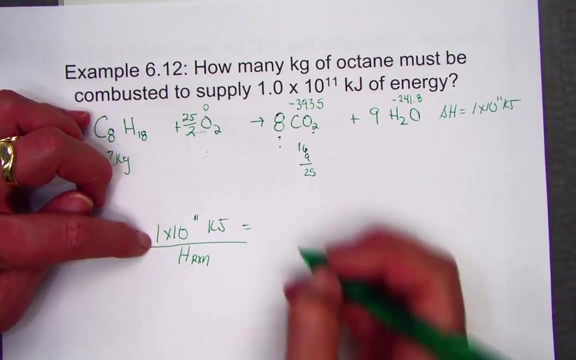 water will come out as a vapor. I'll use negative 241.8.. Oxygen's heat of formation in its natural state is zero. So if this is the whole heat of reaction, that's our target, one times ten to the negative eleventh KJs. 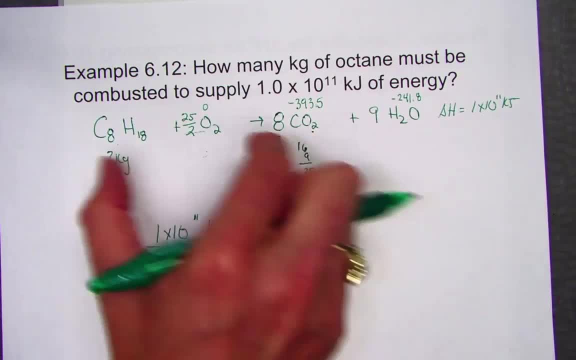 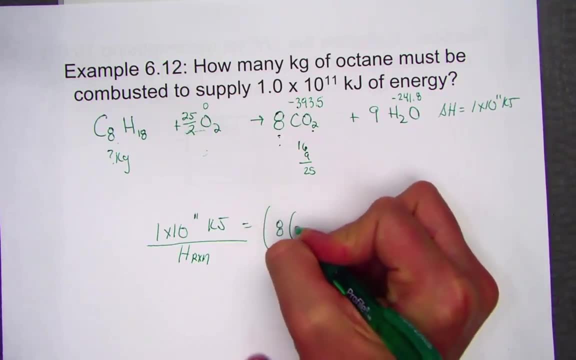 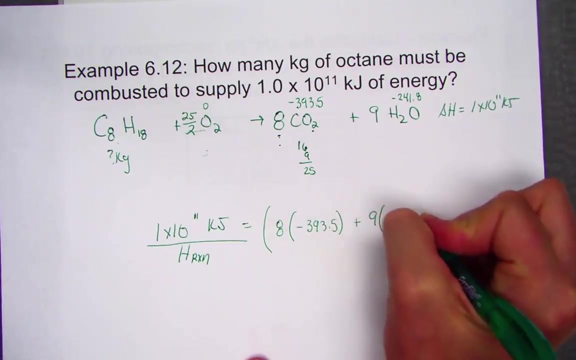 and that was found by taking the sum of the products minus reactants. let's make the octane the target, All right, So we'll have to distribute the coefficients eight times negative- 393.5- plus nine times negative- 241.8.. 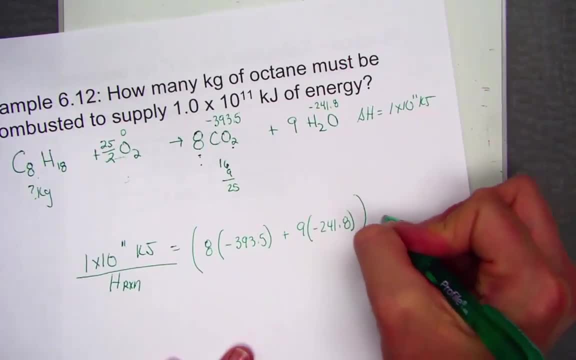 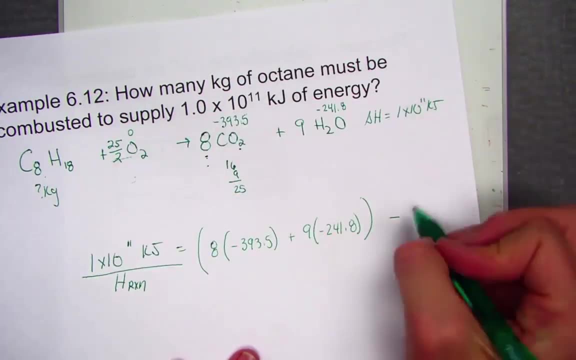 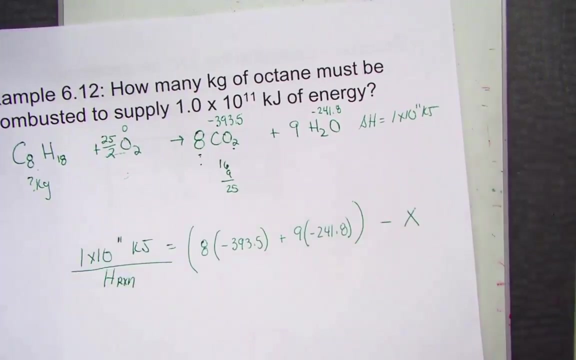 This is the sum of the products minus the sum of the reactants, which we're just going to call X, the heat that's released from this combustion X And just solve for that and we'll look at and call that good. 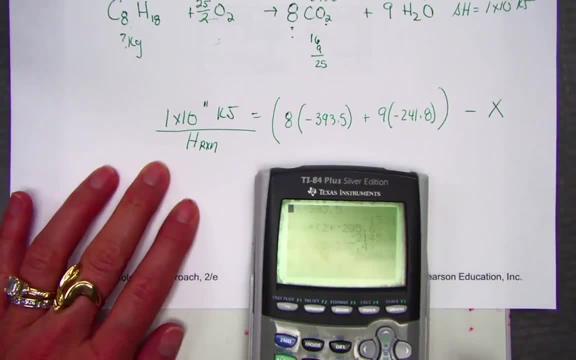 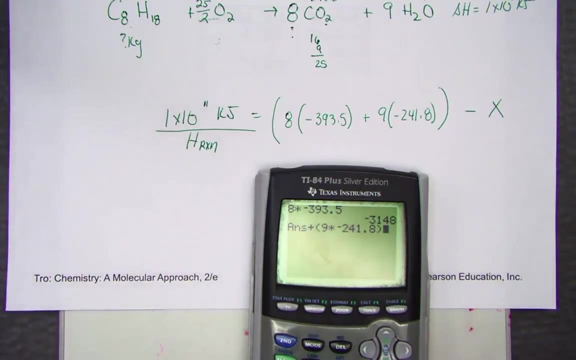 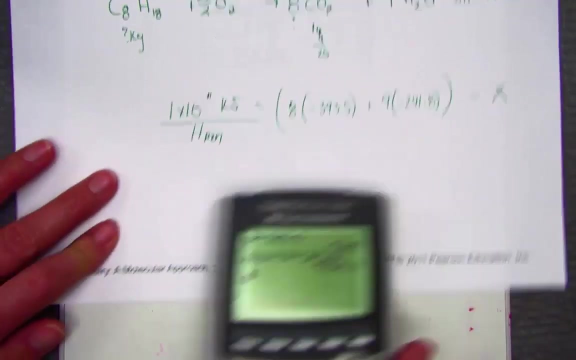 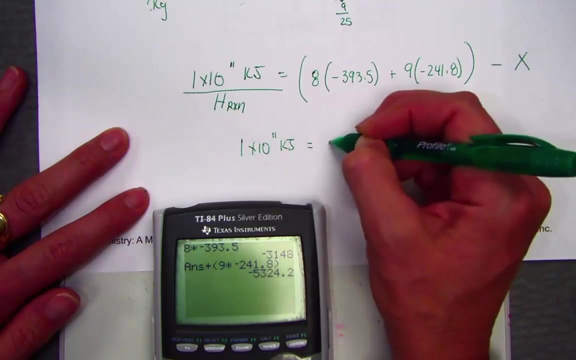 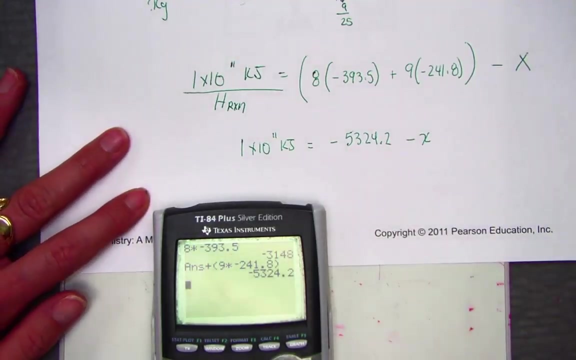 So, all right, let's do a little algebra: Eight times negative: 393.5, plus nine times negative: 241.8.. And here's what I have, and I'll just rewrite: One times ten to the eleventh, KJs equals negative 5324.2 minus X. 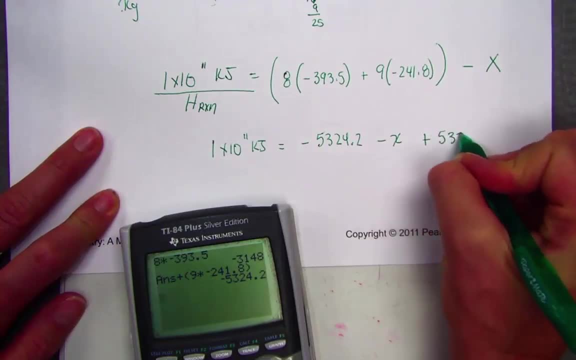 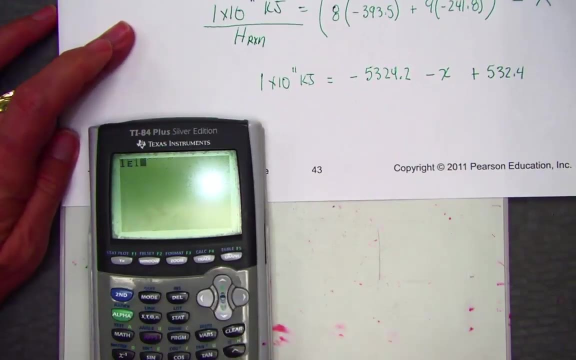 Let's add to both sides, to simplify, 5324.2.. And when we do that this will still be quite a large number. So one E11 plus 5324.4 is still going to be pretty near the same number. 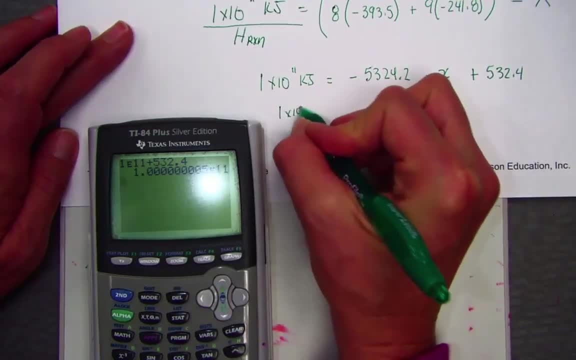 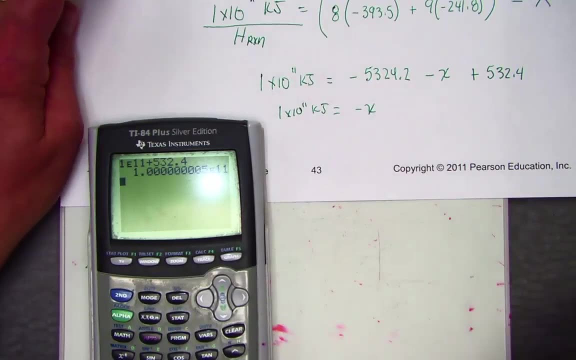 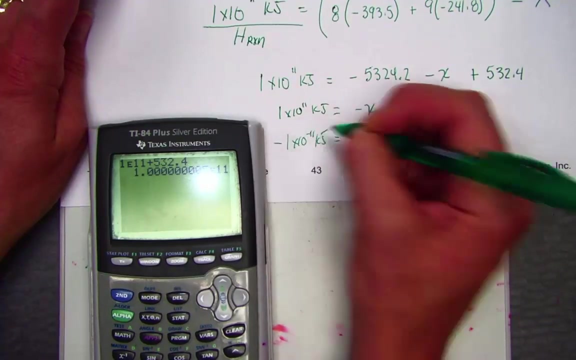 So I don't think I want to bother writing all those zeros down. It's so large it in essence stays the same value. But now I can see that that's what negative X is, And so X really is negative one times ten to the eleventh KJs. 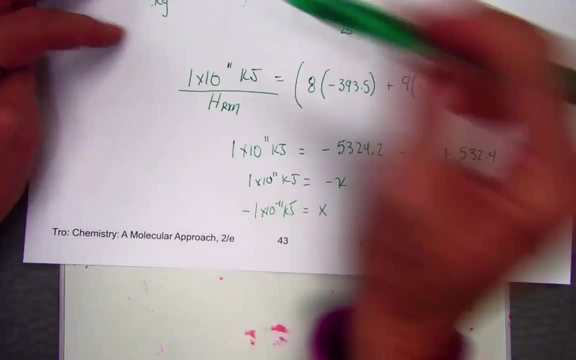 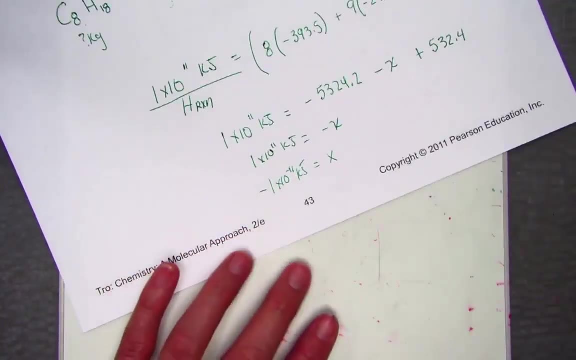 Now I've just verified that. indeed, that's the amount of heat that came out per mole of octane. It makes sense: Octane is gasoline. We burn it for fuel. A whole lot of heat energy is going to come out. And if that's per mole, 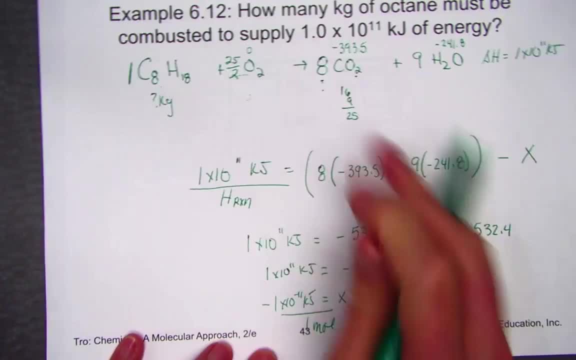 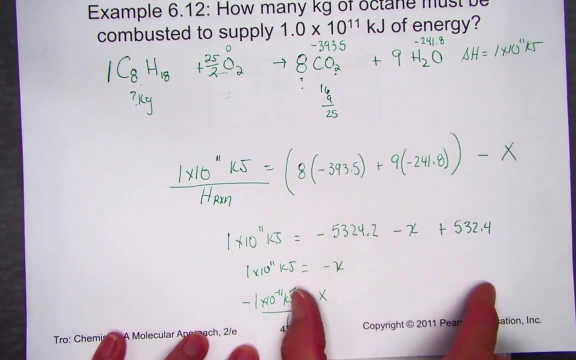 and that's what we let X stand for. if this was a one, we've just now calculated the energy per mole. I had that sense that that's what delta H was, but we just verified it mathematically that the carbon dioxide in the water 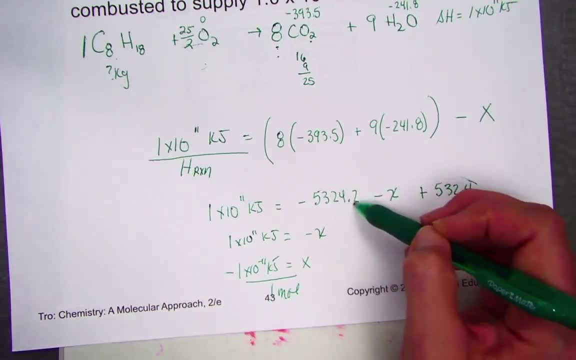 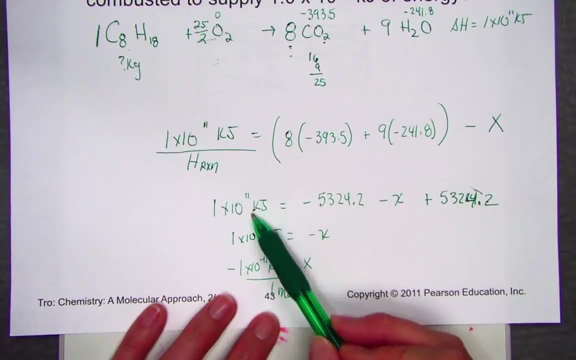 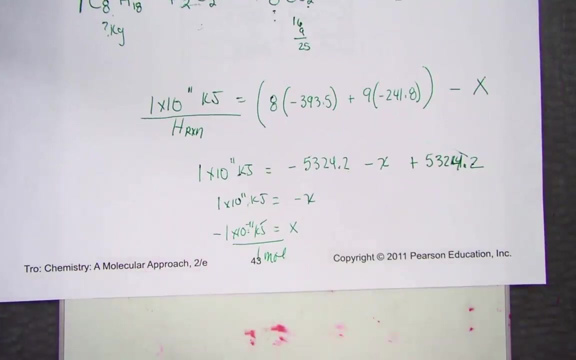 even though it really is 5324.2,, 5324.2,. when I add that to such a large number, it in essence stays the same number, And you could carry all those decimals and it really just wouldn't change the overall answer. 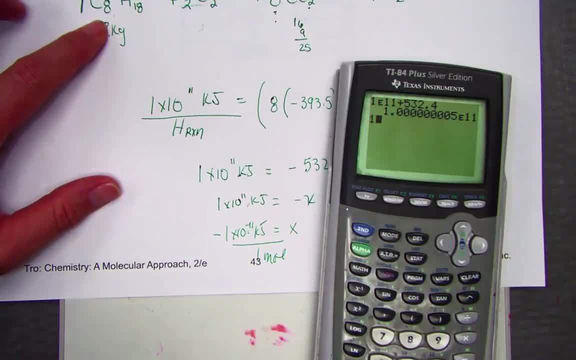 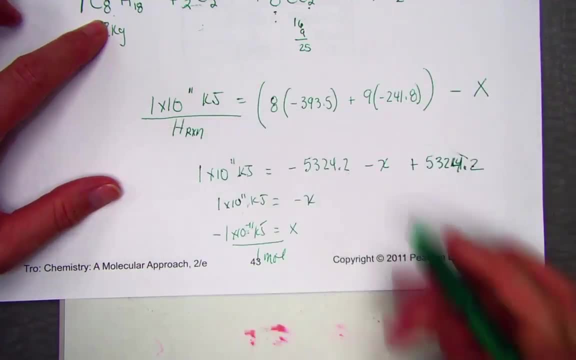 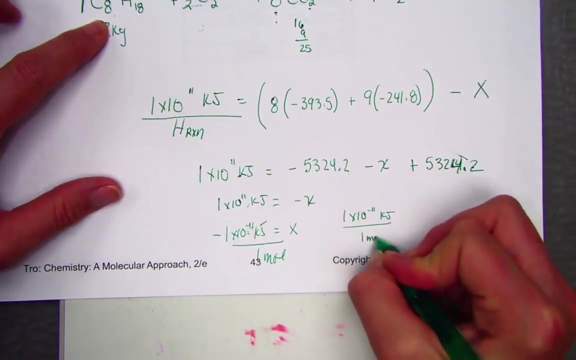 We have a little mole map work to do. Let's take 12 times 8 plus 18.. Finding the molar mass of octane is 114.. So one times ten to the negative eleventh KJs, and that's for every one mole. 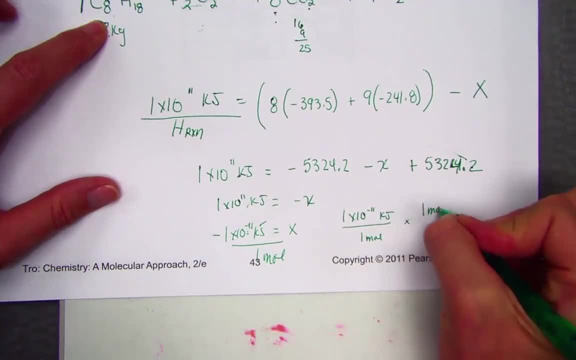 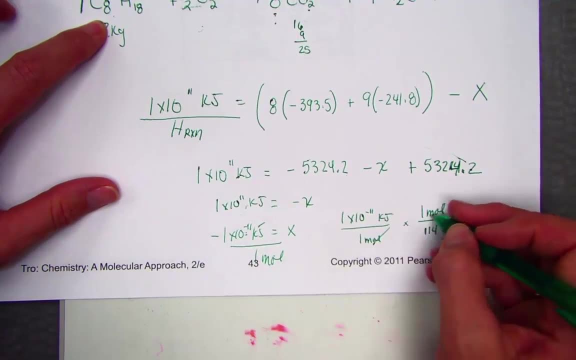 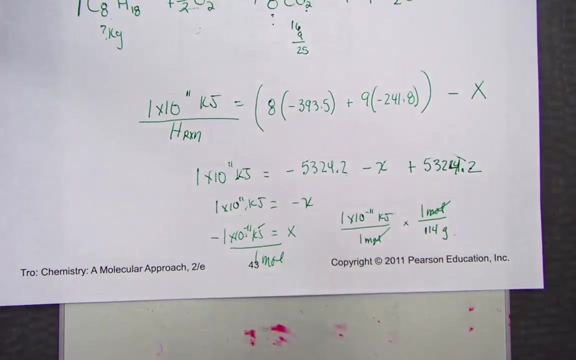 One mole would have a weight of 114 grams. Moles have canceled and we're going to get a KJ per gram and telling us how many grams we'd have to burn- And it will not be a large number- and we'll just ask you to flip to a KJ. 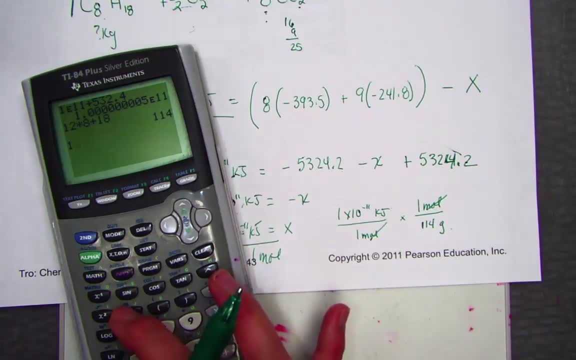 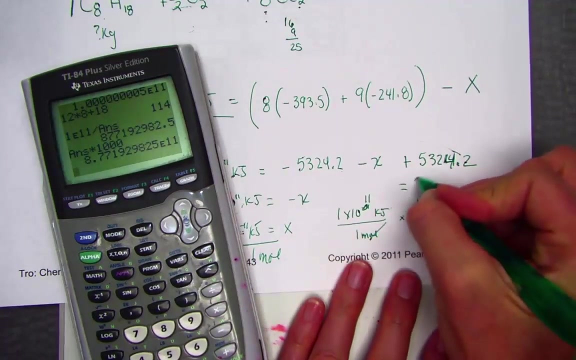 So 1E11.. That's not negative, it's positive 11.. Divided by that number- and I'll just go- times a thousand and it's still quite a bit: 8.77 times ten to the eleventh KJs of fuel. 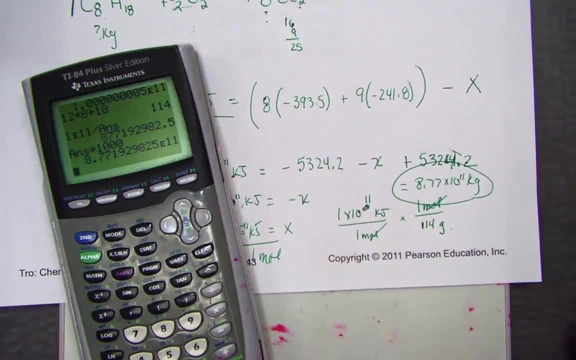 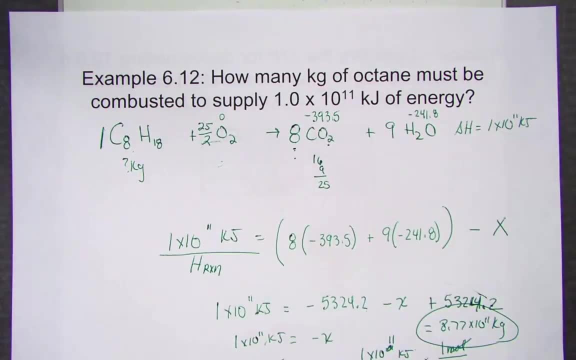 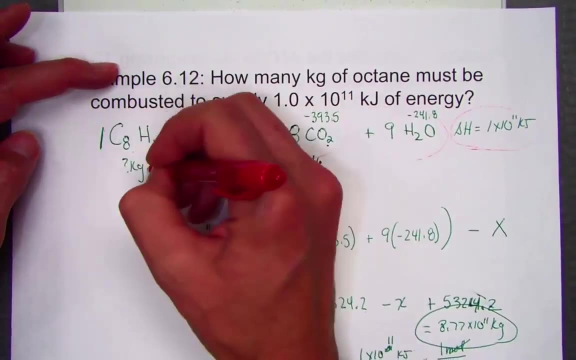 would combust to produce such a large amount of heat energy. I think the bigger story with this particular problem just kind of putting away such large numbers and thinking through this strategy- if we know the heat of reaction and we can look up all but one of the ingredients. 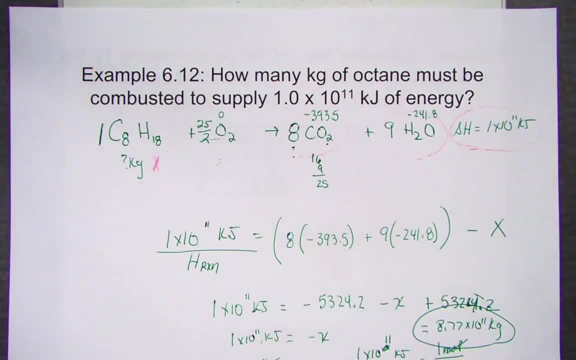 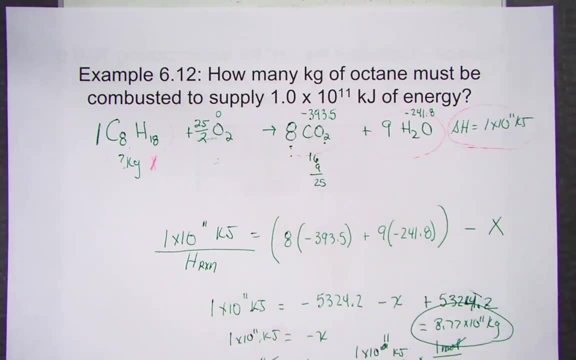 we can make that our target variable. In essence, that's all we've really done. The story problem: that probably wasn't the best because they chose such large numbers that the algebra kind of fell apart, Subtracting or adding such a tiny number to such a huge number. 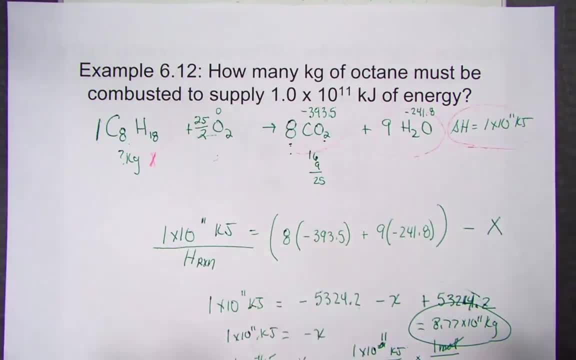 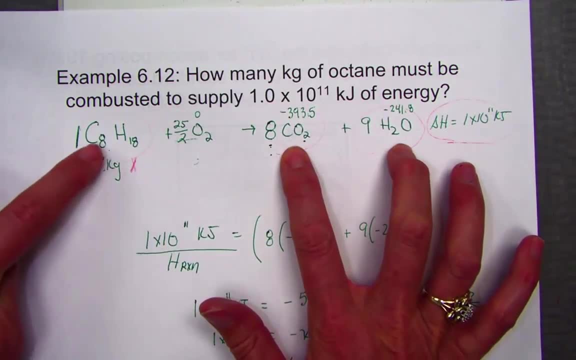 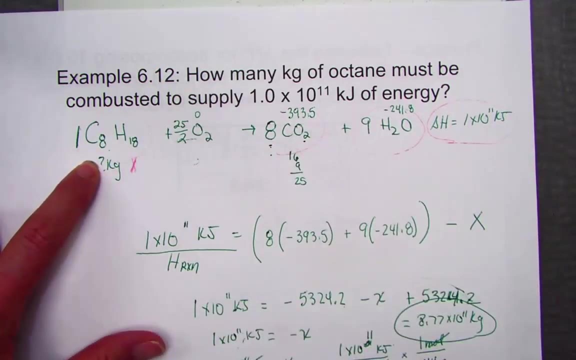 really didn't change it significantly. But just thinking about the strategy, we knew the delta H of reaction. we looked up the sum of the products and called the target variable X the amount of joules of heat energy per mole of C8H18.. 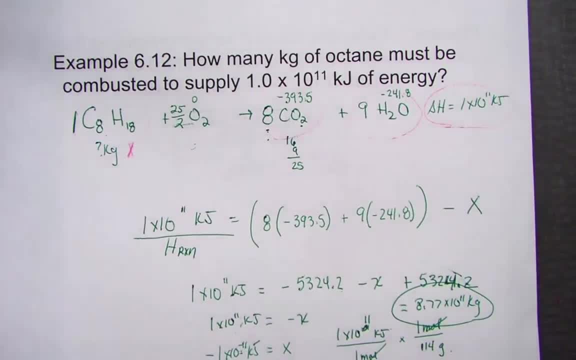 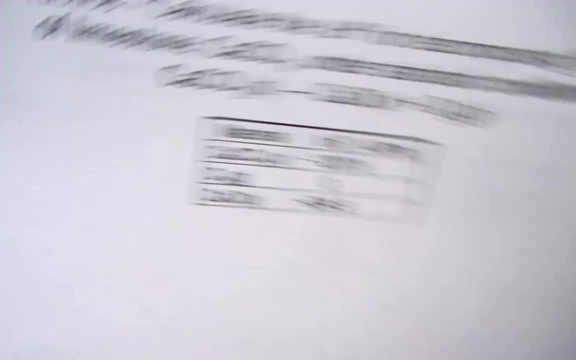 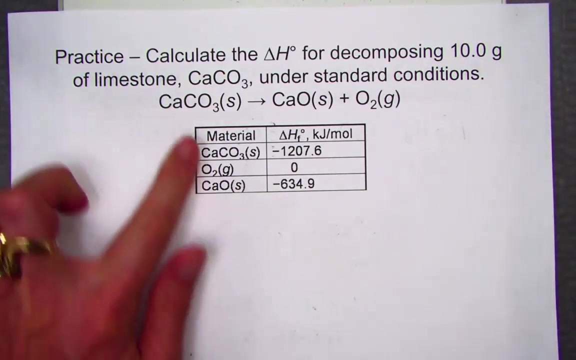 Once we solved for the heat energy per mole, we just simply flipped it to find how many kilograms by using a mole map problem. Let's take a look at one more: practicing delta H for a decomposition: When the decomposition of calcium carbonate under standard condition occurs. 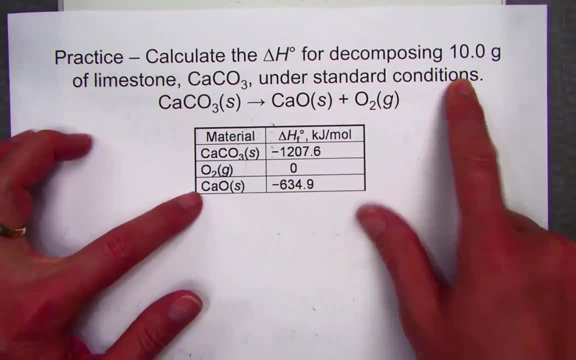 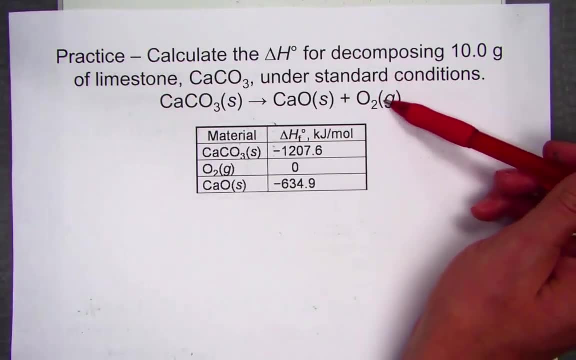 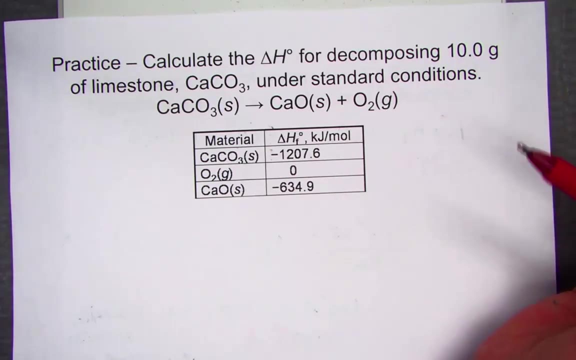 we have the following set of data: Calculate delta H for the reaction. Well, this one's pretty straightforward: The heat of reactants, CaCO3 is given, The products given. So they really have done the legwork. They've looked up, using their appendix, the values for us. 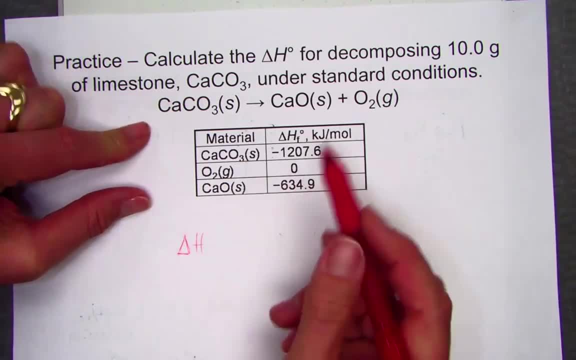 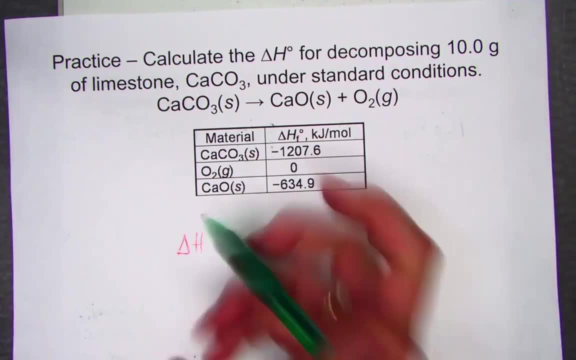 and all we're being asked to calculate is delta H. What that will come to is per mole, and we'll just have to find out for the mass of 10 grams. So let's find delta H By taking the sum of the products. 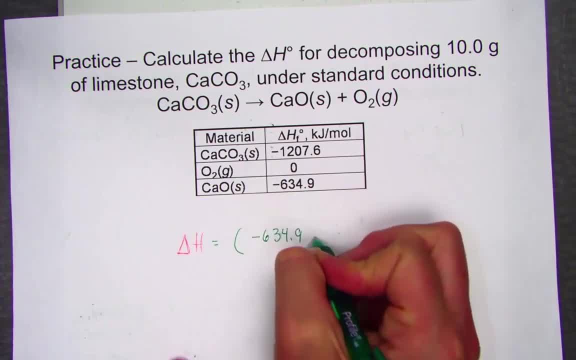 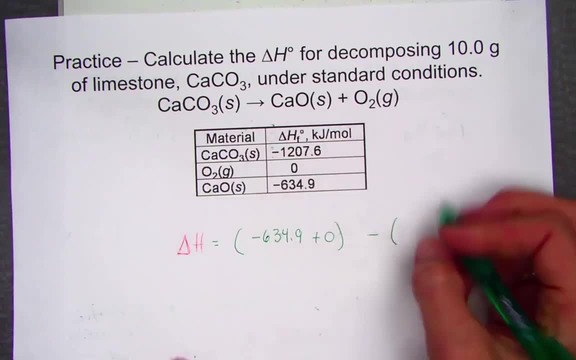 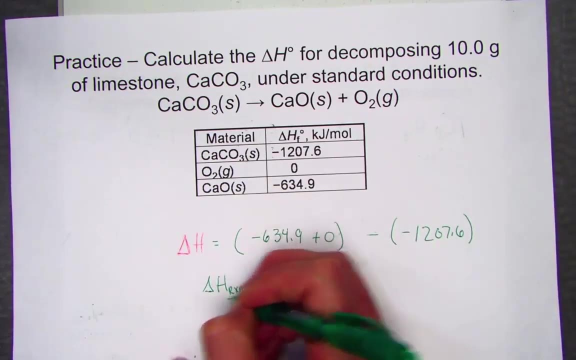 which would be negative: 634.9 plus 0, the two products minus the sum of the reactant, of which there's only one, which is negative: 1207.6.. We'll simplify this for the reaction and that comes out in per mole. 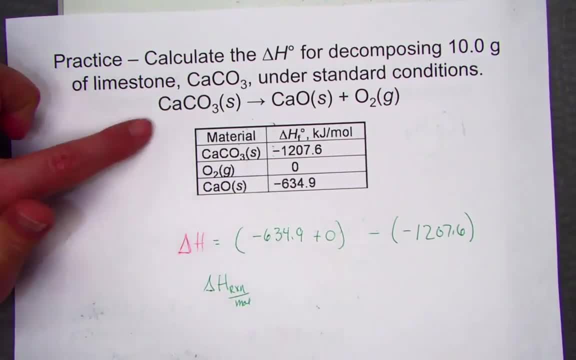 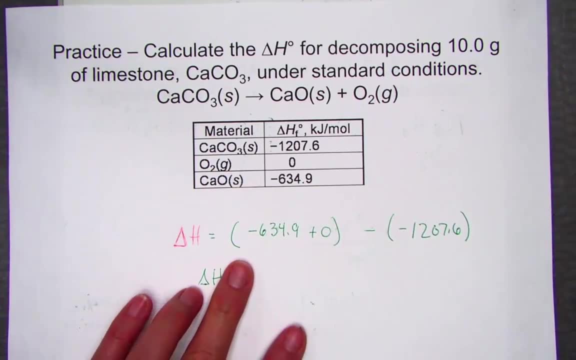 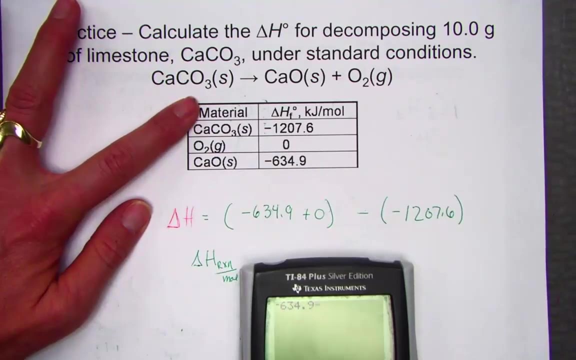 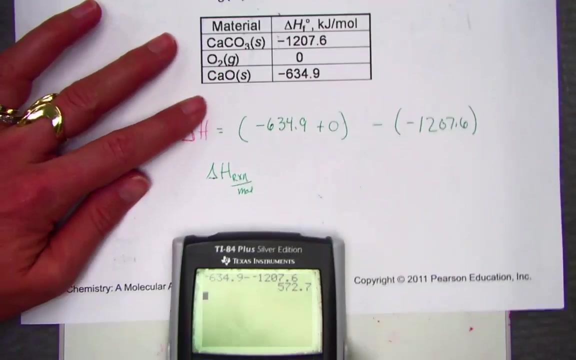 And notice, calcium carbonate is already written in a per mole basis. The coefficient is a 1.. So here's what we'll do. We'll take negative 634.9 plus 0, minus a negative 1207.6.. And that comes out to be a positive value of 572.7.. 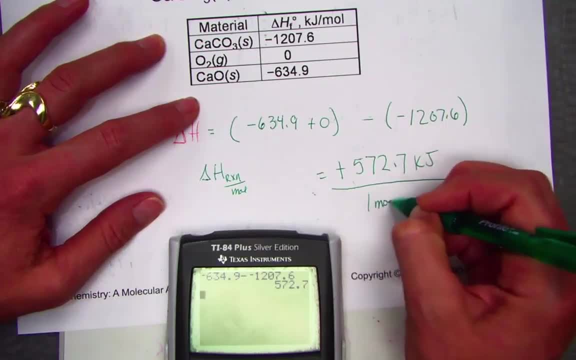 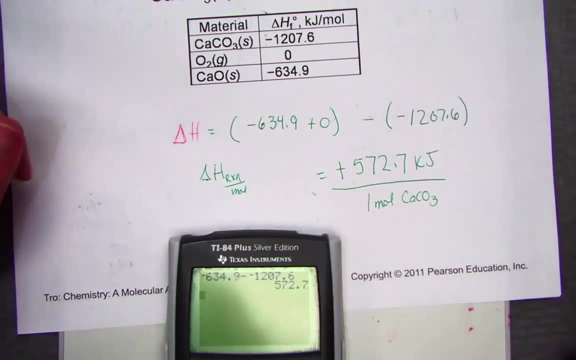 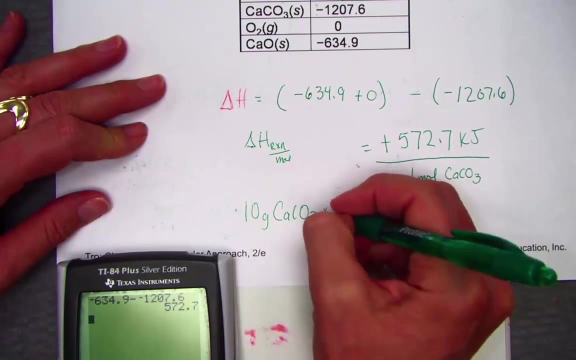 Think about that as just standing for kilojoules of every 1 mole of calcium carbonate. But we didn't have one whole mole, We had 10 grams. 10 grams of calcium carbonate can be converted to a mole by using a formula weight of CaCO3. 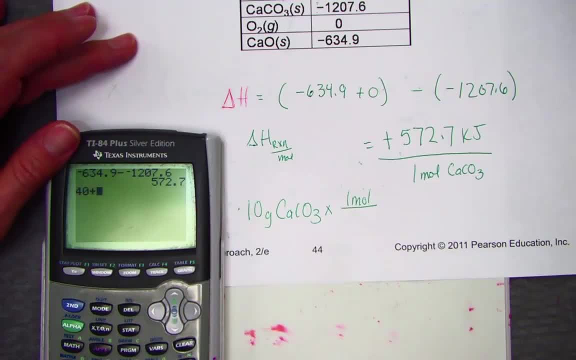 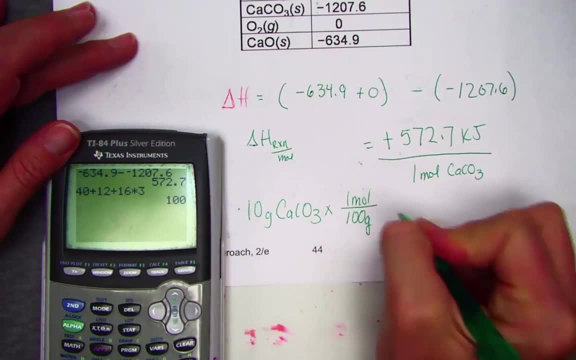 Calcium has a weight of 40, 12 on the carbon and 16 times 3 on the oxygen, and the molar mass here is 100 grams. So 10 grams is the same as saying 0.1 mole of calcium carbonate. 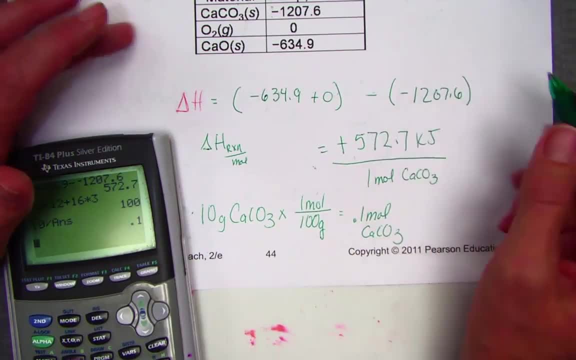 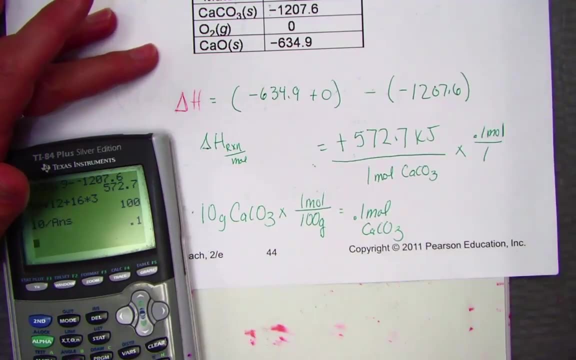 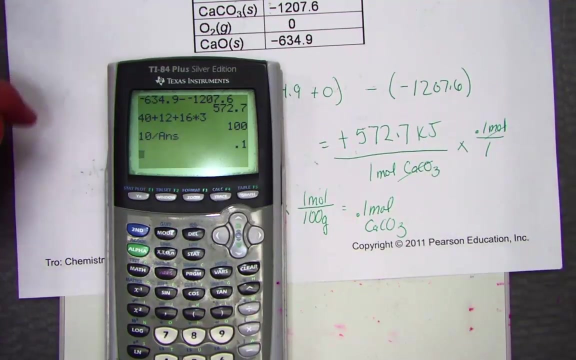 If 527, excuse me, 572.7 KJs were released for one whole mole, how many would have been released for 0.1?? Notice then how the moles cancel, and we've got it in kilojoules per 0.1 or 10 grams. 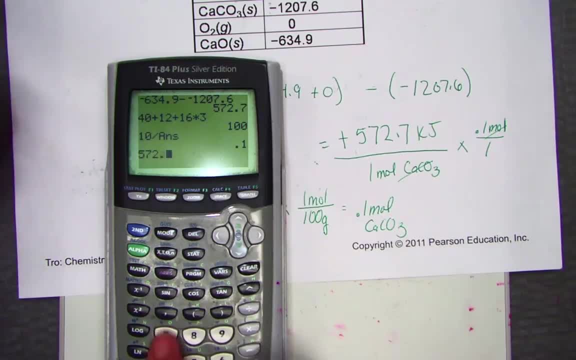 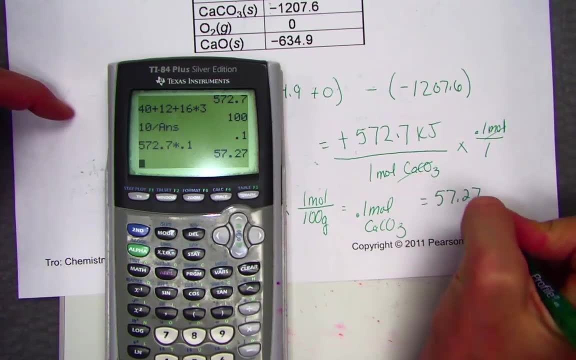 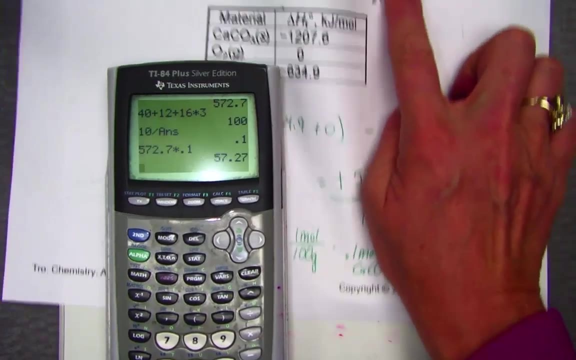 So all we have left to do is really slide. the decimal 572.7 times 0.1 is 57.27 positive units kilojoules of heat. energy Decomposition is an endothermic process. It takes energy to force limestone to decompose. 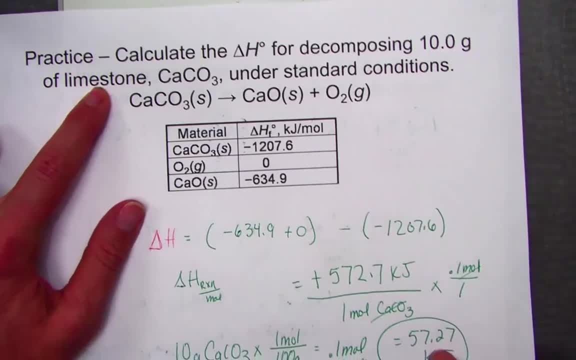 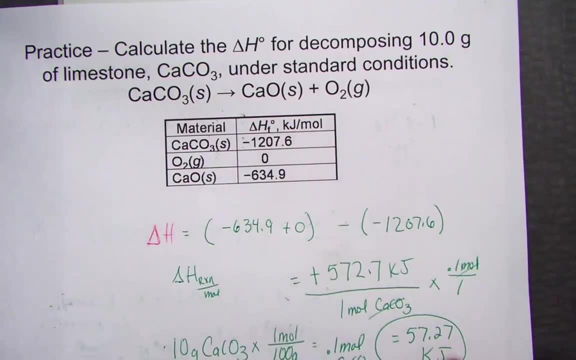 If I had 10 grams of limestone I would have to put in 57.27 kilojoules of heat energy to force its decomposition. Again, we solve for delta H. Notice it's for every 1 mole of the reactant. 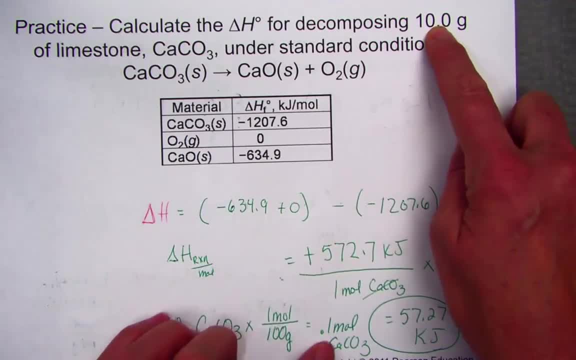 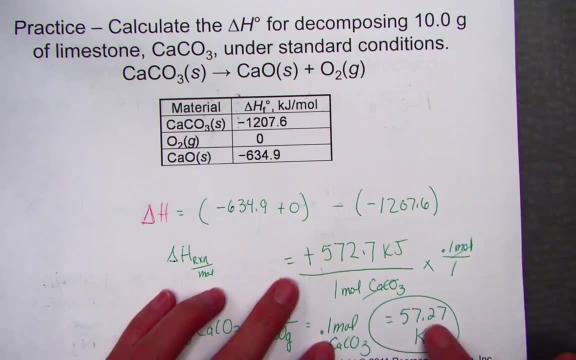 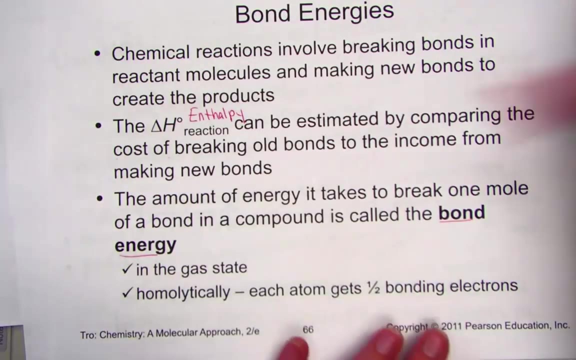 We then converted the 10 grams into a mole and decided 572.7 kilojoules for every 1 mole would be 57.27 if I had only a 0.1 mole. The last topic we'll talk about are bond energies. 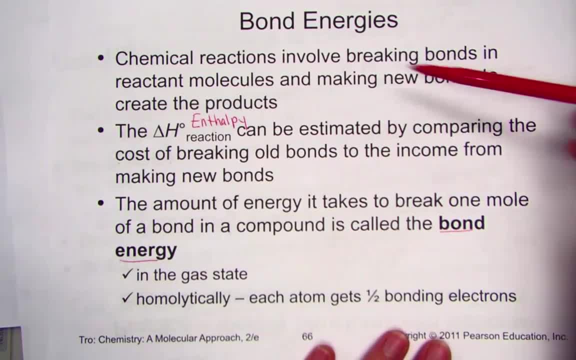 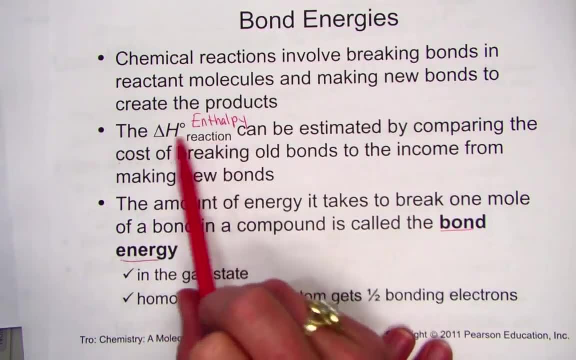 Chemical reactions involving breaking bonds and reactant molecules and forming new bonds to create the products. The enthalpy of a reaction- that's what delta H stands for is enthalpy- can be estimated by comparing the cost of breaking old bonds to the income from making new bonds. 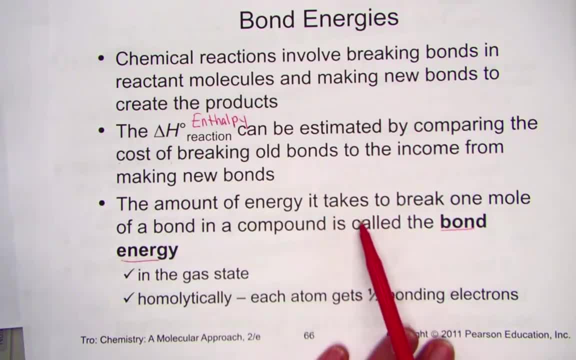 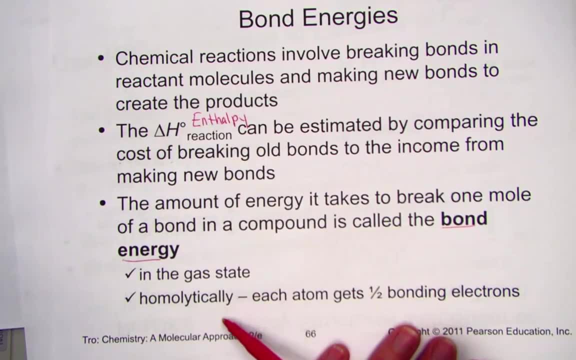 This amount of energy needed to break 1 mole of a bond is called its bond energy. Typically they are reported in the gaseous state and homolytically. just simply saying each atom gets half a mole is the cost of the bonding pairs of electrons. 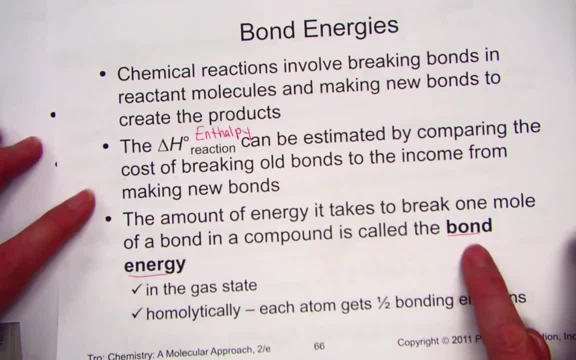 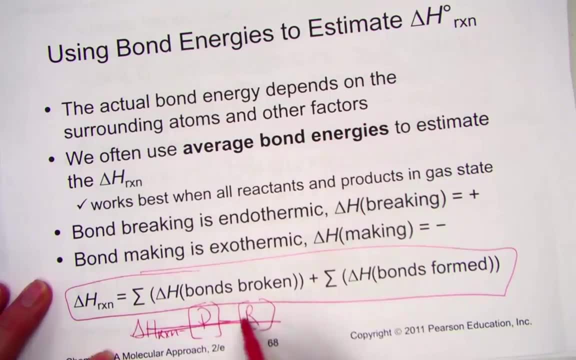 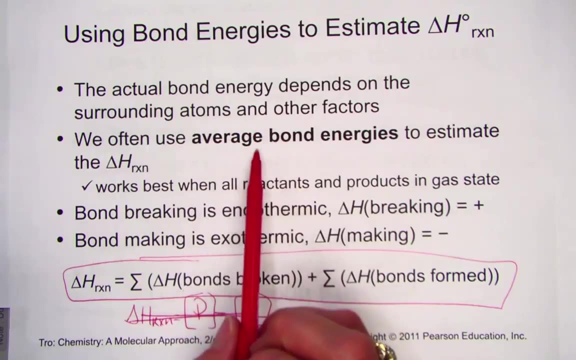 How much energy is needed to break 1 mole of a compound's bond is called its bond energy. The actual bond energy depends on the surrounding atoms and other factors, but we often use what are called average bond energies to just simply estimate the enthalpy of a reaction. 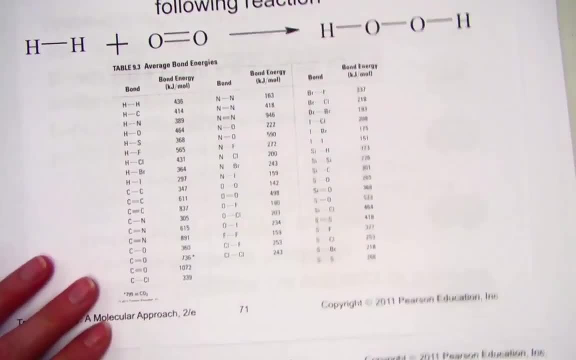 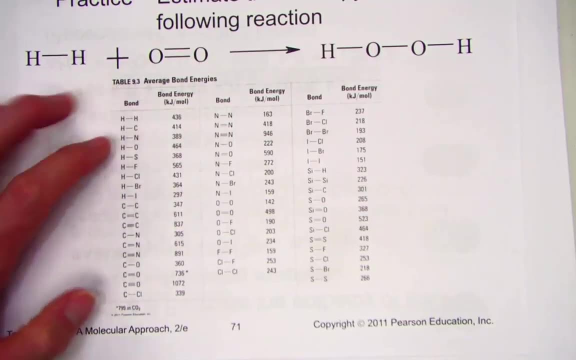 The enthalpy of a reaction really is just given to us in a chart, and here's one now. It's on slide 71.. This is a chart, then, taken from our chemistry book, table 9.3,, and just take a closer look. 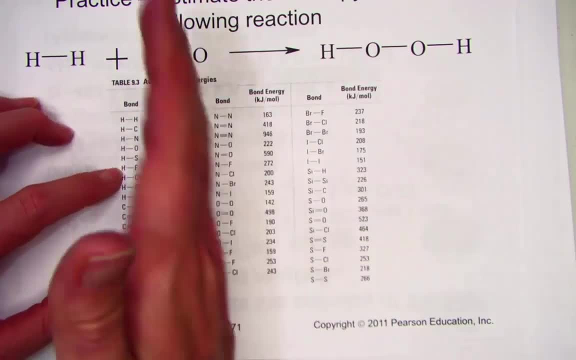 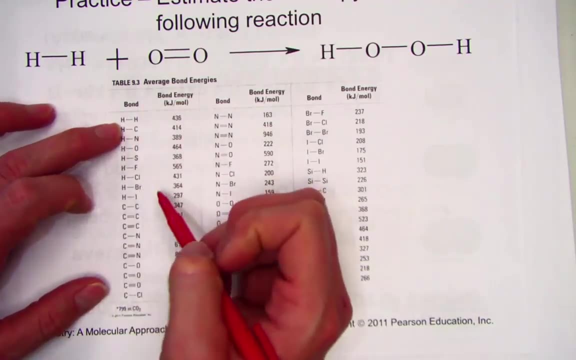 It's telling us how much energy each type of bond is required to just break them in half. If I wanted to break an H-H bond, I'd have to put in 436 kilojoules for every 1 mole of hydrogen. If I wanted to break a double bond to carbon. 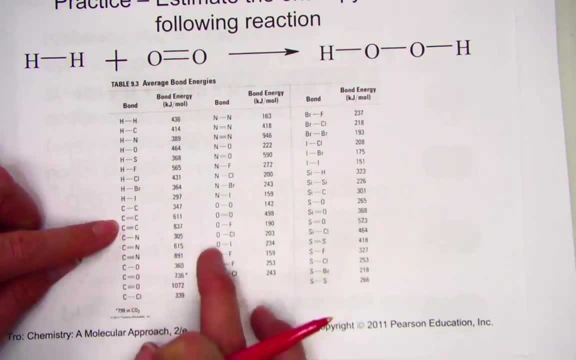 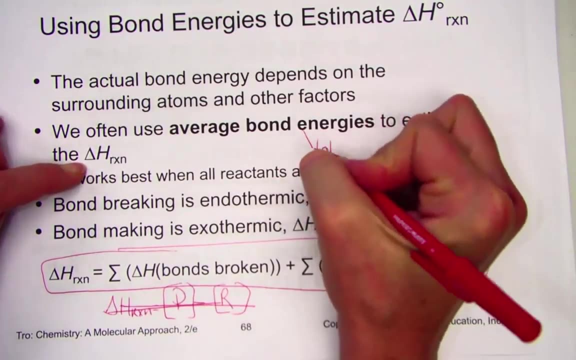 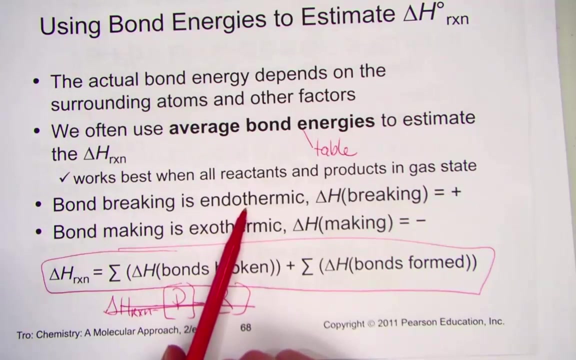 611 kilojoules of energy is required. So it's just giving us an average amount of energy needed to break a bond. So these average bond energies are reported to us in a table. We simply look them up. Bond breaking is endothermic. 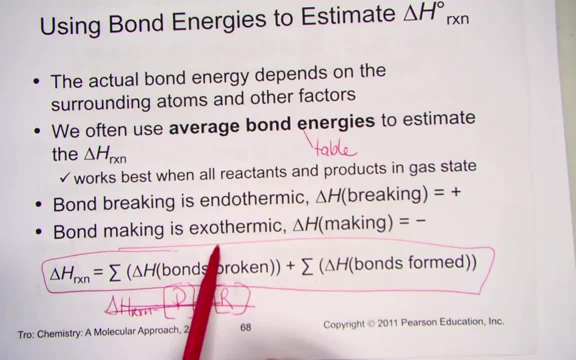 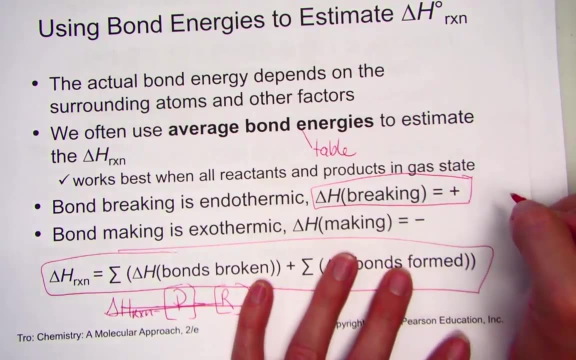 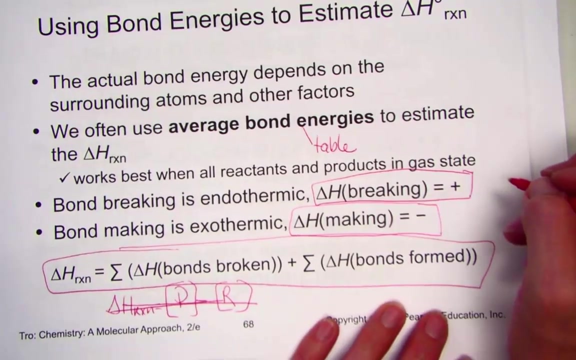 Bond making is exothermic. Breaking bonds requires energy. Making bonds releases energy. Important note: If I'm breaking bonds, the sign on delta H is positive. If I'm forming new bonds, the sign on delta H will be negative. The heat of the reaction is the sum of all the bonds broken. 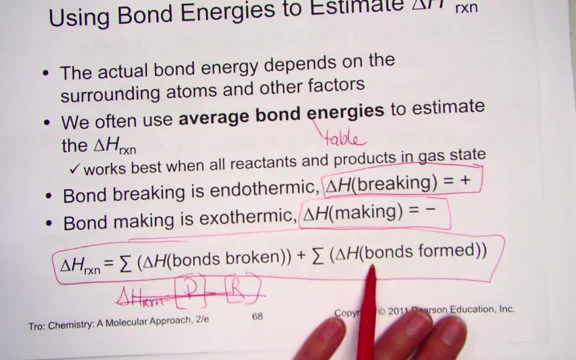 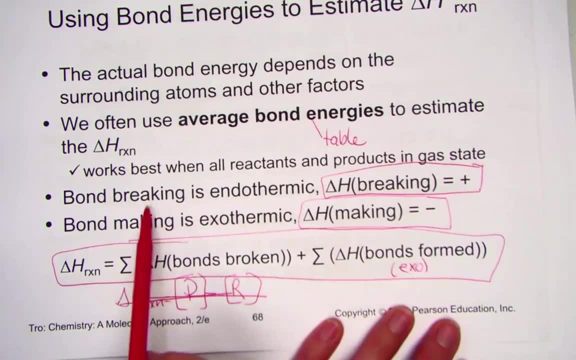 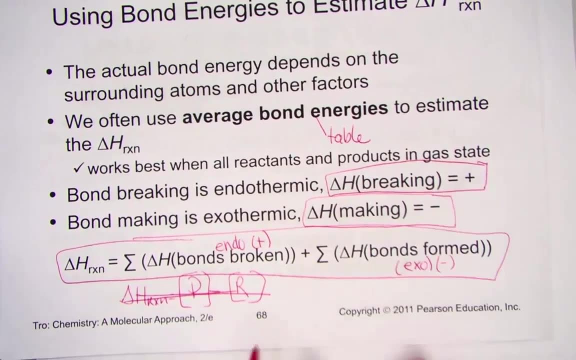 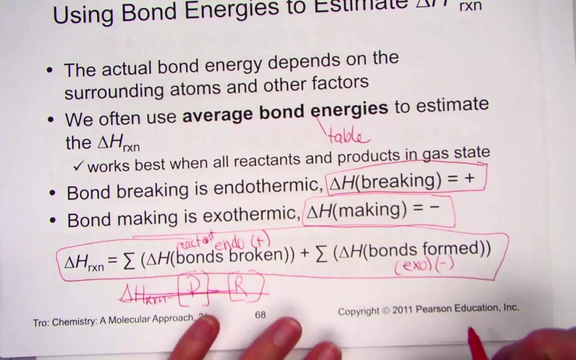 plus the sum of all the bonds formed. Forming bonds is exothermic. Bond breaking is endothermic. Keep in mind when we read the charts. we'll have to make sure if bonds are breaking on the reactant side, those are reported as positive numbers. 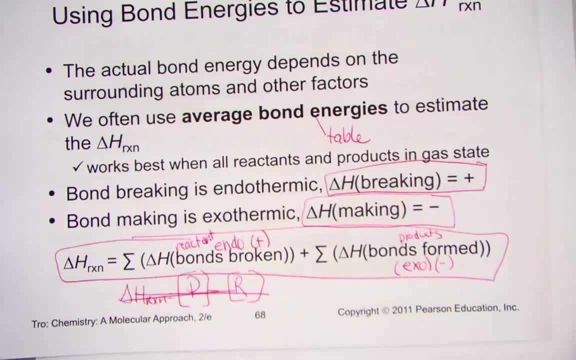 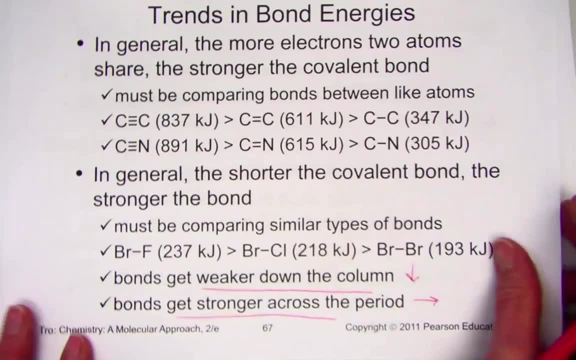 Bonds are forming on the product side. those will be reported as negative numbers. Let's take a model problem. We'll do that in a minute. We'll talk about trends in the bond energies. This is a slide. that's saying the more electrons that two atoms share. 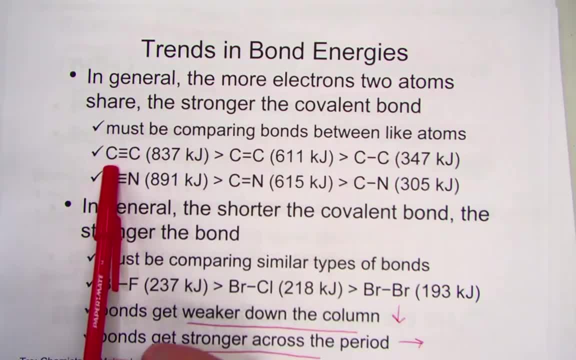 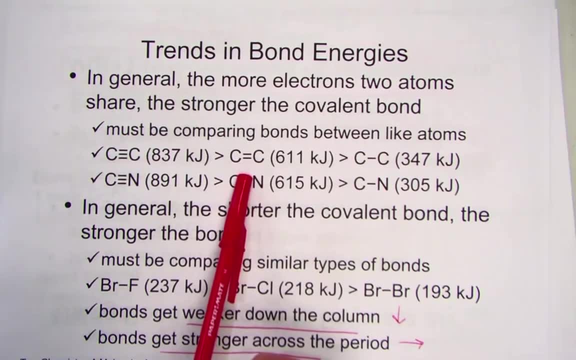 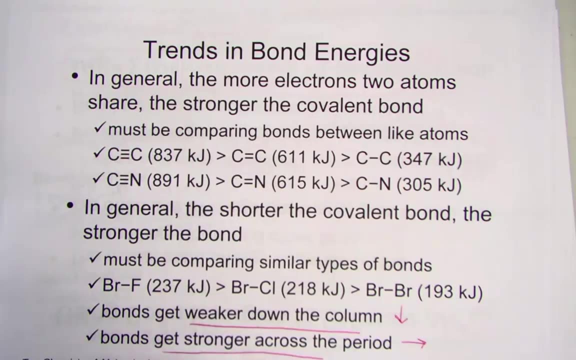 the stronger the covalent bond will be. Notice that a triple bond carbon requires much more energy to break than a double bond carbon, compared to even a single bond carbon. The more bonds between two atoms, the more energy is required to break that. 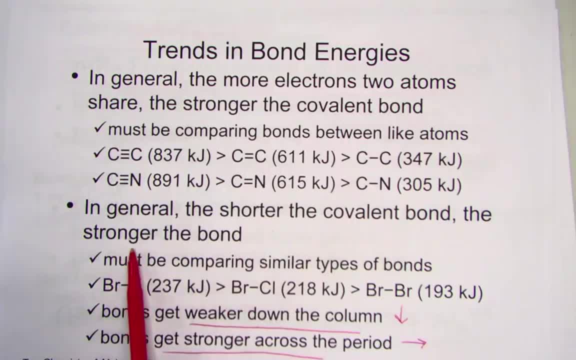 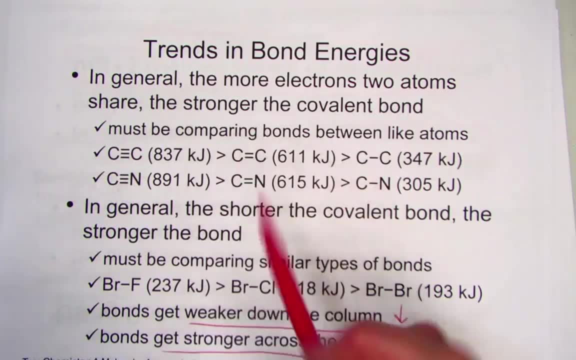 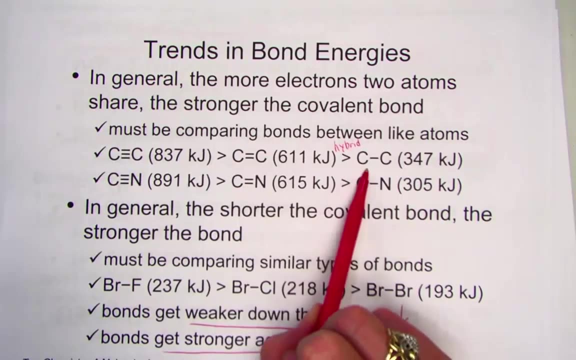 In general, the shorter the covalent bond, the stronger the bond. Triple bonds are much stronger than double, much stronger than single. And remember that resident structure- the hybrid- would lie somewhere between a single and a double bond. So the amount of energy needed to break a resident structure, 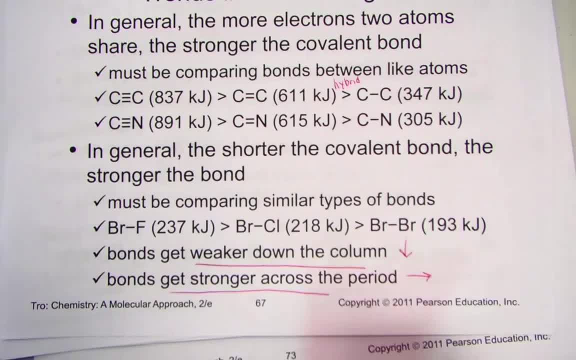 is a little different as well. In general, the shorter the bond, the stronger the bond. You can see comparatively a single bond: bromine to fluorine 237, a little less for bromine to chlorine and a little less yet for bromine to bromine. 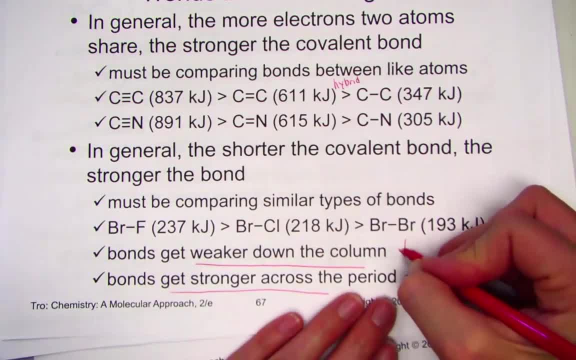 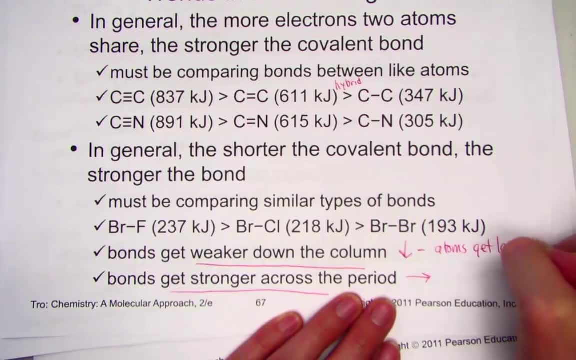 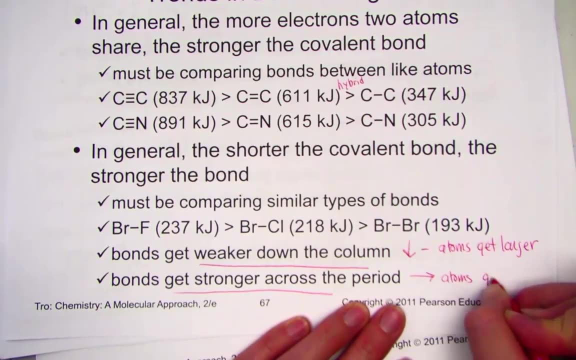 So they get weaker as you go down a column. As you go down, remember that atoms are getting larger As you go across the period. the bonds get stronger. Remember that atoms get smaller as you go across a row on the periodic table. 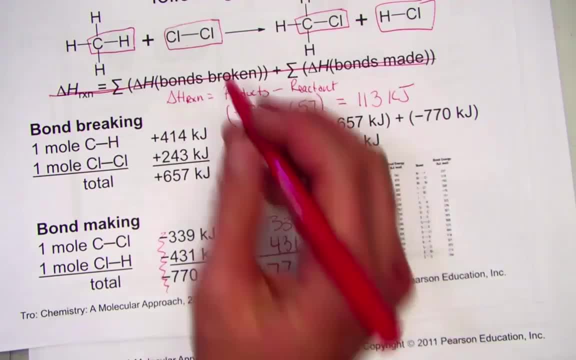 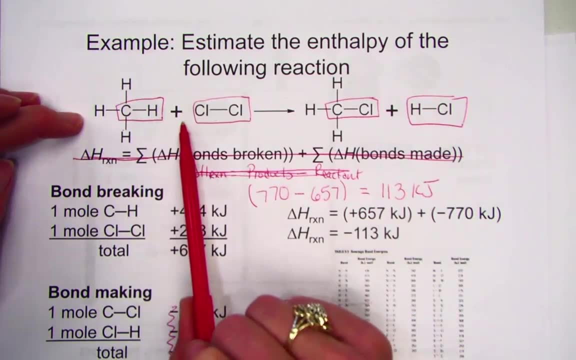 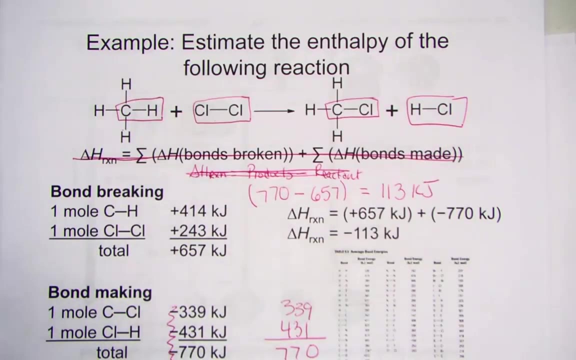 Now let's take a peek at an actual problem, And I wrote on this. I apologize. I'm going to read through my writing. We have a compound, CH4 plus Cl2, giving CH3Cl and HCl, And what's nice is that they've actually drawn for us the structural 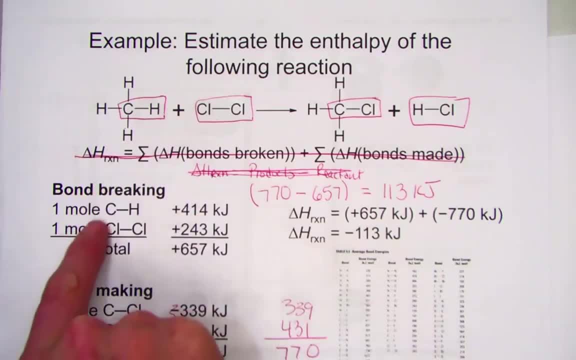 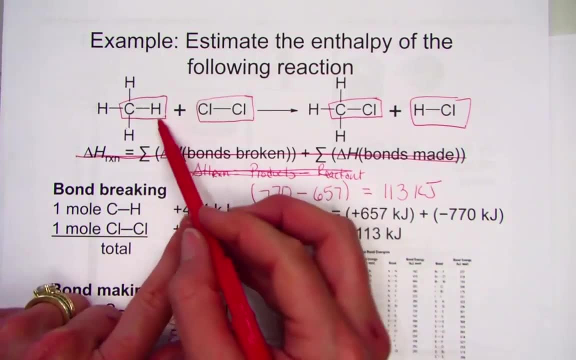 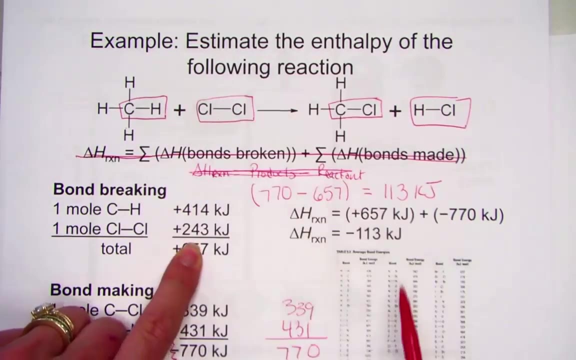 On the left side I can see that a carbon to hydrogen bond had to be broken. Carbon to hydrogen bond is 414.. That's where they're finding this value. Bonds broken end up to be endothermic positive value. I also had to break a chlorine to chlorine single bond. 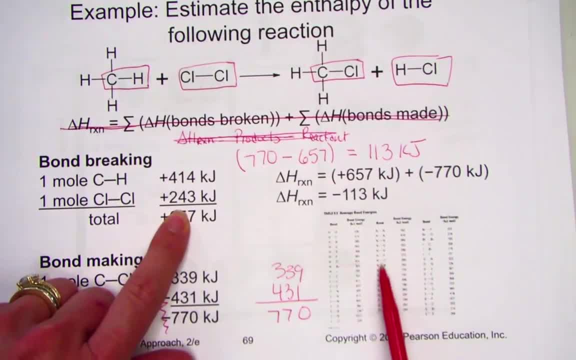 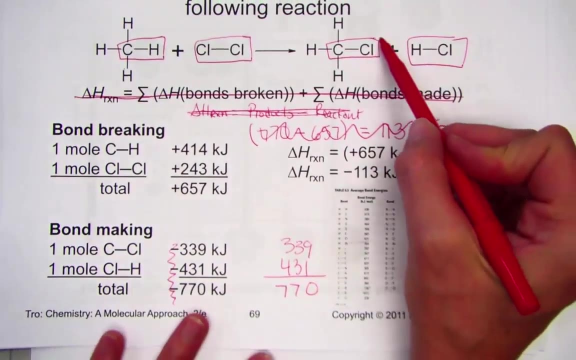 And again, using our chart, chlorine to chlorine is on the bottom of the second middle column. there 243 kilojoules. The sum of all the bonds breaking is 657.. Over on the product side, I had to create a carbon-chlorine bond. 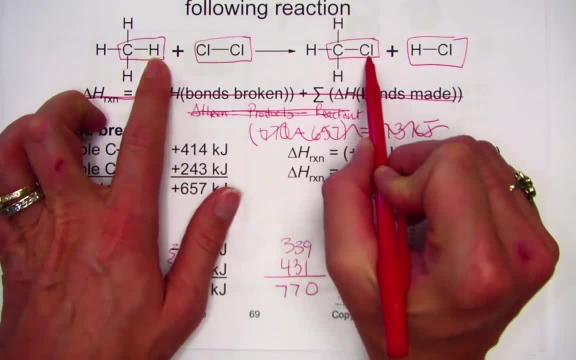 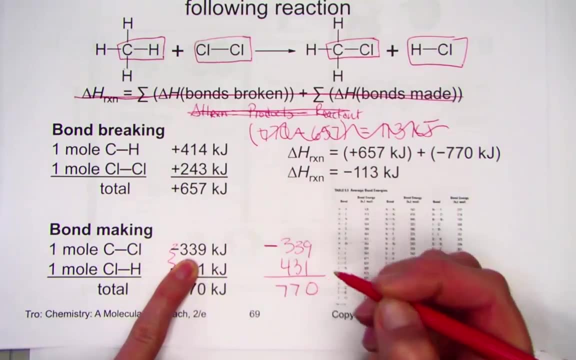 It was a carbon to hydrogen On the product side. now it's carbon to chlorine. Carbon to chlorine, 339.. Notice, the negative sign is being placed there because now the bonds are making and that's exothermic negative value. 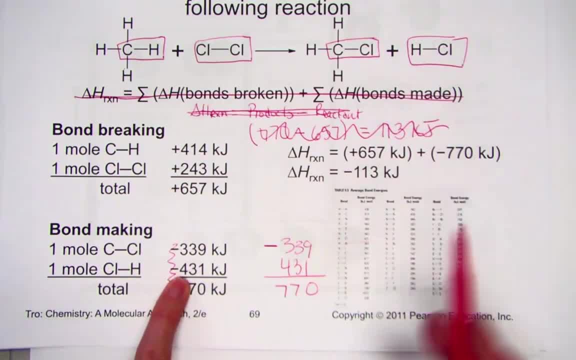 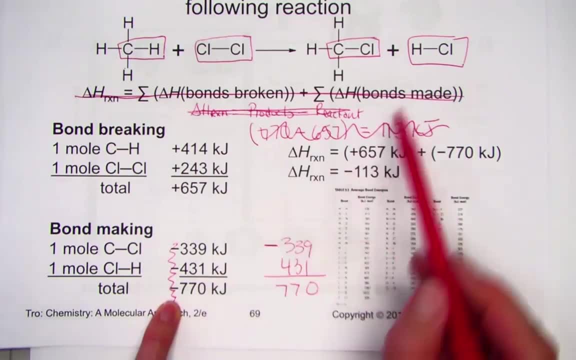 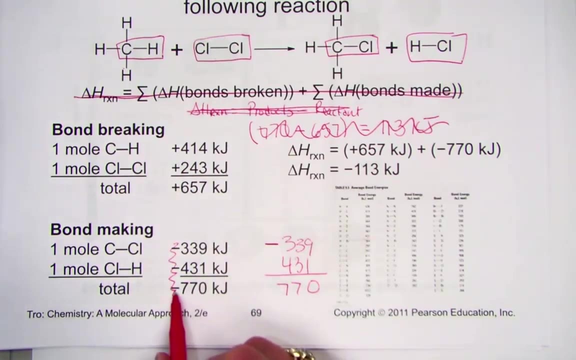 We made an HCl. HCl again- I just look up- Hydrogen to chlorine is 431.. Report that as negative because it is forming a bond. Those are exothermic, The total energy then, and an exothermic value 770 for the product side. 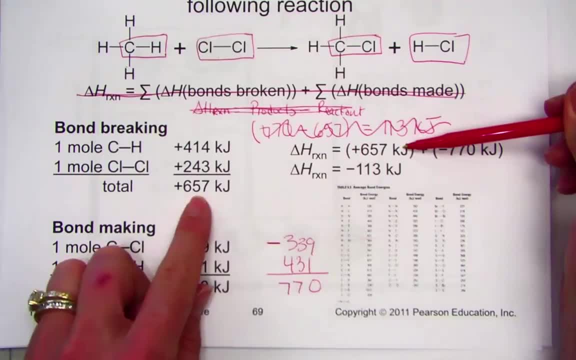 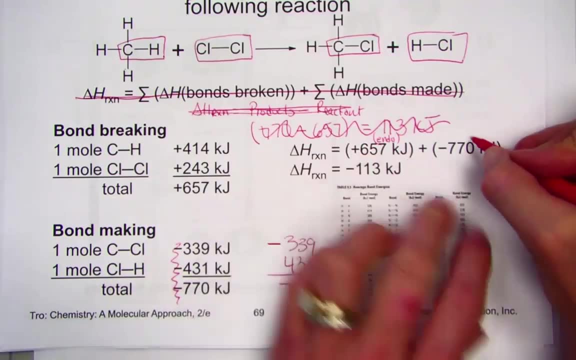 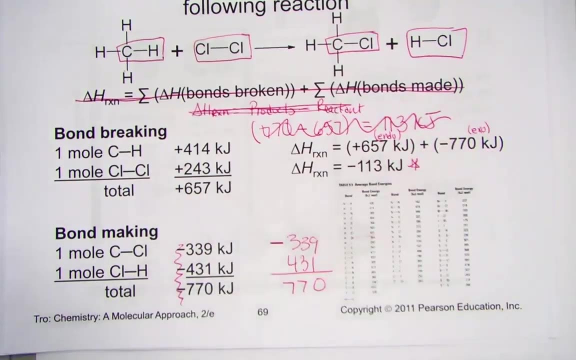 The sum of all the bonds broken: 657.. Notice: bonds broken. Endothermic value for the reactants Plus the exothermic sum for forming new bonds gives us a net heat of reaction of negative 113 kilojoules. This is an exothermic process overall. 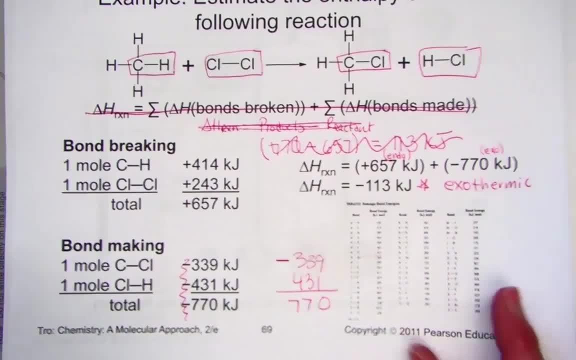 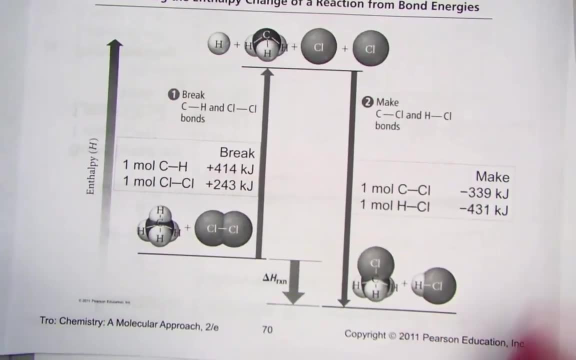 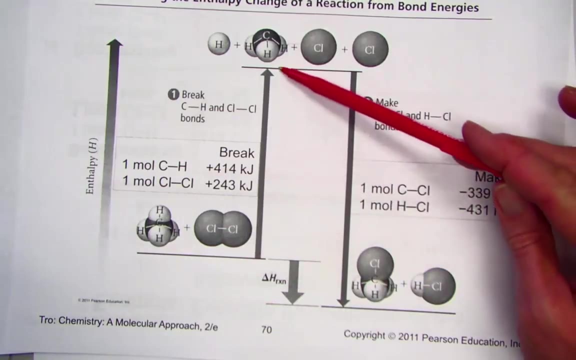 The energy was released during the course of this reaction. Estimating the enthalpy change of a reaction from bond energies. this is just a picture of what we went through. Methane plus chlorine: To break the bonds required energy. We input energy, so it went up positive value. 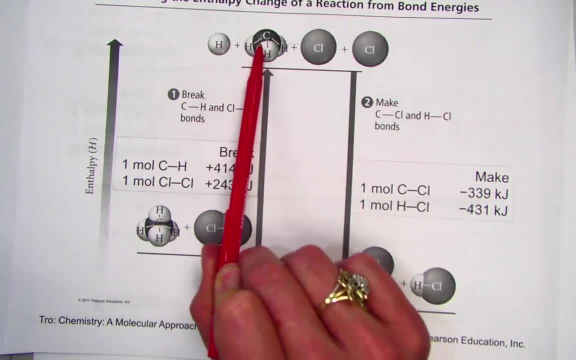 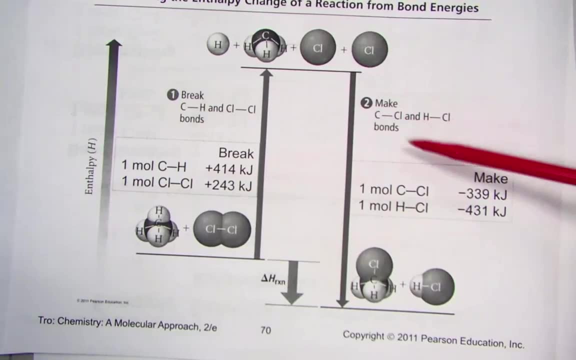 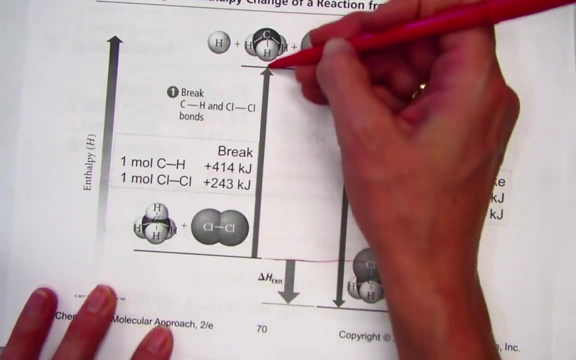 So now we've broken a bond. I see hydrogen has been broken and the two chlorines have been broken apart. We then make bonds. We form a carbon to chlorine and a hydrogen to chlorine. That is an exothermic process. The overall change from the amount of energy input. 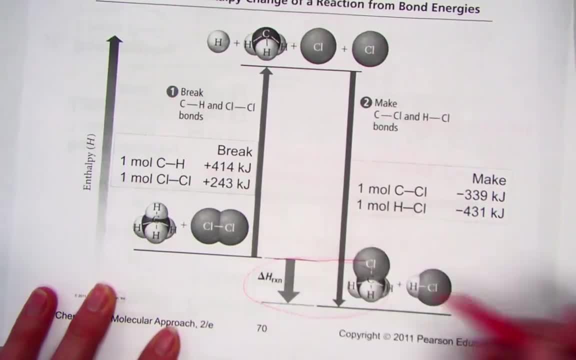 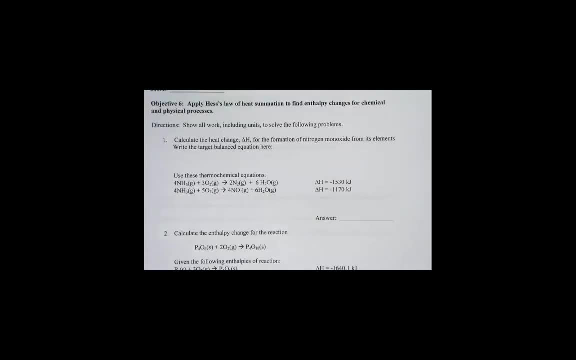 and the amount of energy let go ended up to be a net negative Overall process was exothermic. Our first question says: calculate the heat change, that's delta H, for the formation of nitrogen monoxide from its elements. We are being asked to turn those words into a balanced equation. 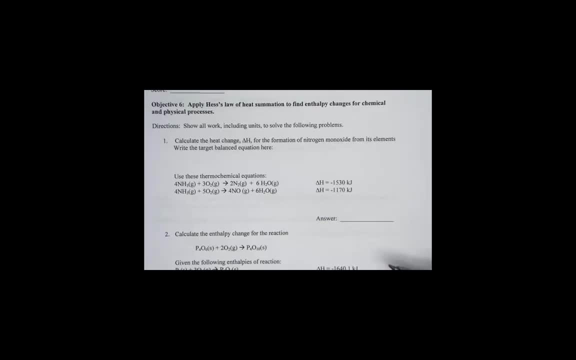 and that balanced equation then becomes our target equation. We are forming nitrogen monoxide To form. we need to point at it, creating a product of nitrogen monoxide, Listening to those prefixes and letting that guide our NO for nitrogen monoxide, The elements that it's built from. 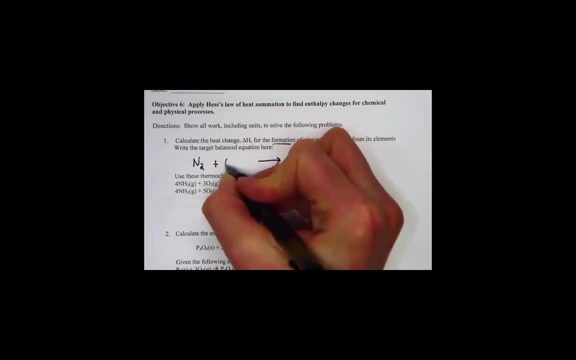 both belong to the Lucky 7 diatomic club. nitrogen and oxygen will be written in molecular form: N2 plus O2.. And, of course, to balance our equation we'll need to have two units of NO, The target equation we are being asked to build. 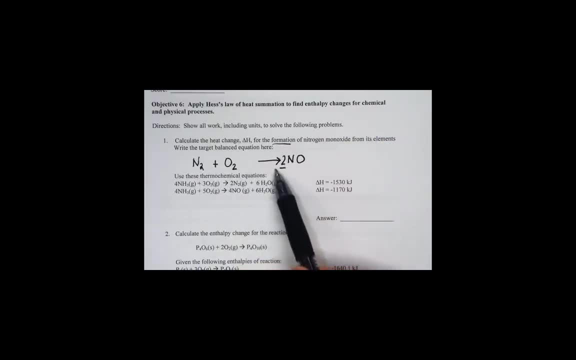 will be N2 plus O2, forming two units of NO. We'd like to know the heat change for this equation. What is the value of delta H? What we do know are the following elementary reactions. In our first equation I'm reading four units of NH3. 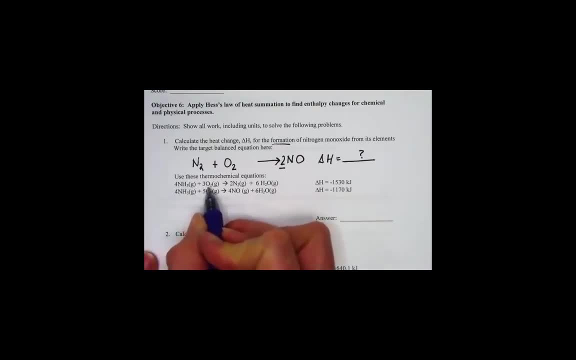 react with three units of O2 to form two units of N2 plus six units of water. Its delta H is given as negative 1530 KJs. Our second elementary reaction: four NH3s plus five O2s yield four NO and six H2Os. 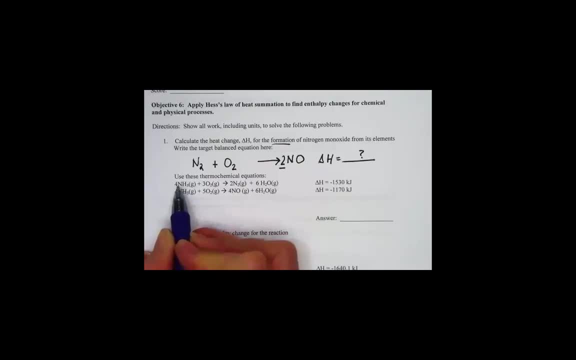 We are being asked to use these two elementary reactions, equation one and equation two, so that somehow, when we add them together, simplifying what we can from the left and the right, that it indeed forms the target equation That we just wrote in that combination pattern. 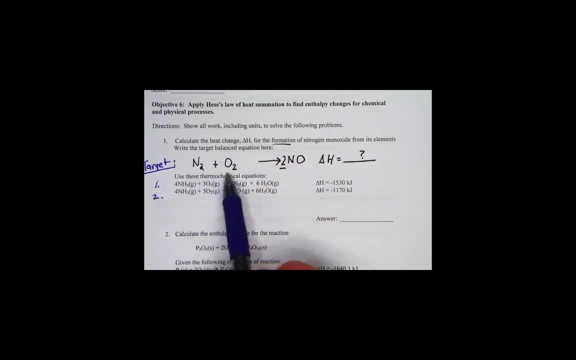 The target is to build one unit of Ns plus one unit of Os to produce two units of NO. For no particular reason than it's written first, I start using my elementary reactions to find the first reactant in the target. Where do we see N2 written in our building blocks? 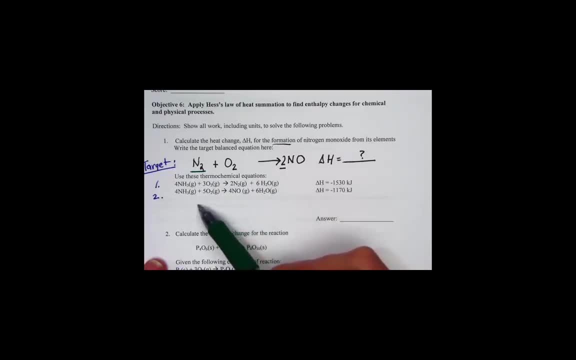 in our elementary equations. Well, I notice in the first elementary reaction I'm seeing it written and it's in a unique spot. That's very helpful in determining what to do with that first elementary reaction. I notice that N2 is on the wrong side of the arrow. 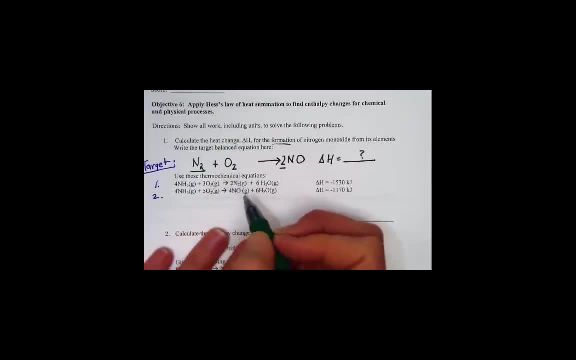 as compared to my target, And I'm noticing that it's twice as big as I'd like it to be. I have a hunch that I'm going to flip the direction and I'll need to cut it in half Again. my reason: 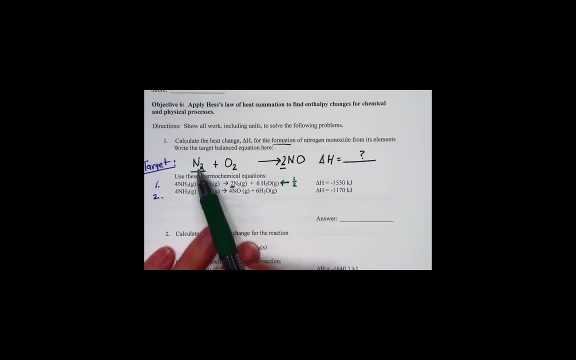 I'd like to have one unit of N2 on the reactant side, but where I'm seeing it is on the product side and it's twice as big as I'd like it. If I flip it and cut it in half, I might have just what I need. 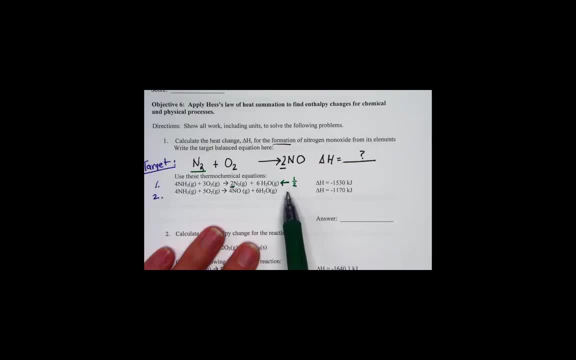 Again, I'm not showing work yet. I'm just simply thinking out loud, brainstorming a strategy. The next reactant is the O2 in the target equation. What I'm noticing is the O2 appears in both elementary reactions. It's not very helpful if it's appearing in both. 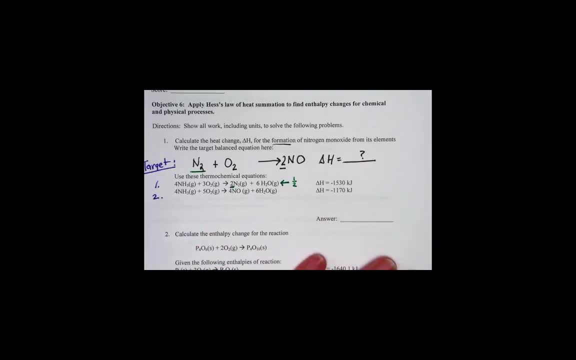 I'm not going to gain insight into what to do with that second elementary reaction. I'm going to choose to ignore that for right now. I'm not finding it in a unique place. More interesting is the placement of our product. NO. I'd like to make two units of NO in our target equation. 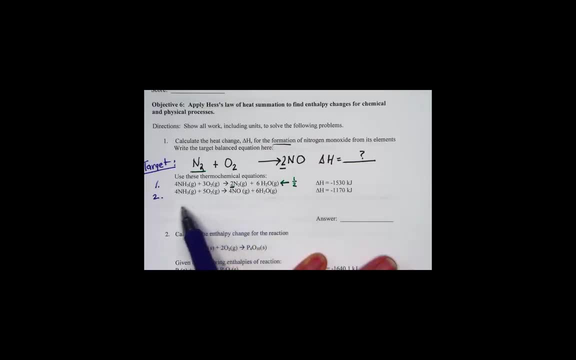 Where might I find NO in the elementary reactions? Well, I'm finding it in the second equation, right here, as the listed of the first product. I like the side that it's placed on. It's on the product side as I desire it to be. 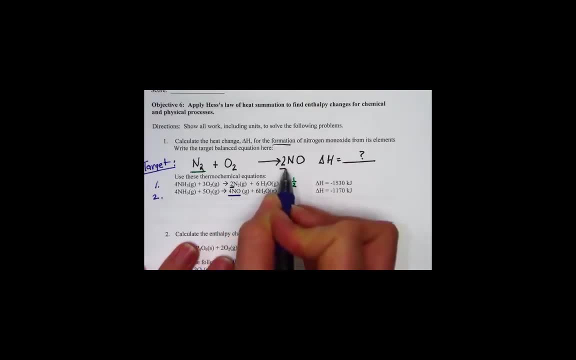 But four units of NO is twice as large as I'd need in my target equation. I only need to produce two units and I have four in the target. Again, thinking out loud, I'm going to divide this by two or cut it in half. 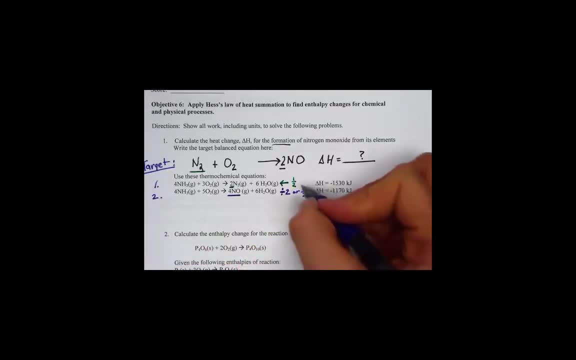 whatever you think in terms of being easiest for you- Cutting in half, dividing by two- we'll need to do both of that: Flip the first, cut it in half and then simply cut the second one in half. Let's see what that gives us. 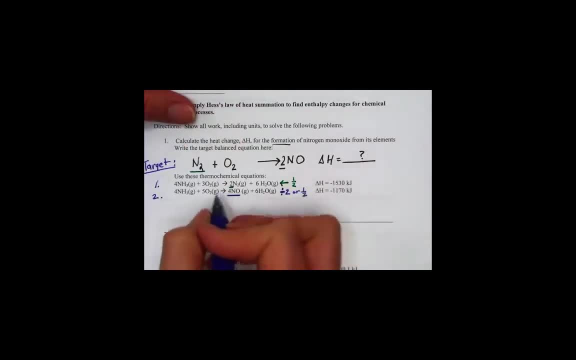 Let's rewrite the strategy so far. We decided in our first elementary reaction, rewriting it in the opposite direction, taking only half the amounts. So the original products now become the reactant. We had written two units of N2.. Let's cut that in half. 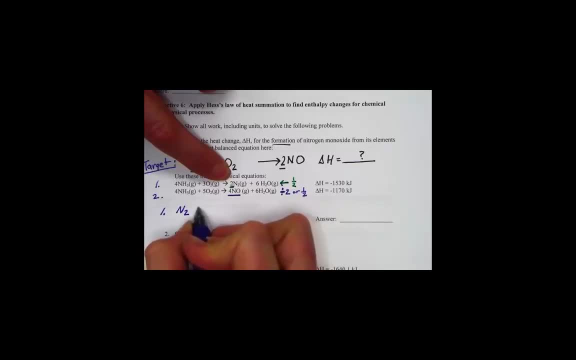 We'd now be left with one unit of N2 plus plus. We started with six units of water. Cutting that in half gives us three units of H2O. Then we see the yield sign On the original reactants, now writing M on the product side. 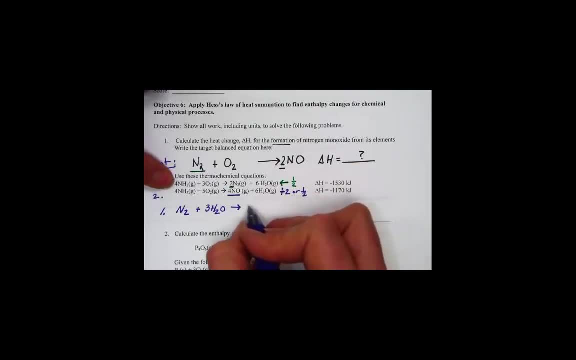 we started with four units of ammonia. Cutting it in half, we're down to two units of ammonia NH3.. Up here we started with three units of oxygen. If we cut that in half, let's write that as three halves of O2.. 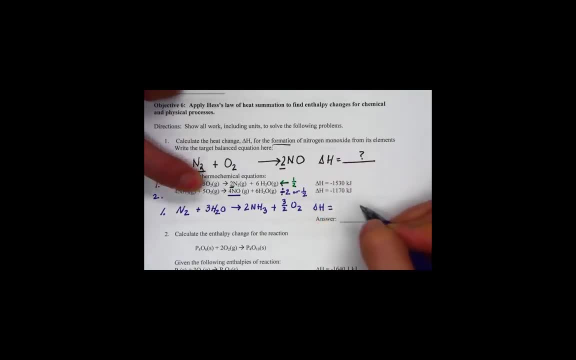 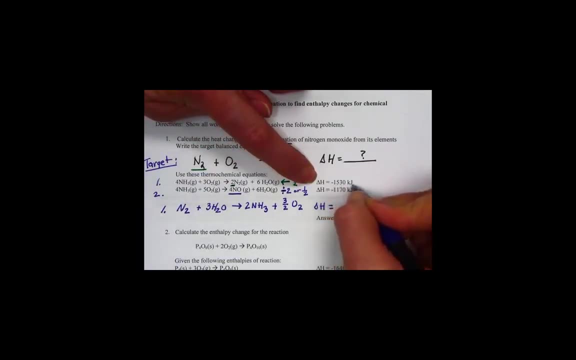 The delta H for this new equation will be found by looking at the first value given, negative 1530.. Since we flipped to the direction we need to make it positive and we also cut it in half. We need half the value. 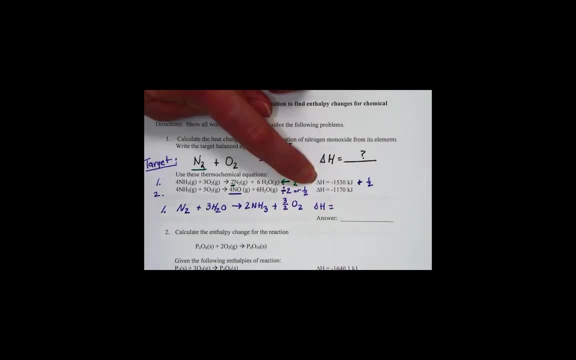 Let me hit on the calculator: 1530 divided by two, and I find that to be 765.. Half the amount and the opposite sign give us the new delta H for our elementary reaction. The second equation: we decided to leave the direction alone. 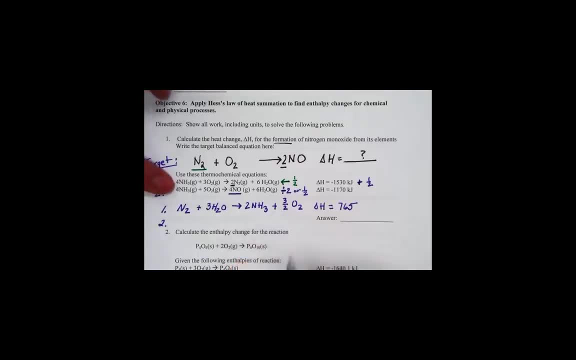 but to cut it in half. We started with four units of ammonia. Cutting that in half leaves us with two units of ammonia. The next reactant written is five units of O2.. When we cut that in half we would write that five halves of O2.. 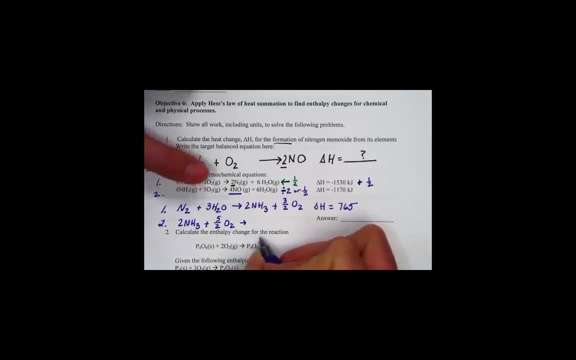 Leave it in the fraction form. The next product listed is four units of NO, but cutting that in half leaves us a net of two units of NO. And finally, six units of water: cut in half gives us three units of H2O. 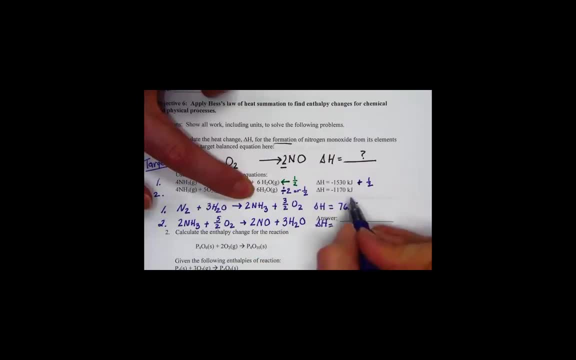 The delta H for this new equation would simply be half the amount of the original value. Let me hit that: 1170 divided by two, It's 585.. Still remaining negative, but half the amount. Hess's Law of Summation. 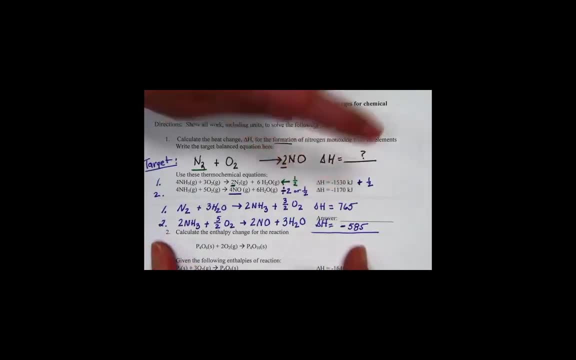 If we add our two equations together, simplifying what we can. let's prove to ourselves: we indeed have made the target equation. What could cancel, I'm noticing? in the first reaction I made two units of NH3. And in the second equation, 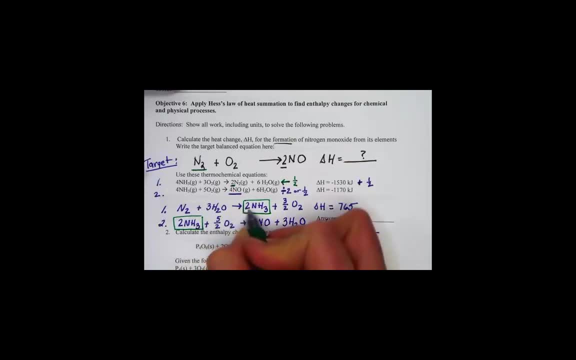 two units of NH3 are being used. A product on one side cancels the reactant on the other. The ammonias are gone. I also notice in the first equation I have three waters written on the reactant side And in the second equation. 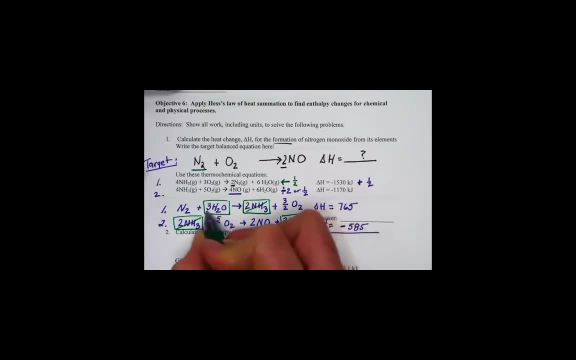 I have three waters written on the product side. Three H2O's on the left will cancel with three H2O's on the right. in the next equation The waters are gone. I'm also noticing O2 appearing on both sides On the first equation. 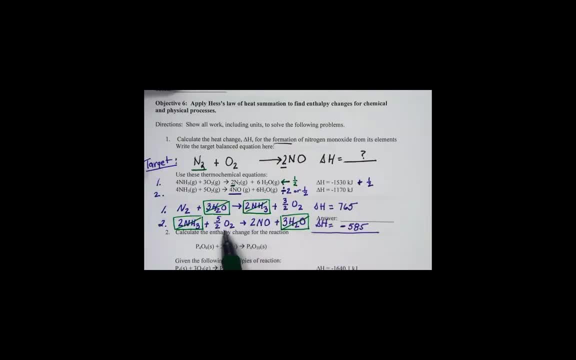 we have the amount of three halves. In the second equation we have the amount of five halves. That can be simplified: Five minus three is two. Two halves is equivalent to writing one unit of O2.. If I take out the product side, 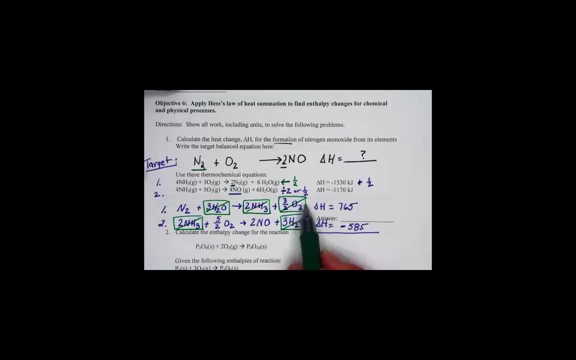 in the first equation three halves O2, and I simplify with the five halves that was written. five minus three would give me two halves. Two halves is equivalent as one. And look what we've done. We have taken N2 plus one unit of O2. 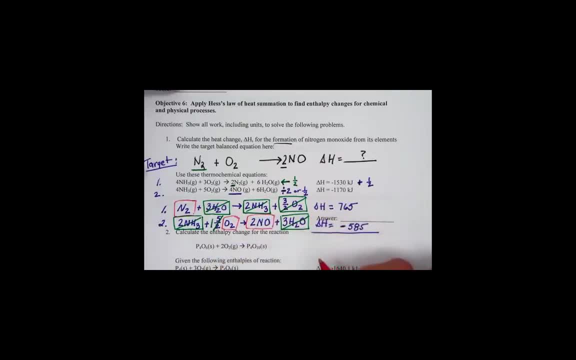 to form two units of NO, And that, indeed, is our target equation. The only thing left to do is to add the new values of the delta H's Positive 765 plus a negative 585 gives me a total value of positive 180 kilojoules. 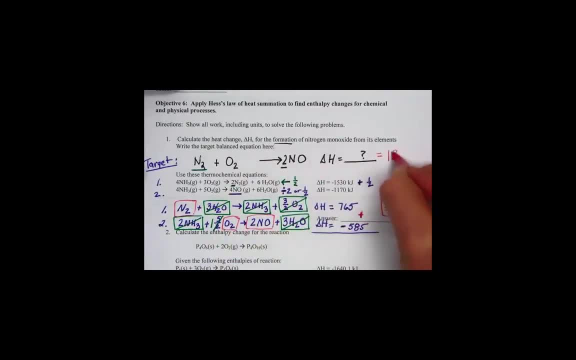 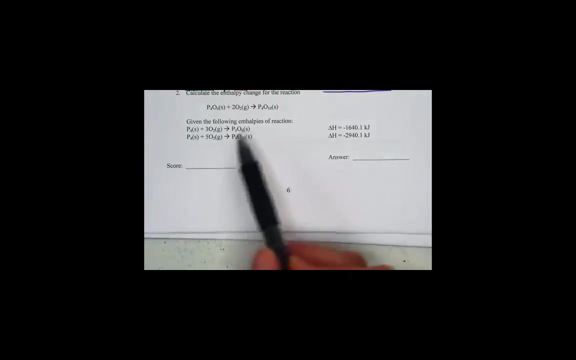 The value for our target equation. we were solving for 180 KJs, an endothermic value. Let's look next at practice test A, the second question. with Hess's law, Our target equation has us looking at P4O6 as a solid. 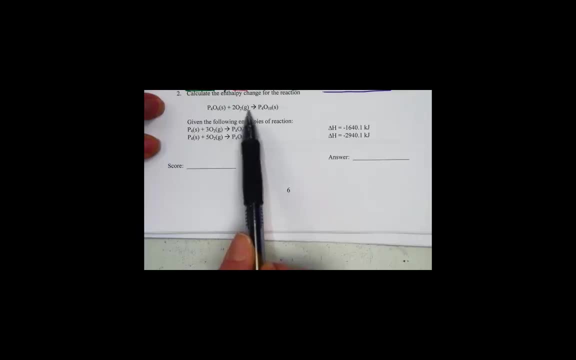 plus two units of oxygen O2, forming P4O10 in a solid phase. This is what we would label as our target equation. We have two elementary reactions to build our target Elementary reaction. one has P4 as a solid plus three units of O2. 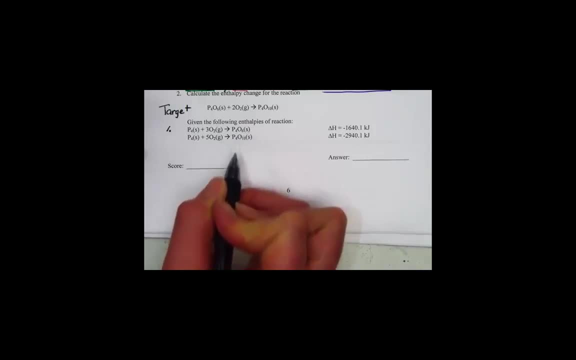 as a gas forming P4O6 solid, And that second elementary reaction, P4 solid plus five O2s, yields P4O10 solid. For no other reason than it's written first in my target equation, I generally start looking to find my first reactant. 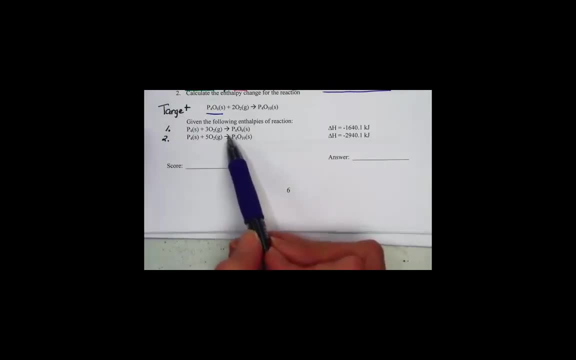 Where might I look to find the first reactant, P4O6?? And again, just start skimming through the elementary reactions until you locate it. Here I have it at the first equation, at the end listed as a product. What I like about it. 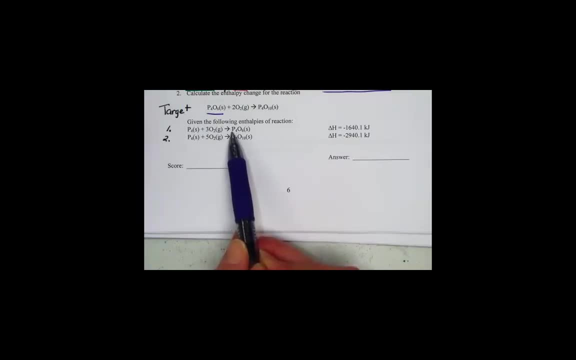 is that it has the correct number of units. There is a one which matches the target value. We need a one, But what I don't like about it is the side of the arrow. it's on In my target. it appears as a reactant. 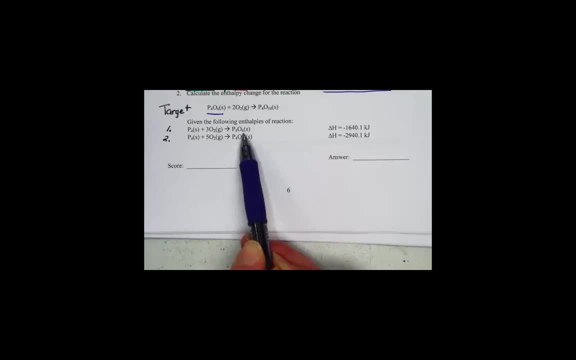 But in the elementary reactions it's appearing as a product. Thinking out loud of a strategy, I think I need to flip the direction of the first reaction. I notice the second reactant is oxygen O2.. I'd like to end up with. 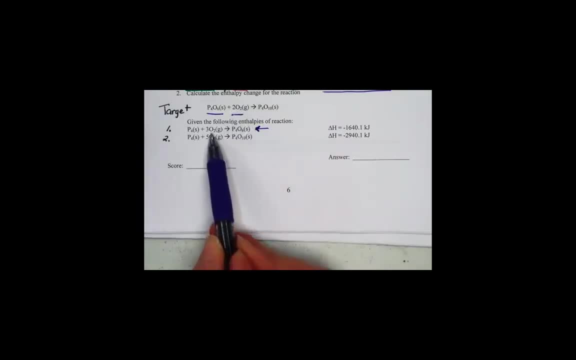 two units of O2.. But the O2 appears in both elementary reactions. It's not in one unique place. The O2 is not something I would choose to make a decision on what to do with these elementary reactions. Let's instead focus on 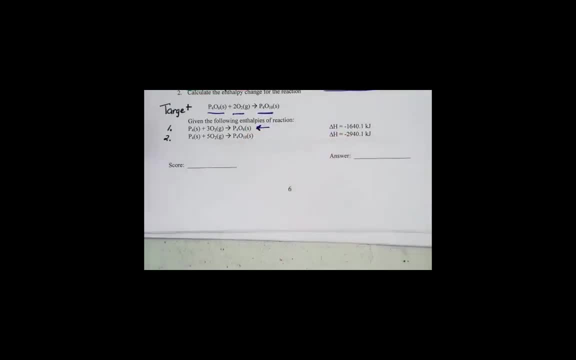 the product P4O10.. P4O10 appears as a product in the second equation. Again, I'm going to ignore the O2 because it's not in a unique place. The P4O10 is unique. It's uniquely placed as a product. 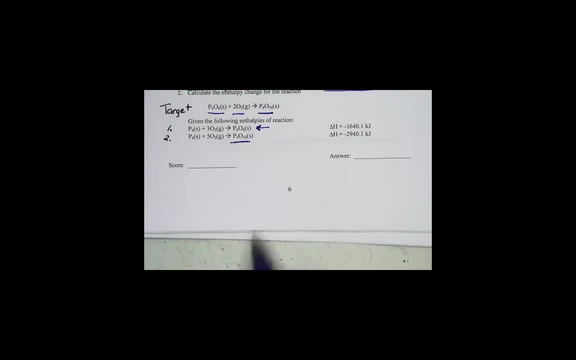 in the second elementary reaction. Here's what I like about that. I have the correct number of units In my target. I need to produce one unit of P4O10.. And the target equation has just one. so does the elementary reaction. 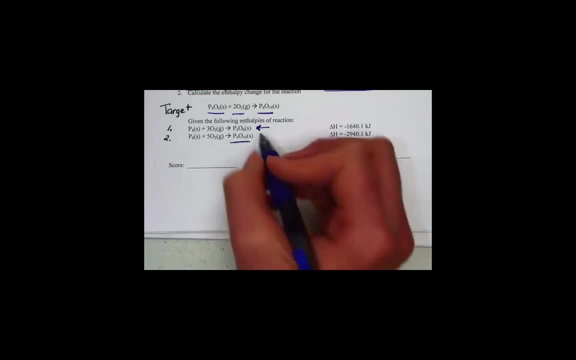 And it's on the correct set of the arrow That tells me I should leave this alone. So far, I've just been sharing a strategy. Let's indeed prove to ourselves that, by flipping the first, leaving the second one alone, we have indeed built our target equation. 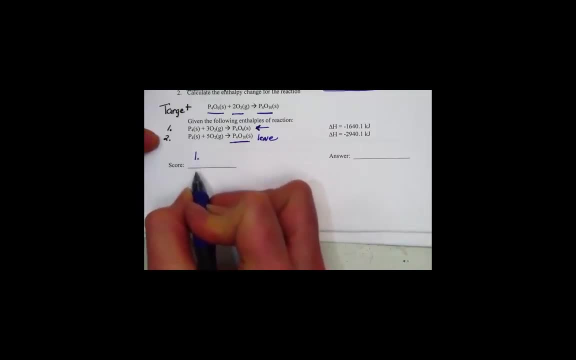 Let's rewrite elementary reaction one, but flip its direction. The original product, P4O6, now becomes the reactant, And the original reactants now are on the product side. P4O6 points at P4 plus 302.. 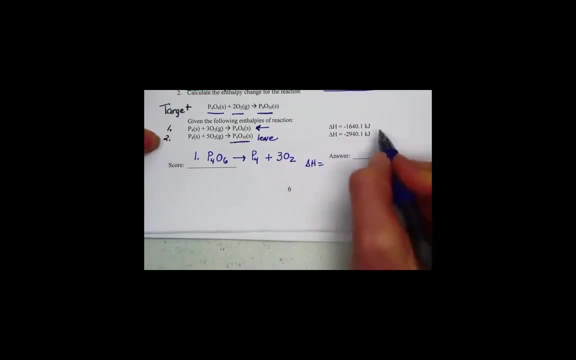 The delta H for this equation. simply flipping the sign, it now reports a positive 1640.1 kJs. We decided to leave the second elementary reaction just as it appears. I'll simply rewrite: P4 plus 502s make P4O10.. 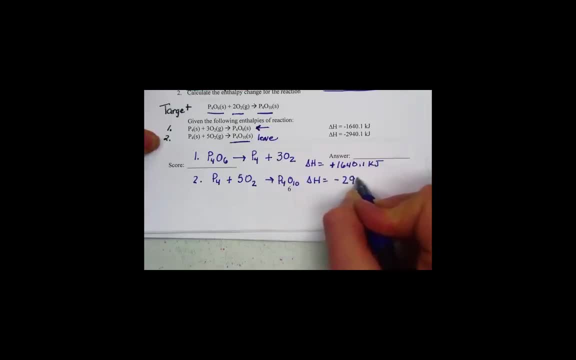 The delta H remains the same value: negative 290, negative 2940.1 kJs. If we indeed add these together, simplify what we can. I notice that P4s are on opposite sides of the arrow. a product in equation one. 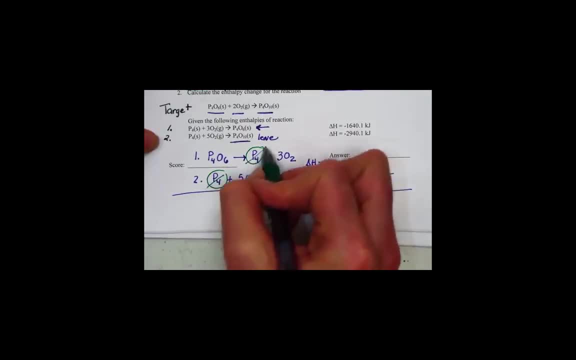 a reactant in equation two. They will cancel one another. I also notice that on the right side of our first equation I have three oxygens and on the left side of the equation, in the second, I have five. If I simplify, 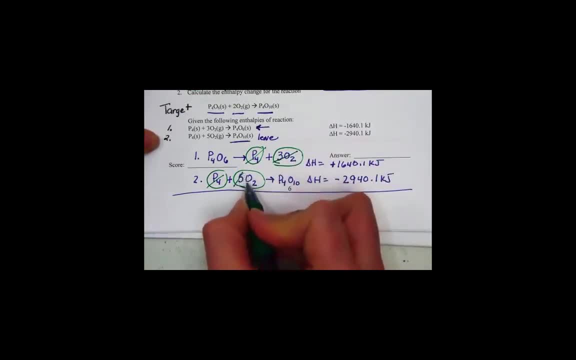 I can get rid of the 302s, leaving me a remainder of two. Five minus three simplifies to two units of O2.. And indeed we have built P4O6, left over from that first equation and two units of O2,. 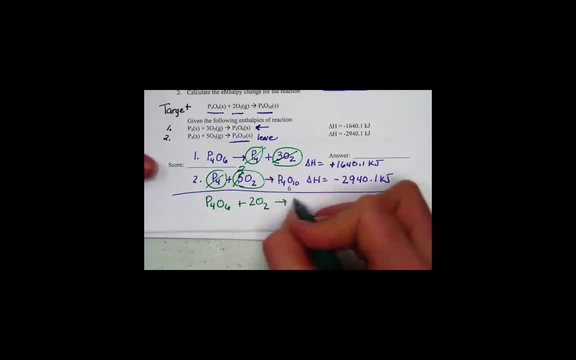 the remainder of our second equation forming the desired product of P4O10.. When I add together elementary reaction one, its heat, with the elementary reaction two of its heat, we'll find our final answer. So let's hit positive 1640.1. 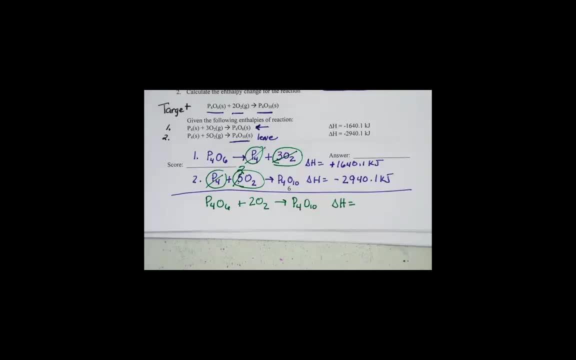 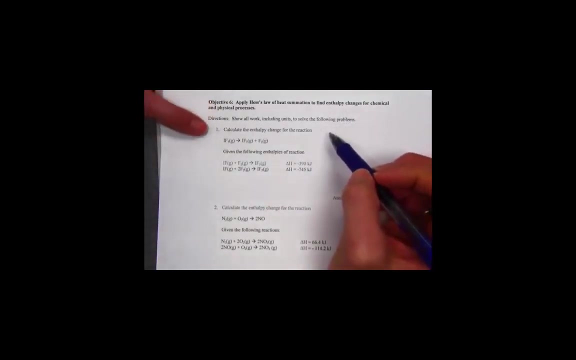 plus a negative 2940.1.. I get a value of negative 1300 kJs, an exothermic value With Hess's law of heat summation: we are being asked to find the enthalpy change of what we call our target equation. 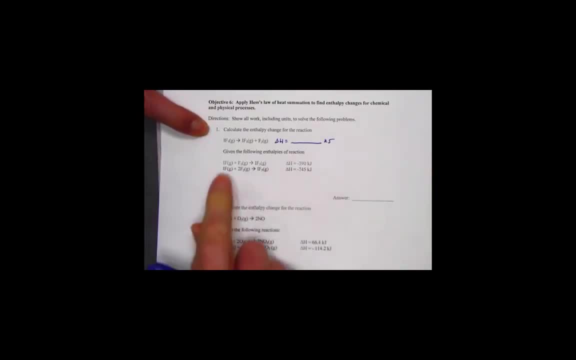 given the elementary reactions to build from. What we're trying to do is somehow add the two equations below so that they create the target equation, And once we do that, we simply add their values of delta H to find the target. Whatever we do to the elementary reaction, 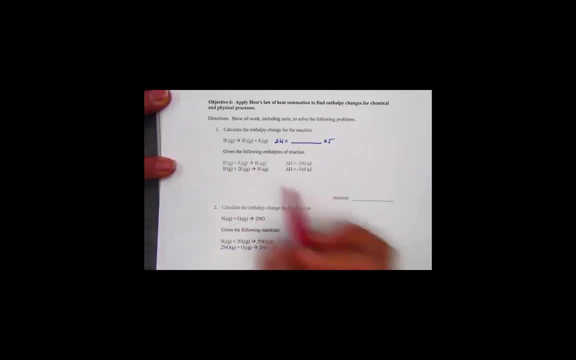 we do the same thing to the target IF plus F2. given IF3, its value of delta H, provided IF plus two fluorines give IF5, its delta H is provided We have two building block equations to create the target: IF5 yields IF3 plus F2.. 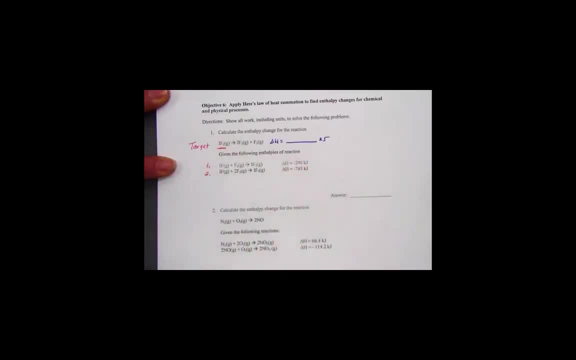 I simply turn my attention to the first reactant in our target equation and start skimming through where I find the IF5 in the targets. I'm noticing that IF5 is given to me in the second equation and it's a unique place. 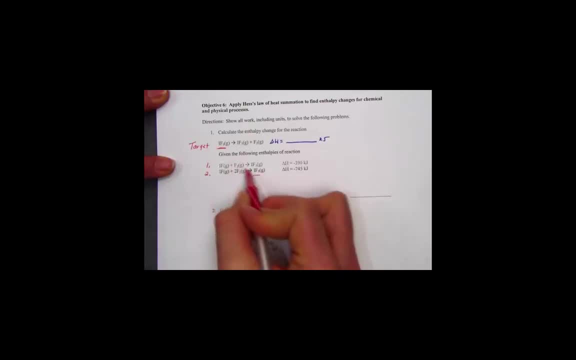 There is only one location of IF5.. What I'm noticing is I have the right number, but it's on the wrong side of the arrow. I'm predicting that we'll need to flip or reverse the reaction for number two, And when I do that? 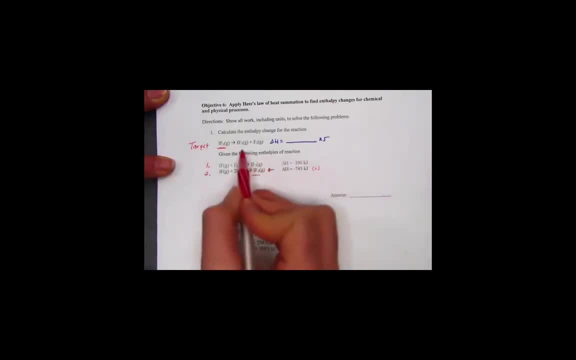 I know I need to change the sign. The second ingredient listed up here in the target is the IF3.. IF3 appears uniquely in that first target equation. I like the number I have and I like the side of the arrow I'm on. 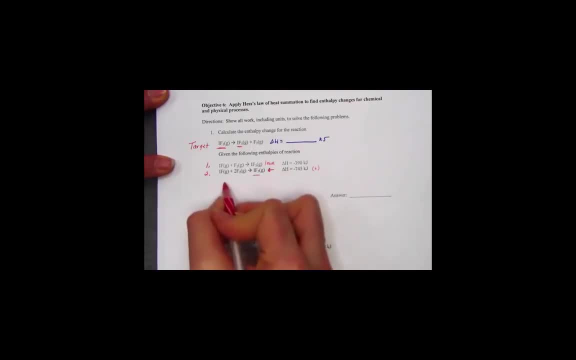 I bet we just leave that alone. Let's rewrite, finally, showing the work we would be required, Leaving the first one alone. we'll just simply rewrite it. IF plus F2 yields IF3.. Delta H has stayed the same at negative 390 kilojoules.